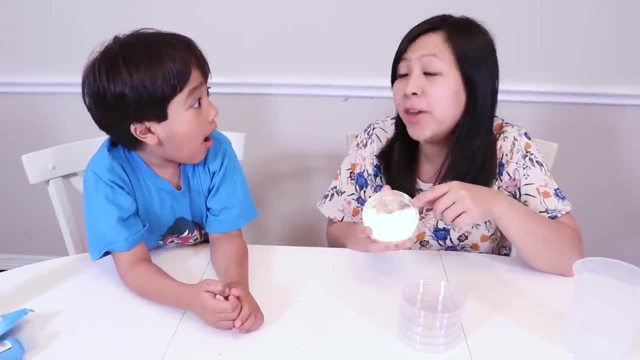 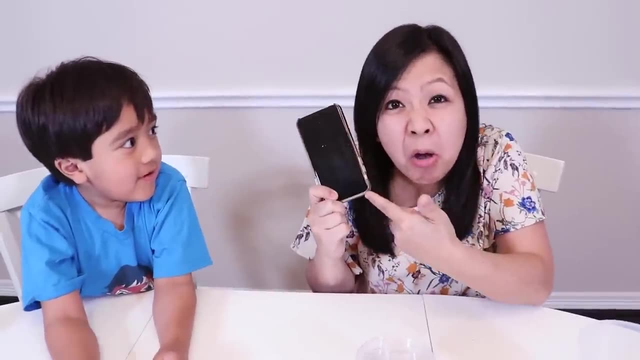 And it's going to take a whole week. So there's bacteria everywhere. There's bacteria right now on this table. There's bacteria probably on my phone Bacteria probably on us. That's true. yeah, There's probably even bacteria on my shoe. 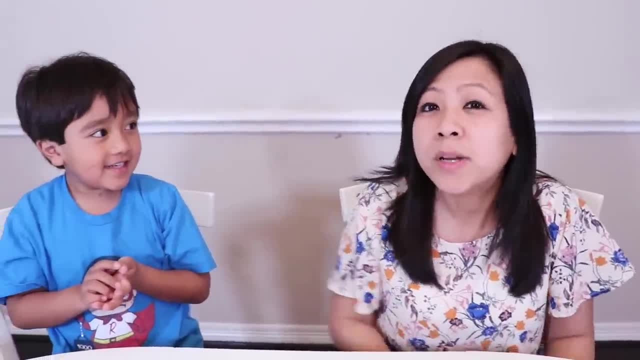 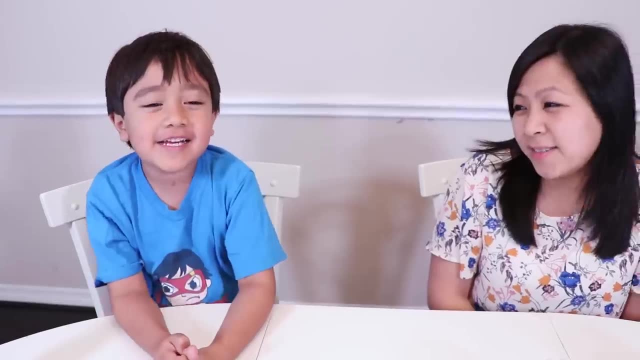 So you want to tell the kids what's a very important thing to do. The very important thing, The very important thing to do is wash your hands after you go potty or before you eat. We always make sure we have some clean hands, right. 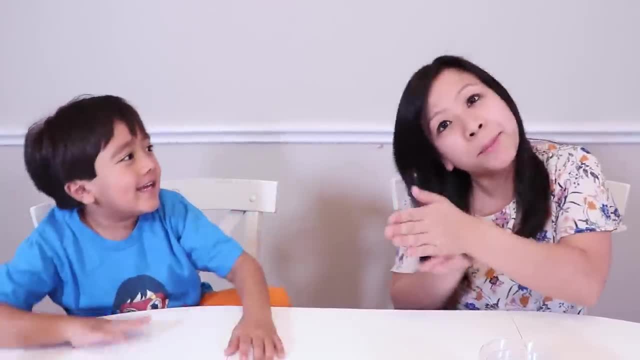 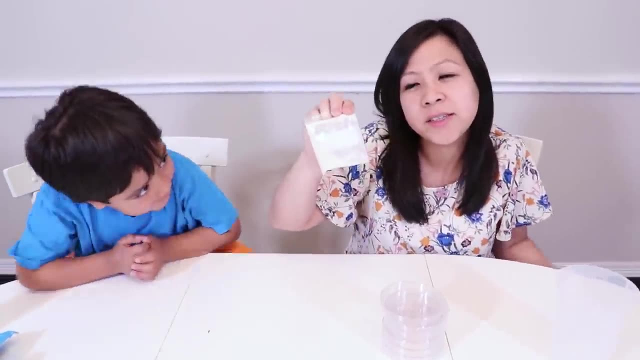 So every time Ryan gets to the restroom, he always sings A, B, C, D, E, F, G Or happy birthday, Or happy birthday, That's right. yeah, So this is called agar. This is like bacteria food. 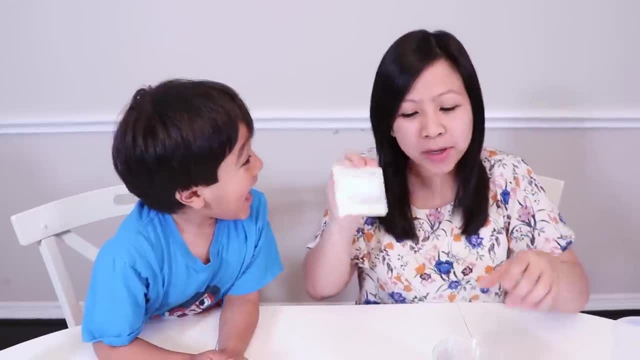 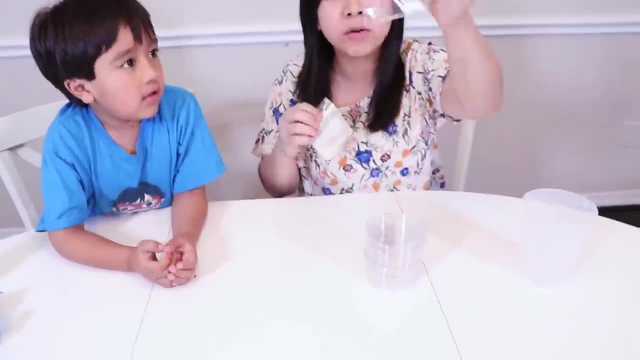 It says it's made from seaweed derivative. So what we're going to do is we're going to mix the bacteria food, Put it in the petri dish, And then we have these little cotton swab here. We're going to swab it. 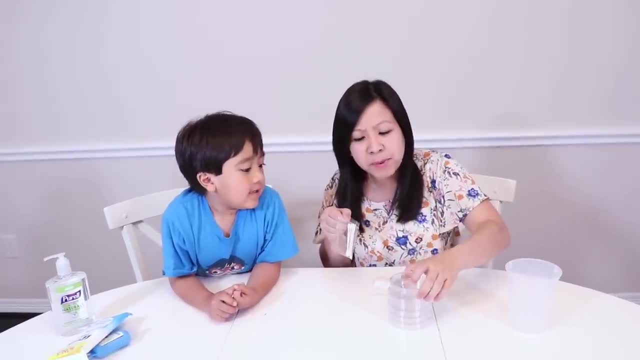 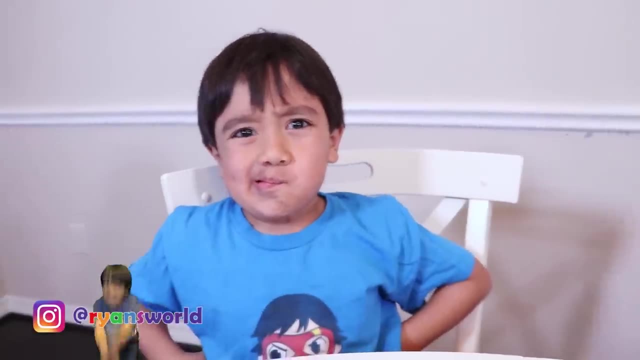 That's right. We're going to swab different places around the house, Put it in this petri dish And let's see what type of bacteria grow after one week. Are you ready? Ryan's doing a funny face challenge while we wait for mommy to prepare. 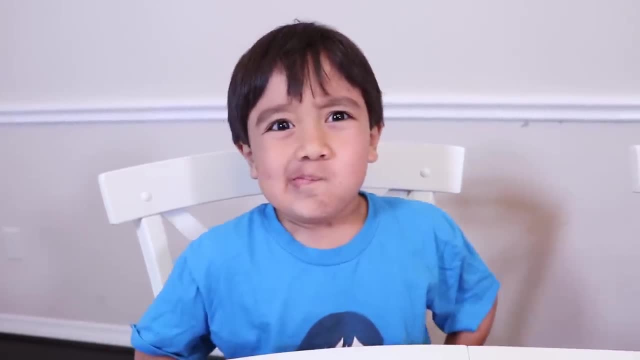 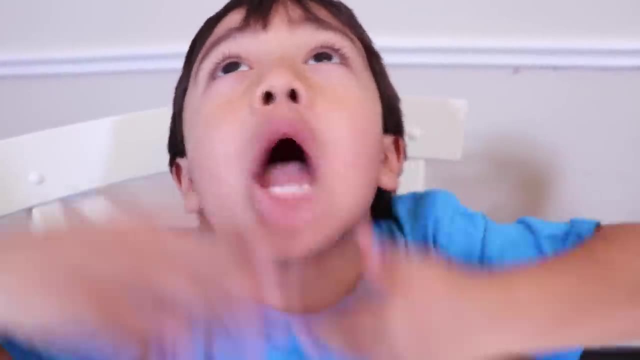 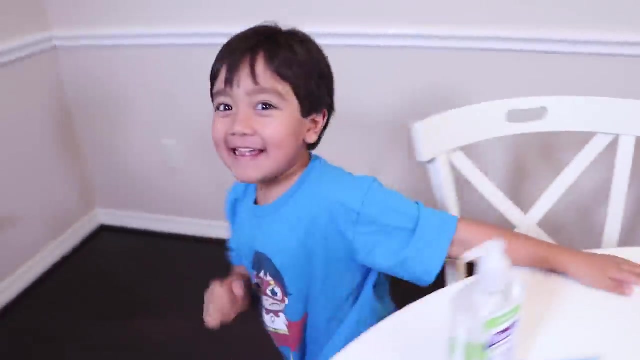 Ooh, that's a funny face. What's the other funny face? you can do The surprise face. What else? So, silly, Show me your dance move. Oh yeah, you have to stand up. Ryan's going to pour in the agar in the bowl. 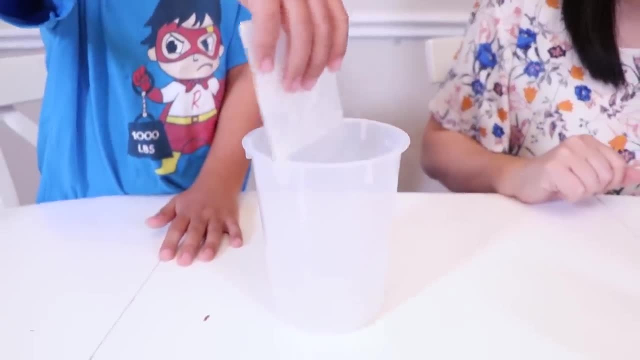 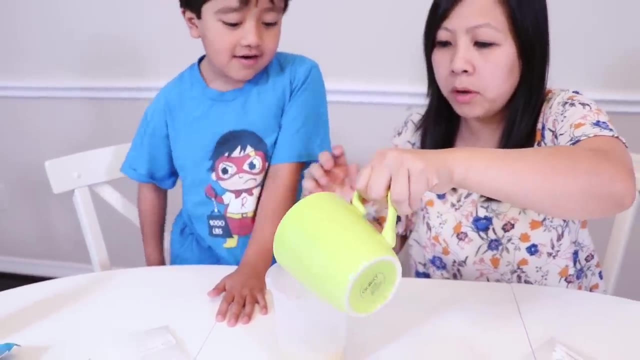 We're going to make some food for the bacteria. Yeah, they have to stay alive. And here's some hot water we're going to mix in. Is it hot? Yeah, It looks like coffee or orange juice. It does Wee. 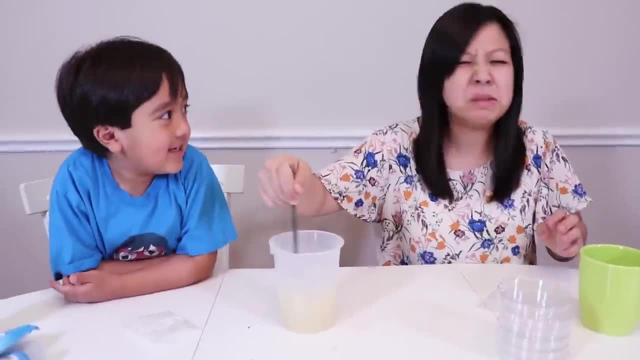 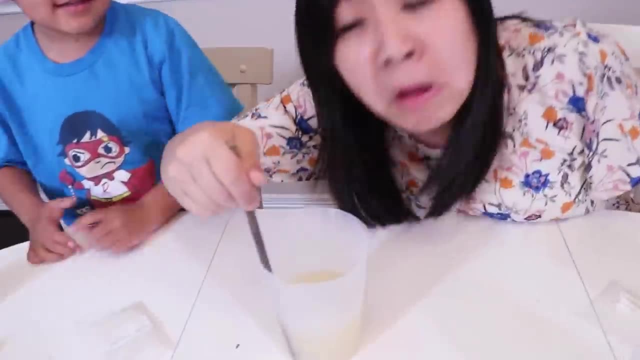 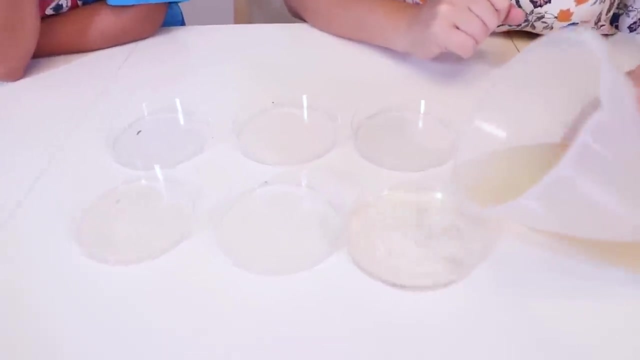 It looks like orange juice. It feels pretty jelly. It smells What it smells. Yeah, Ew, Yeah, bacteria. food does not smell good, So now I'm going to pour the agar into the petri dish. Be careful not to spill it. 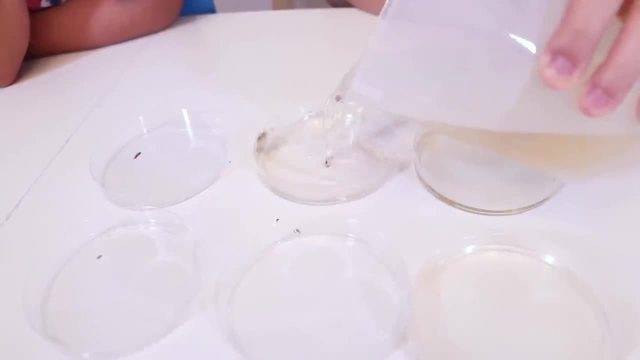 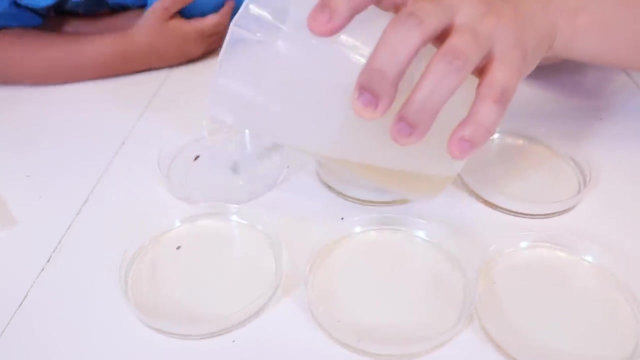 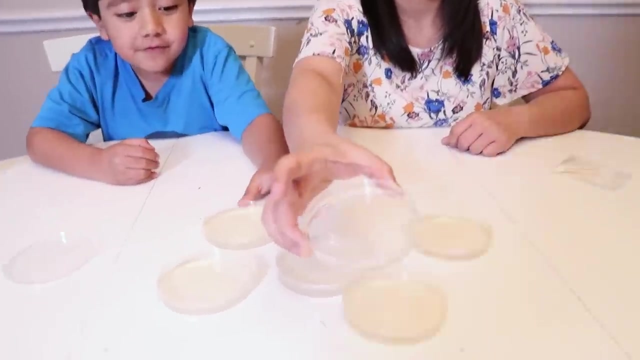 Wee, Wee, Wee. Oh yeah, we don't want to spill it right. This is some yummy food. One of the bacteria. Now the agar is solidified. That means it is nothing now, So if you touch it, 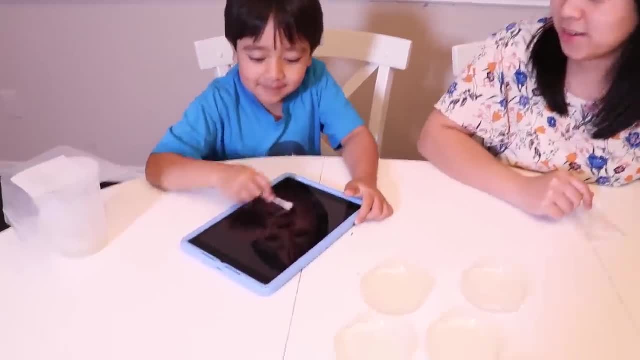 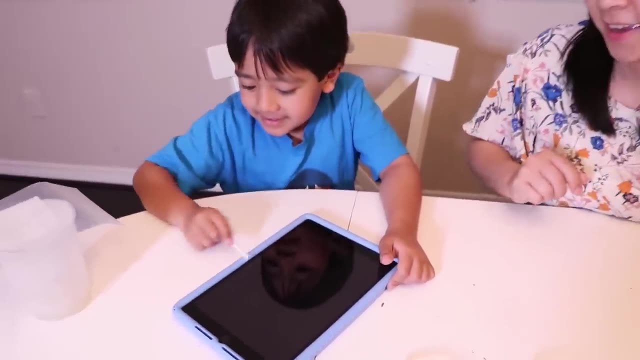 There you go. It's hardened, So I'm going to get the bacteria from my iPad Now. we all know it's super dirty, right? So many like this. now Maybe there has to be some on the side. It's grabbing all the bacteria. 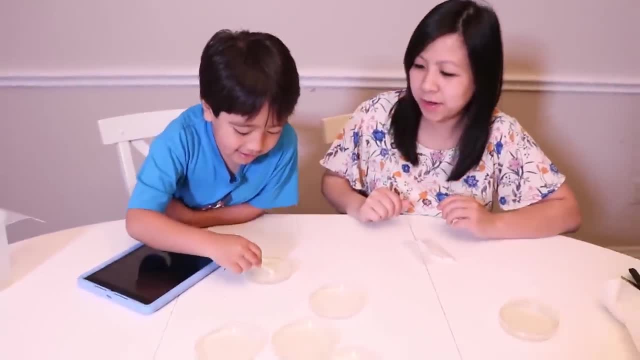 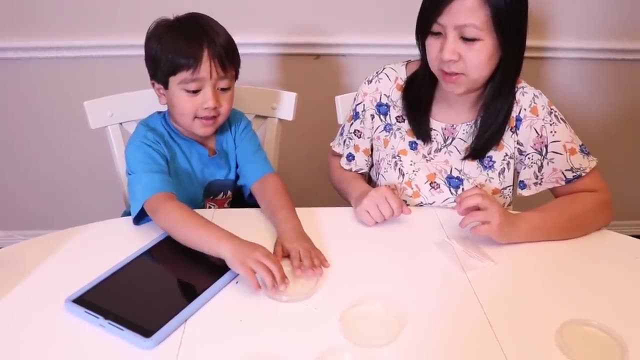 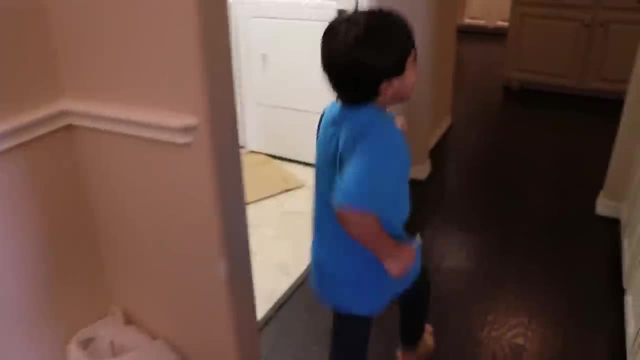 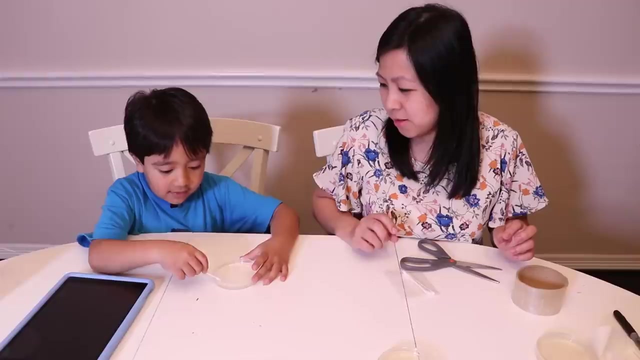 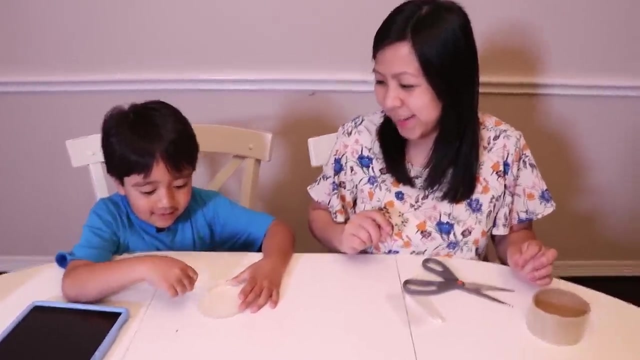 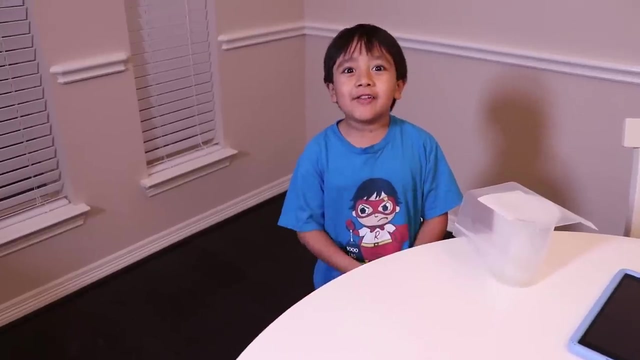 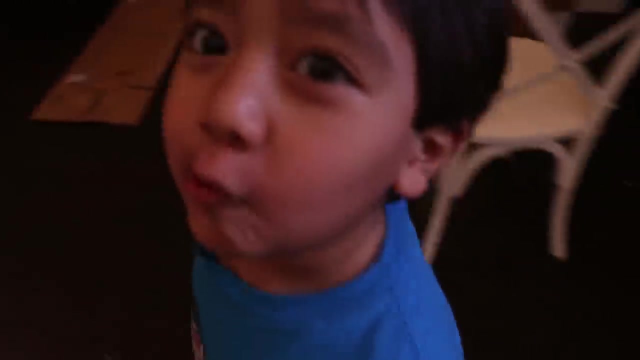 Now I'm going to test something far away, So this is from the table And the counter. Yep, Cool, Now let's close it Close. We all know the bathroom is dirty, So we're going to test something, Don't mind me. 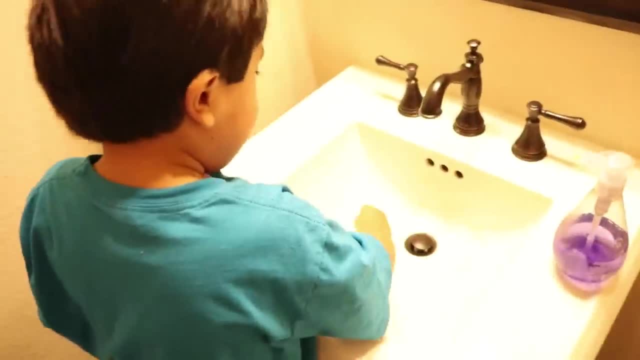 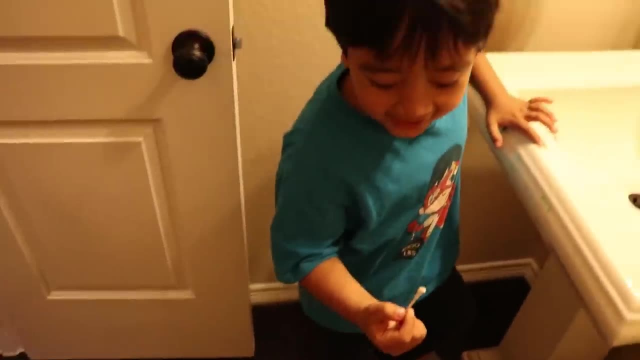 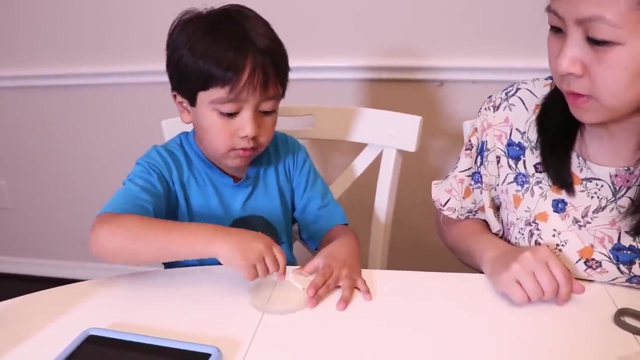 Ta-da. Oh yeah, Definitely know there's dirty stuff here, That one probably has the most bacteria on it. Oh yeah, I can see it. I hope you can see the bacteria. What color? Orange, Orange, So you actually can see. 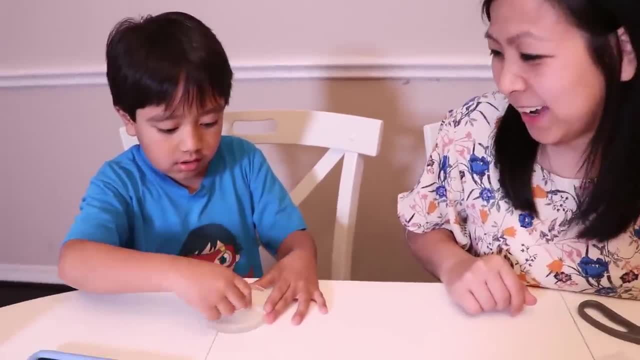 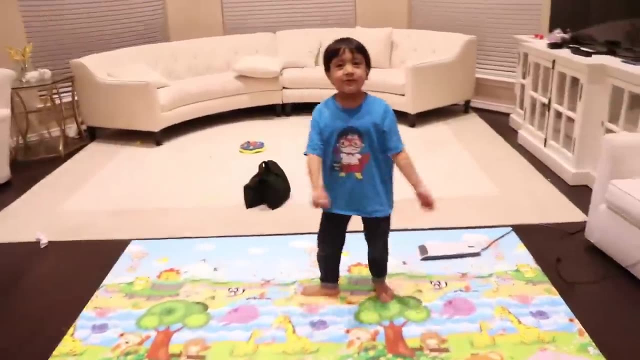 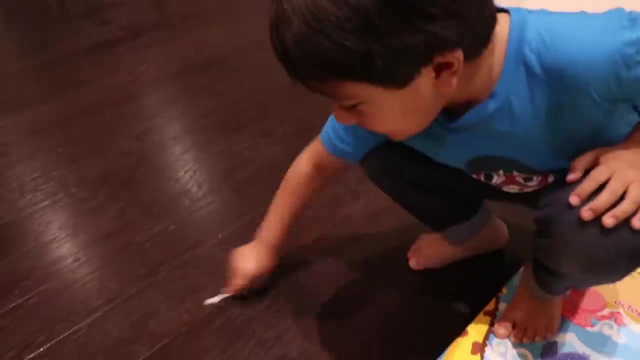 It's so dirty. Get on that cleaning. How well do it? What's wrong, Lauren, Are you doing Well? can we do the floor? We can do the floor. yeah, Floor might be really really dirty. Says floor. 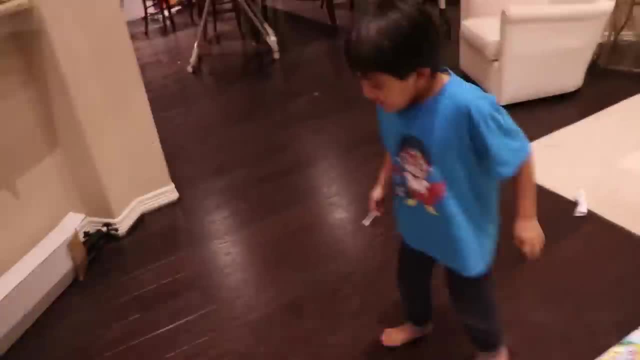 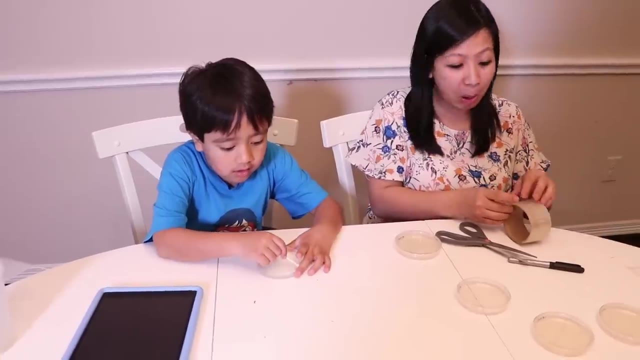 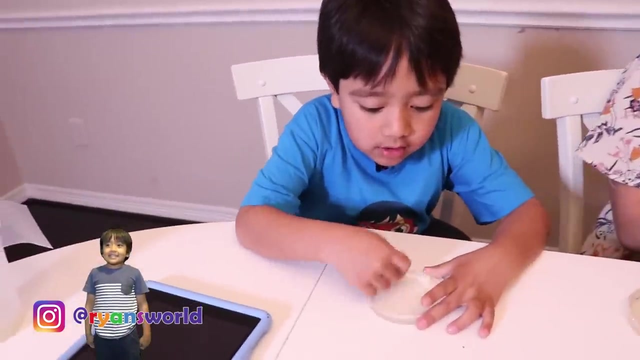 Oh, wow, That's good. ultrasounds. We're going to have to close the house. Let me guess some dirty stuff. Hai ss, Definitely dirty stuff. Let's test it out. No, Somebody needs to clean the floor. I can tiny bit like see where I'm rubbing. 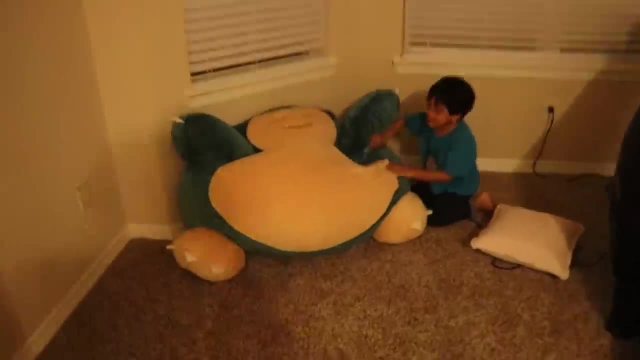 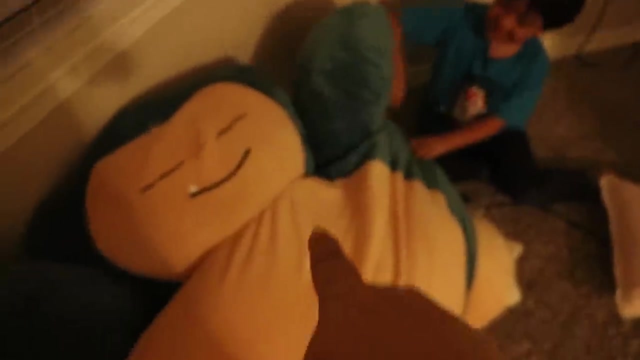 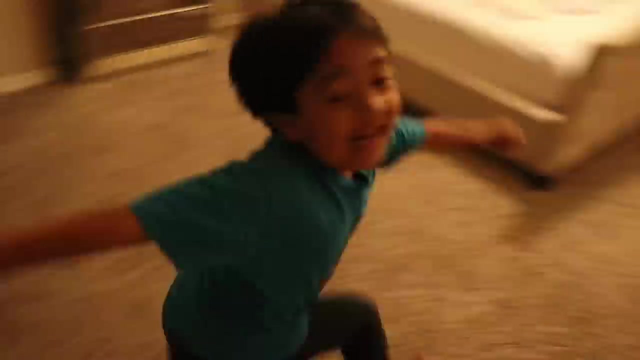 Of course the pillow is dirty. Just kidding, I'm going to do snow like dogs. Yow Nasty, Definitely dirty Snow. looks like he's having fun. That feels actually good. Scratch more, please, Scratch more, please. Got it. 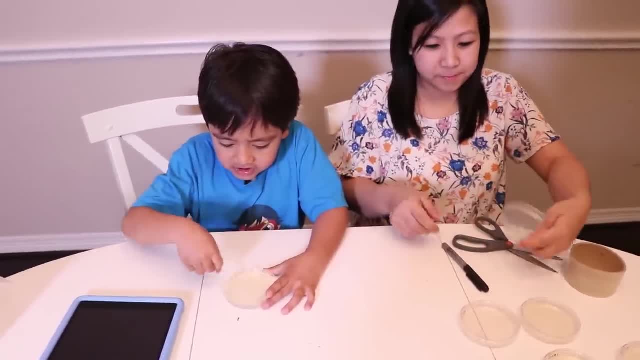 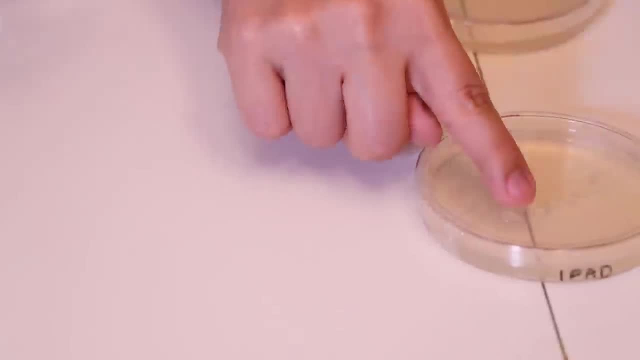 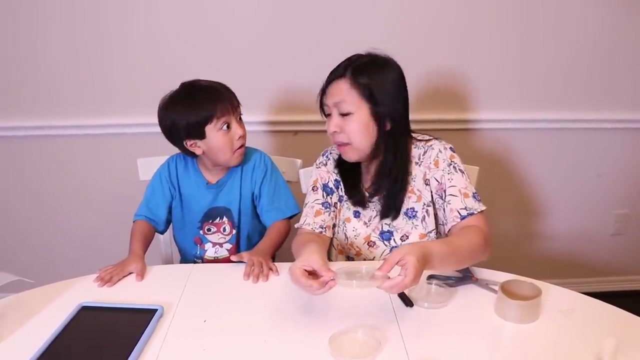 Alright, that's good, Maya. So on all of these I labeled them. So this one I labeled mouth iPad, And then I'm also taping on all of them Because we don't want the bacteria to get in. So once we have bacteria on here, 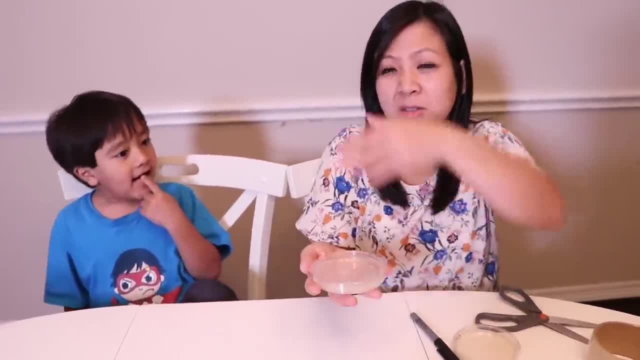 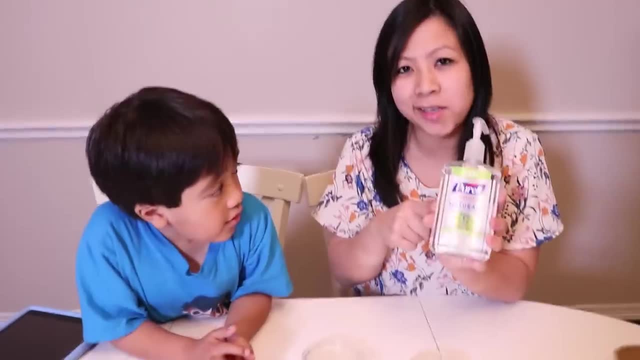 we do not ever open the lid Because we don't want bacteria to go into the air, So it stays closed. So before we finish the experiment, I'm actually going to try hand sanitizer and see how effective it is, So we're going to open one of them. 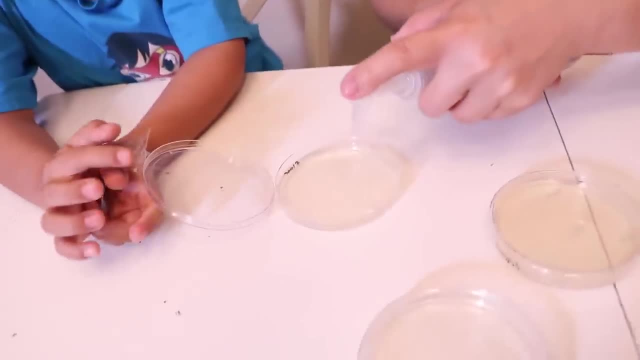 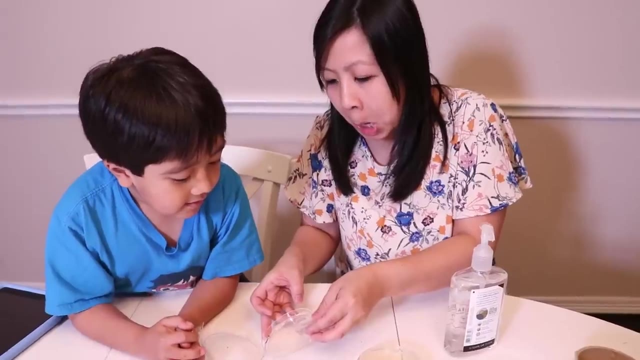 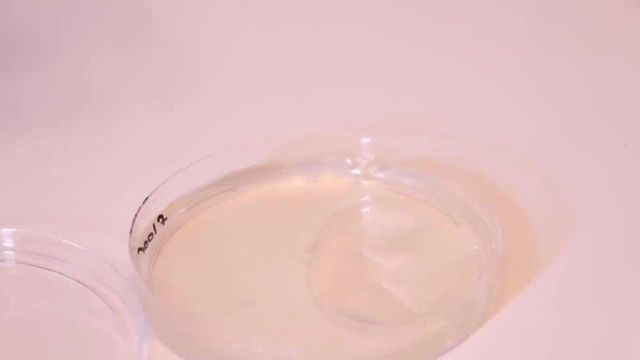 and just squirt hand sanitizer on one side of it. Ah, this is the floor one. Yeah, so if I put hand sanitizer on one side, that means that side shouldn't have any bacteria. Right One side of it has hand sanitizer and one side of it has hand sanitizer. 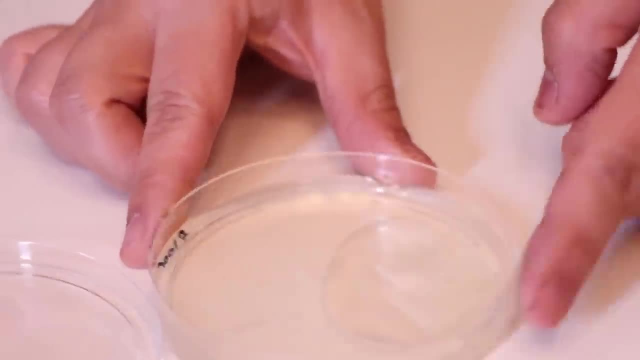 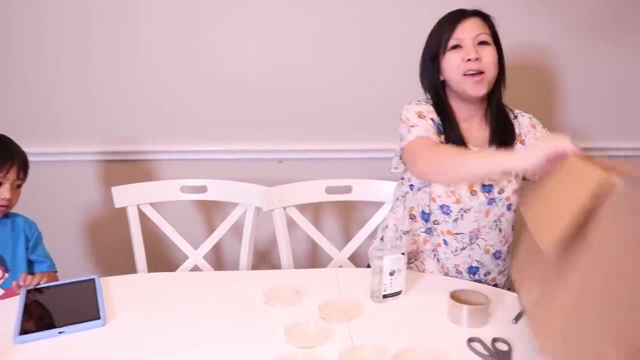 And one side of it has nothing. Yeah, so where the sides of the hand sanitizer, there shouldn't be any bacteria growth on it, right, Hopefully. Alright, close it shut, So we have an empty box here. What we're going to do is: 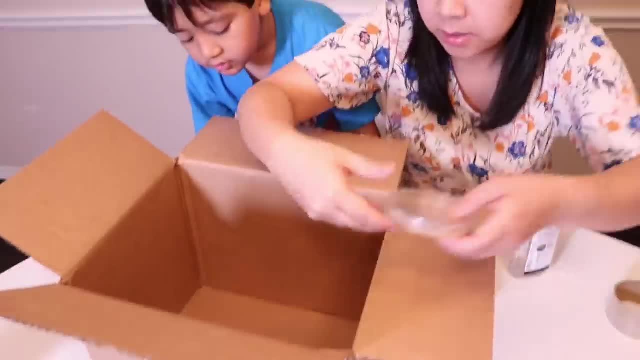 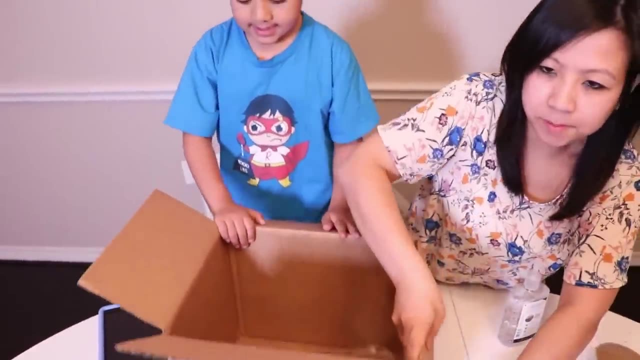 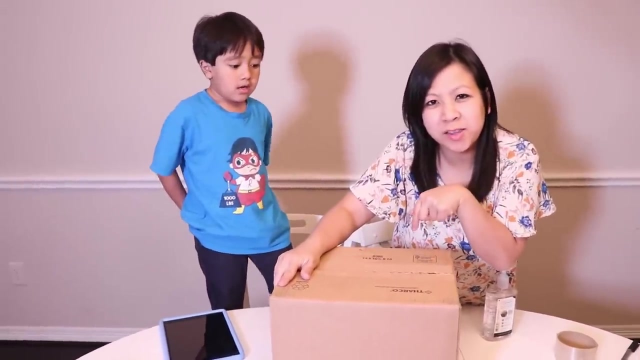 we're going to store all the petri dish in here. There we go And they're still tight, So we're going to close it, put it in a warm place and every couple of days we're going to check on it to see if any bacteria are growing. 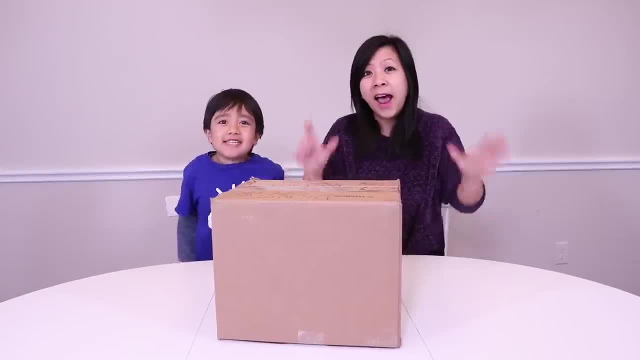 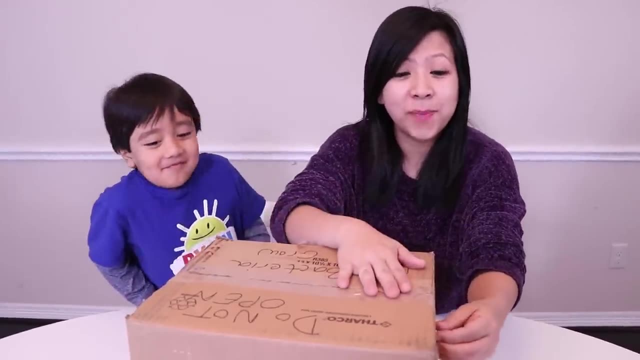 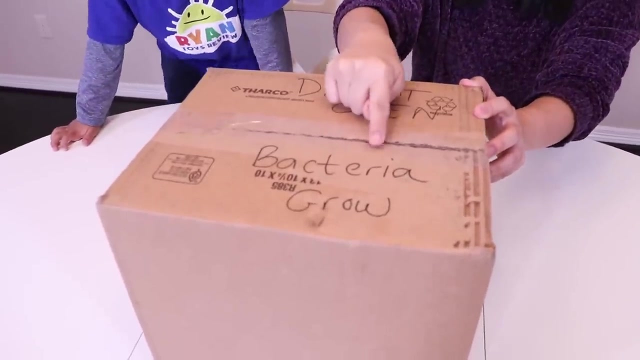 Okay, It's been seven days, So let's see how much bacteria has grown. I'm excited to look at all the bacteria that has grown. I'm scared. He said: do not open. Sounds scary, Do not open bacteria. What if you open it? 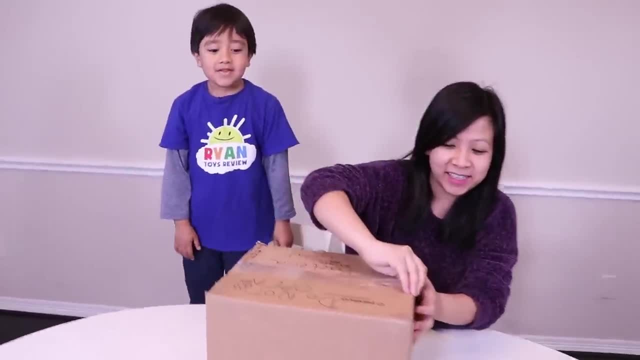 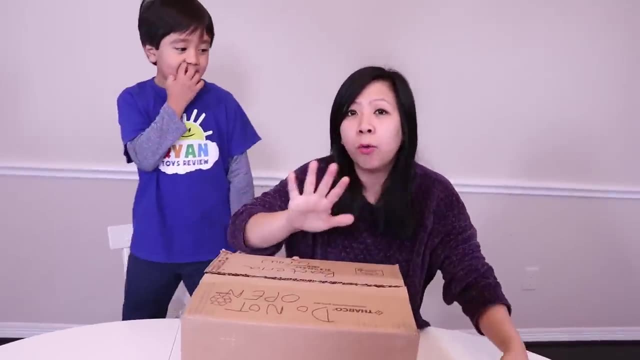 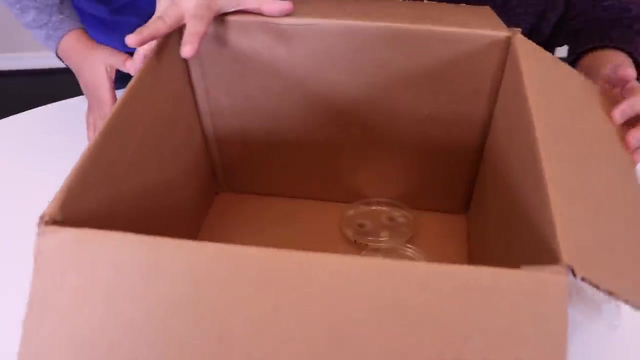 and it just starts coming out from the box. Don't say that It's contaminated in the box, It's fine. We just do not open the petri dish. That's all You got that, Ryan. Don't touch it. 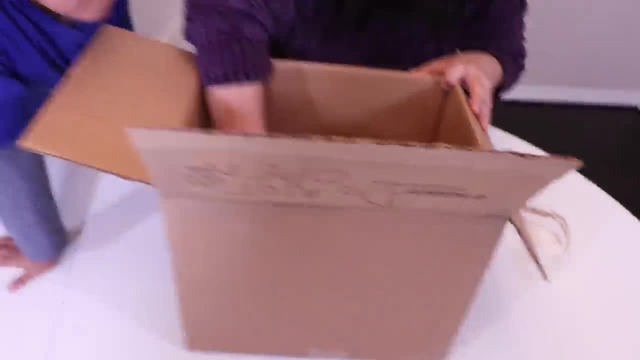 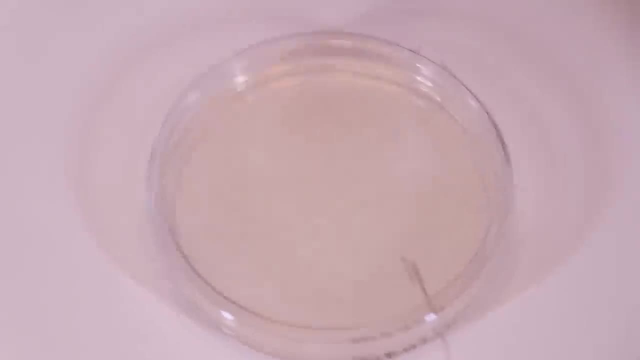 Oh wow, Take it out. Okay. so number one: we got mouth. Oh, my mouth isn't so bad. Mommy's mouth is clean, Alright. number two: This is from the counter. We gotta wash our counter. Look at that. 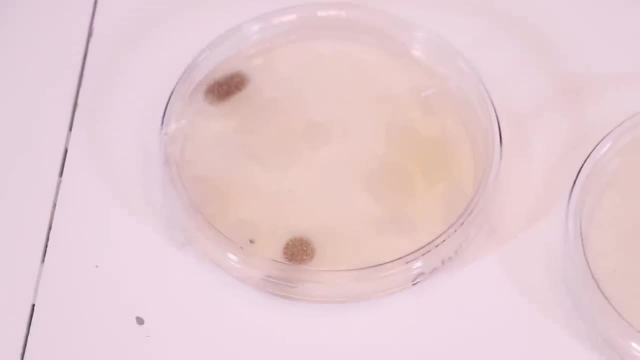 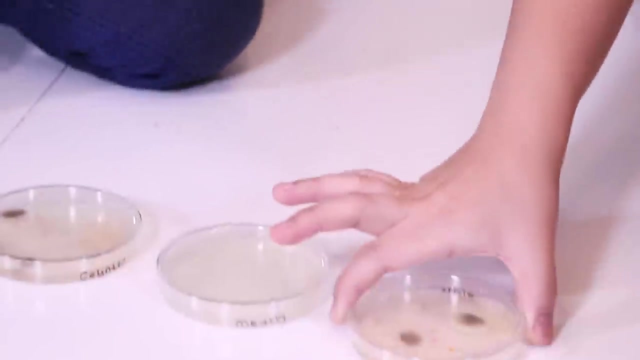 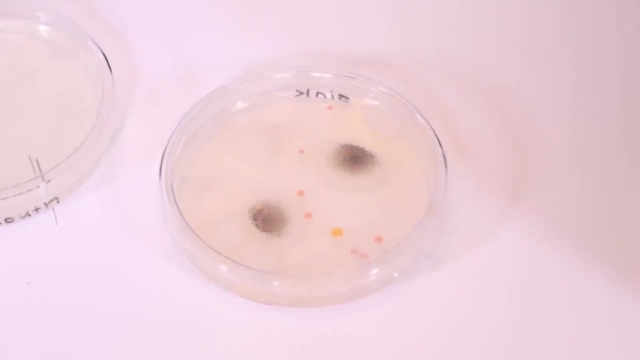 Wow, Look at the different type of bacteria. Yeah, Okay, number three: This is from the sink. Whoa, It's huge. Wow, Different colors too. What is that orange thing? This is a major bacteria colony coming up. It's huge. 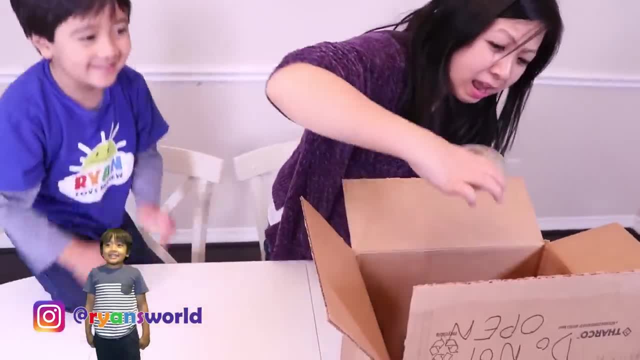 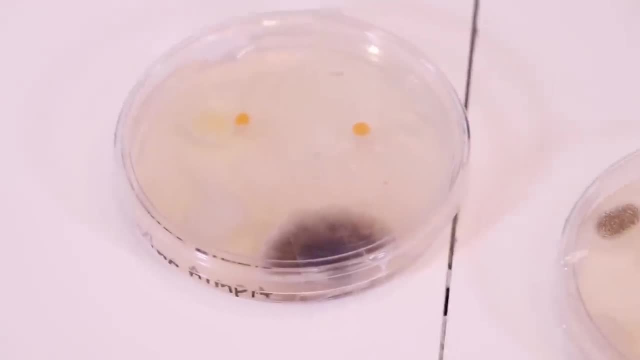 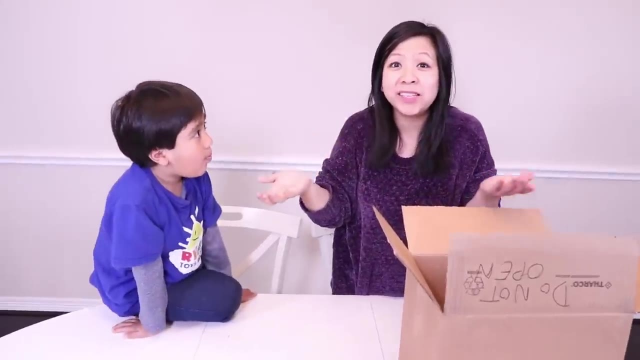 Look at this. I'm scared. It's from Snorlax's armpit. No, Snorlax, Wash your body. It's black too. It's super black. Snorlax, We need to start washing toys. 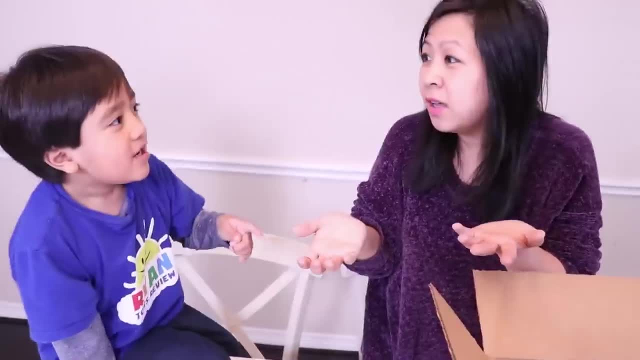 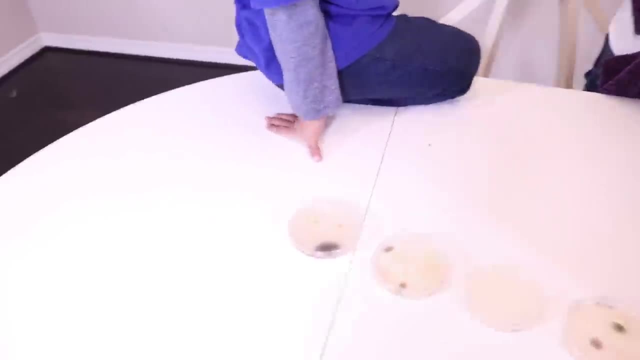 That's what it means, right? It's very important to always wash your hands. We never use the thing where it cleans the toys that much. Yeah, we need to start washing our toys more, And Snorlax's armpit, obviously. 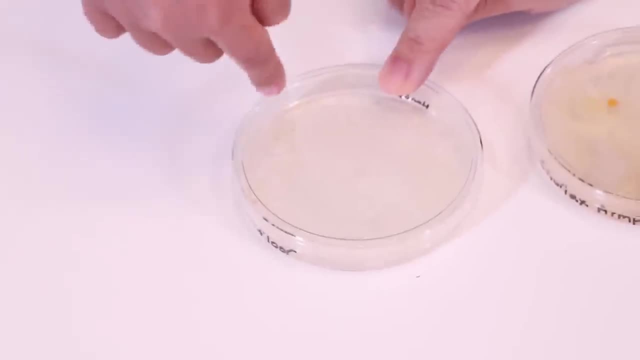 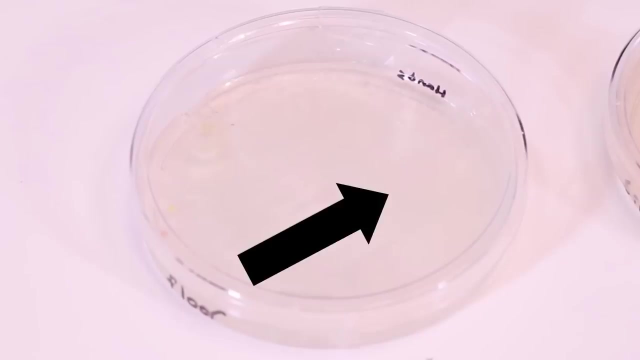 Alright, so this is from the floor, So the floor isn't super bad if you look at it. Really. Yeah, It's just on the side a little bit. Oh look, And here's the part with the hand sanitizer And hardly any bacteria. 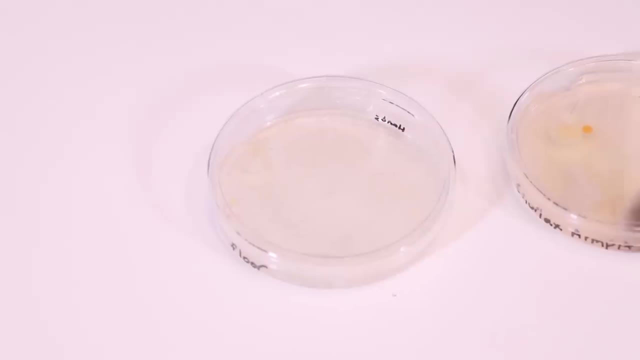 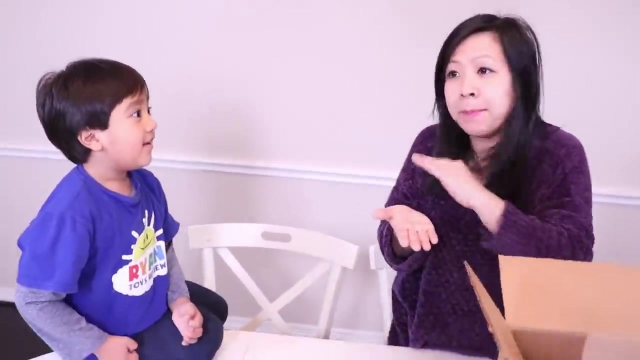 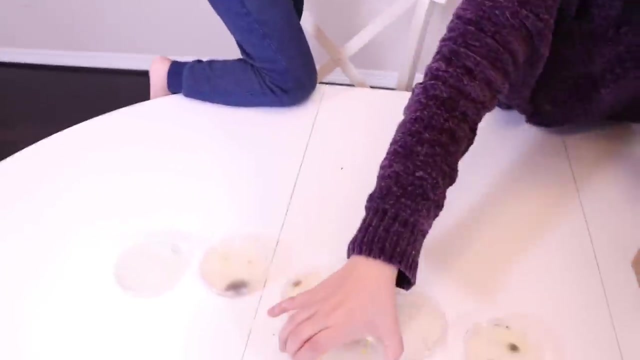 is growing. That's cool. No, not every floor. Okay, Ryan, this is from your iPad, So we definitely need to wipe down our iPad every day While they clean. Uh-oh, Look, this is from Ryan's iPad. 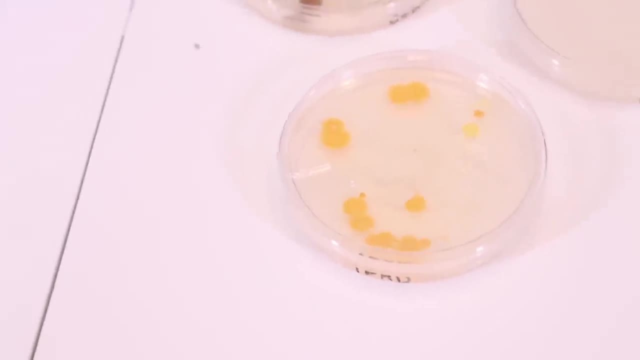 Let me see. What is that orange thing? What Do you see? like the same thing happening in some other stuff too. Yeah, So the sink also has it: The orange type of colony, the iPad And Snorlax's armpit. 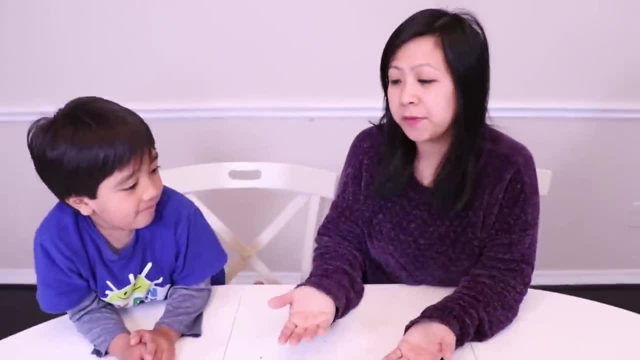 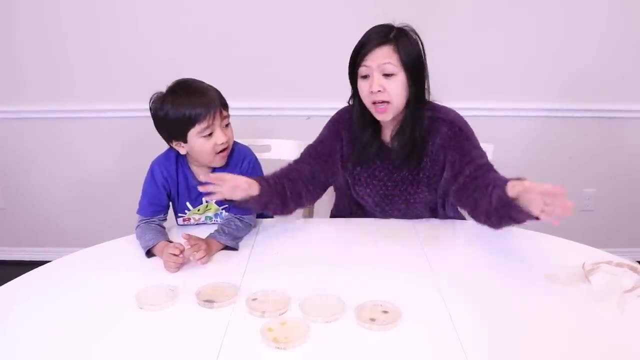 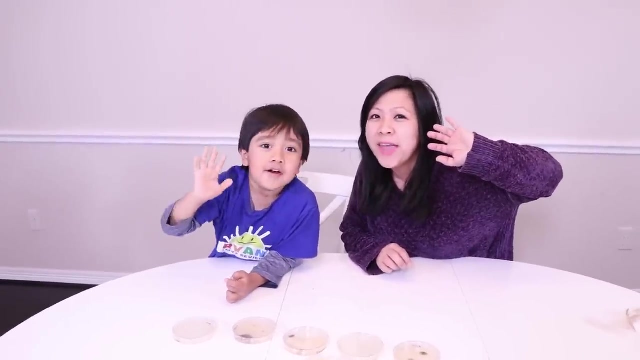 That's interesting. Okay, Ryan. so what did we learn from this experiment? We need to wash stuff. Yeah, wash stuff and wash our hands and sanitize more, right, Alright, guys, thank you so much for watching our bacteria experiment. 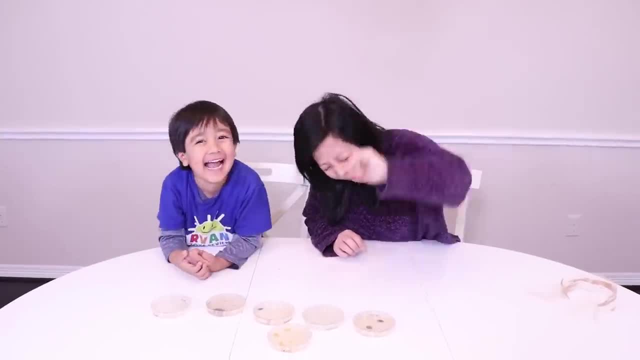 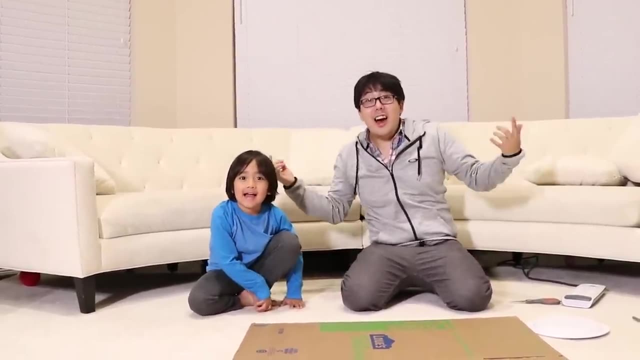 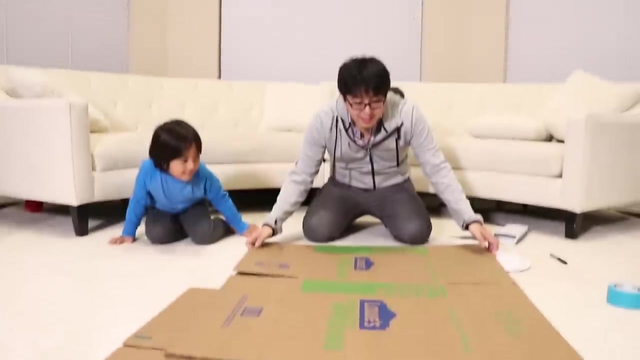 Bye, Bye, Hi Ryan and Daddy, Hi Mommy. What are we doing today, you guys? Today we're building giant air bazooka Out of cardboard. First, what we need to do is make a box Ooh, like a box fort. 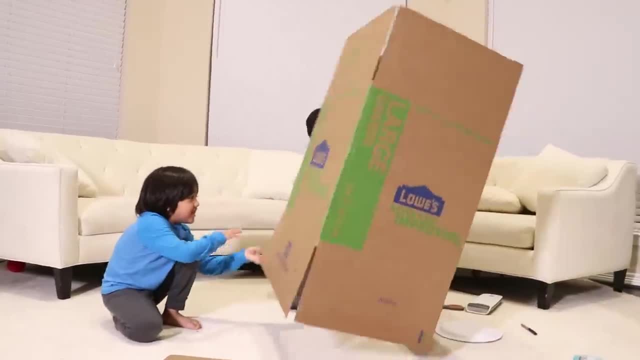 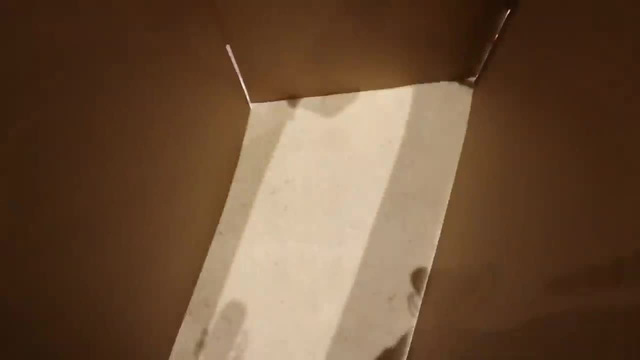 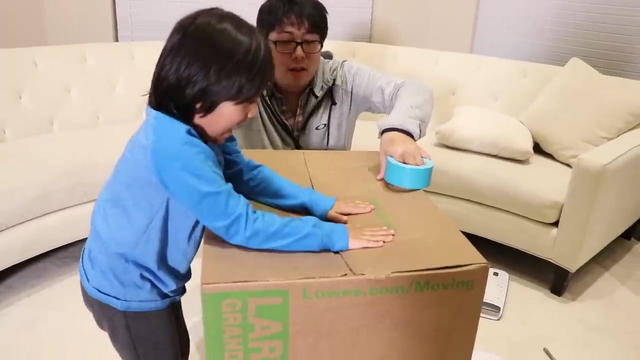 Yeah, Box fort, challenge Like that, Yeah, like this, A giant one where I can go inside. Don't go inside, And then I'm gonna be a bullet. You're gonna come out like a bullet. Yes, Can you hold this box so I can tape it. 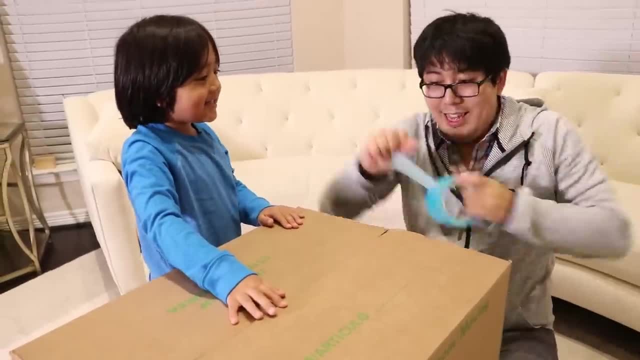 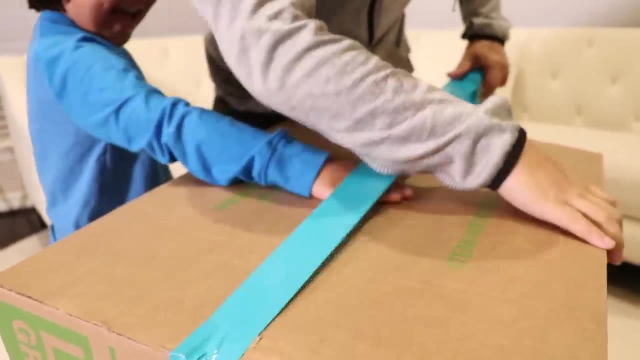 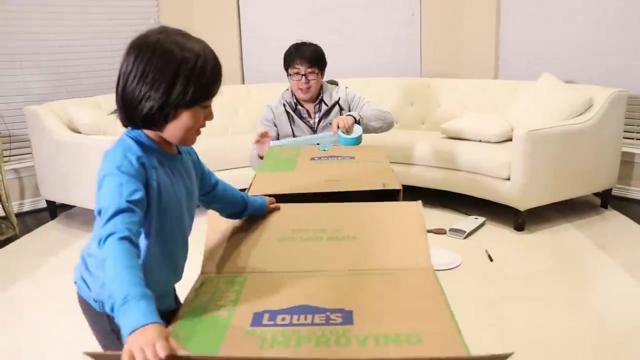 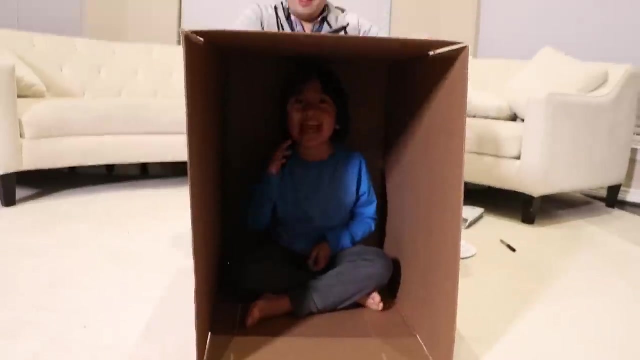 Thank you, Don't tape my hands. Watch out your hands. Thank you, And now it's size. Okay, Whoa, that is super long. Are you connecting it With a tunnel? Where's Ryan? I'm safe That burned down. 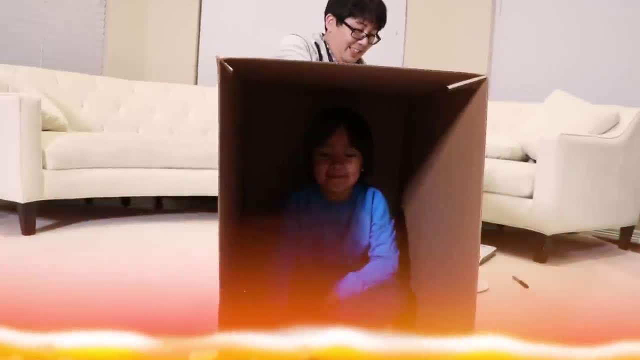 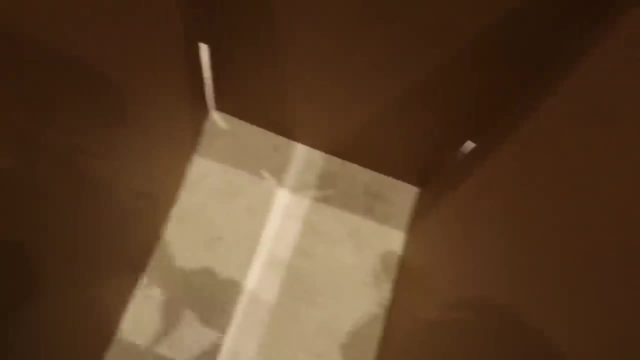 from lava. Oh really, Is that your secret base? Secret base. Ryan hid somewhere and we have no idea where he went. Where is he? Ryan, make a noise? He's in here. Nope, he's not in there, But it's closed off. 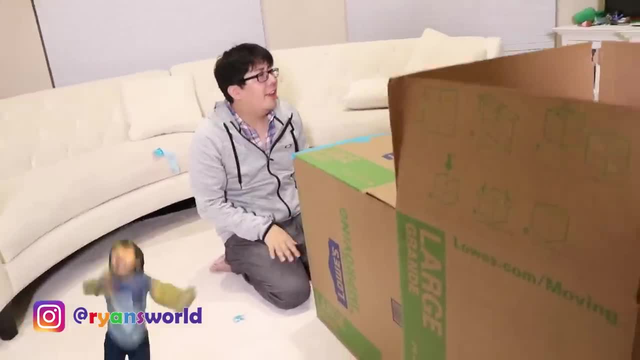 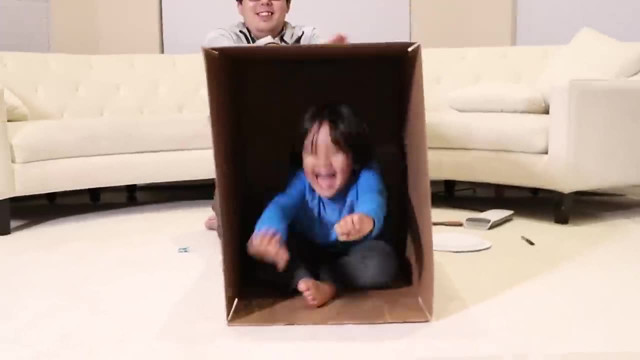 so I don't know what to do. Ryan make a noise, Make a noise, Ryan, Make a noise. Oh, He's in this box here. Let's see. Let's see. Found you Taping the top side too. 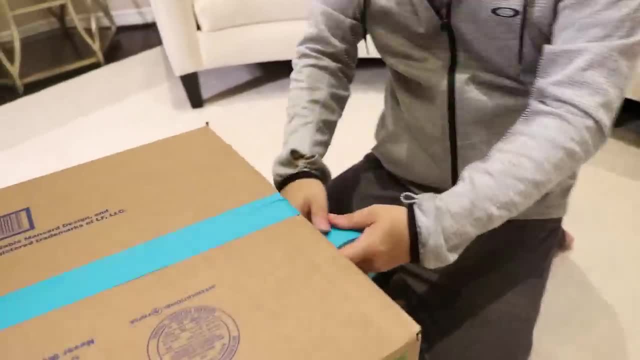 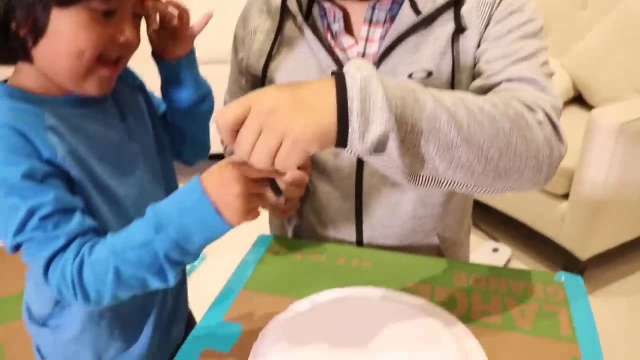 So I can not get in. Yeah, No more getting in the box. Next we're going to make a hole in the box with this circle. Alright, Ryan, Here's your pen. I'll hold the dish so you can draw the circle. 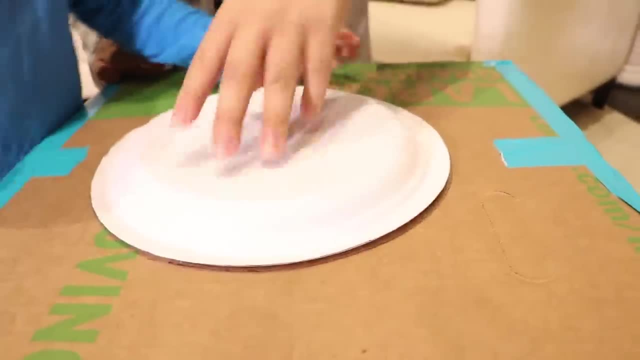 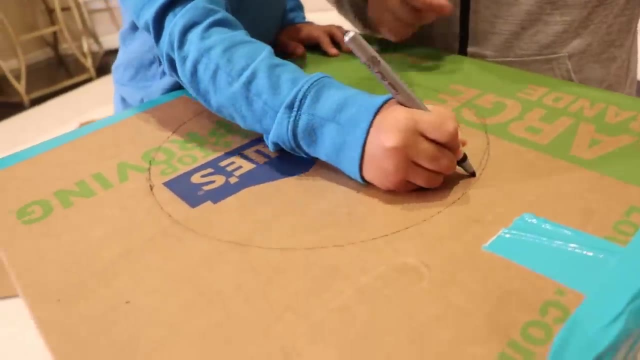 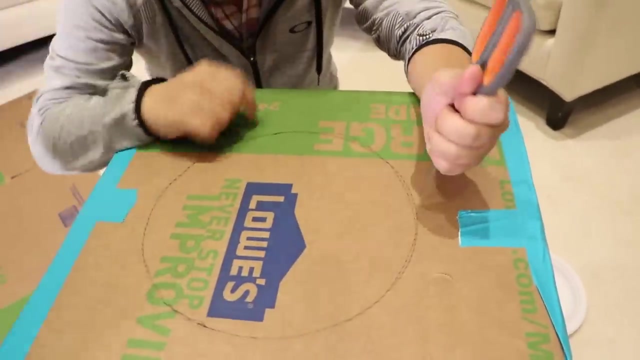 Let's see Ta-da. Oh, Good job, It's perfect. I feel like it's getting worse. Ryan, Now I'm going to cut it out. It's going to be very hard. Yeah, I'm going to cut it out of this circle. 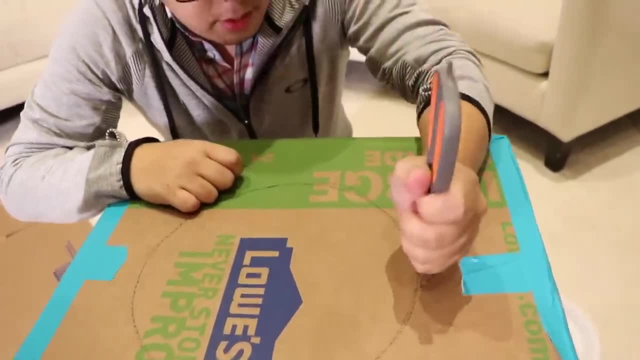 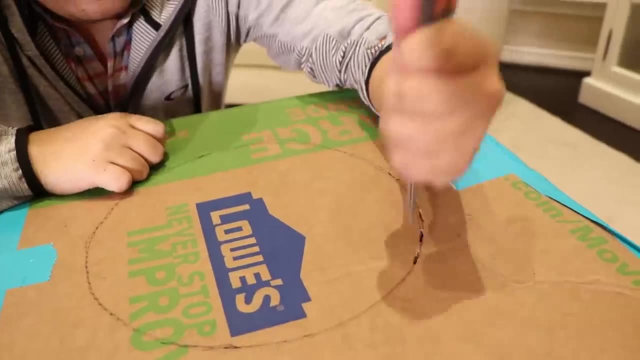 Dad's going to do dots first, then he has to make enough room for him. So this is probably a step for grown-ups, right? Yeah, because you have to use scissors, A bunch of holes, and then I'm just going to cut it in between. 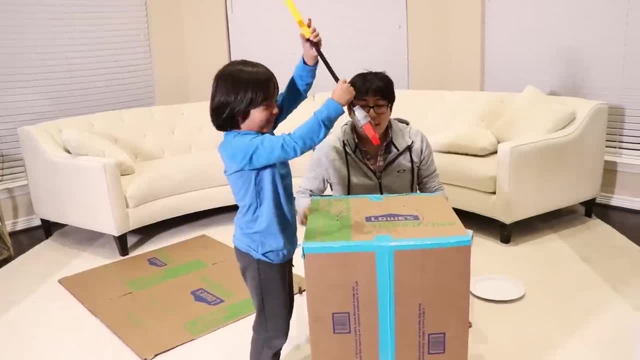 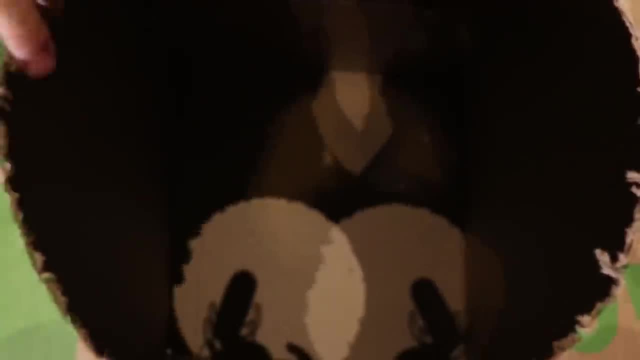 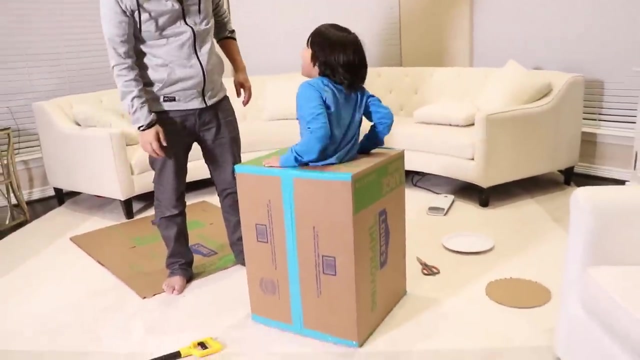 Even more time. Punch out the hole. Oh, Oh nice. Oh nice, nice, nice, Good circle. Good job. I think you're too big for the circle. Oh no, You fit. What if it shoots out you? 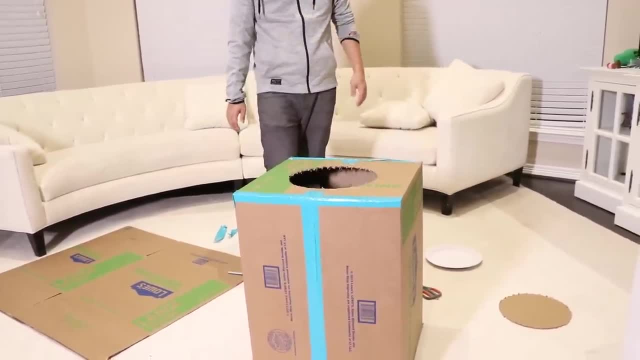 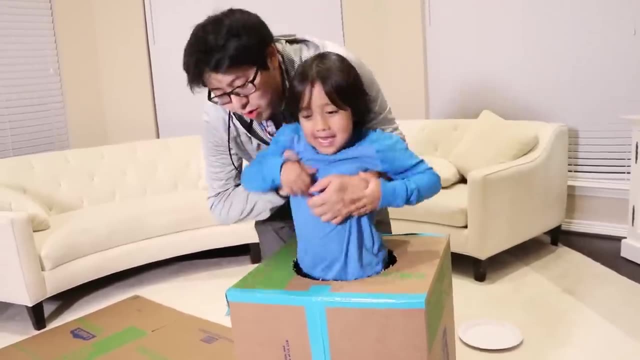 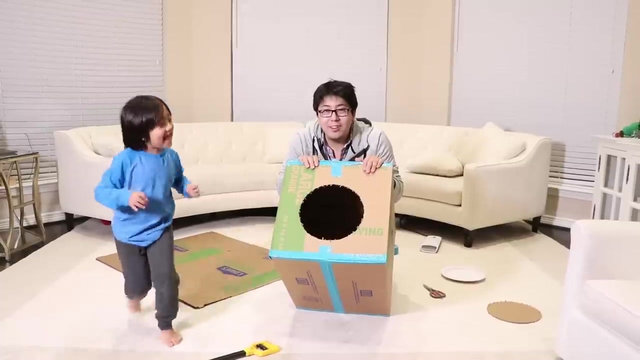 This is an epic hiding spot. Oh yeah, Wait, Where's Ryan? Where Ryan? where There he is. It shoots you out. Okay, kids, This is it actually. It's that simple. This is air bazooka now. 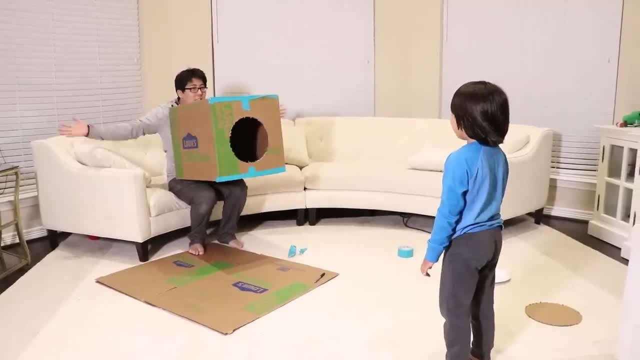 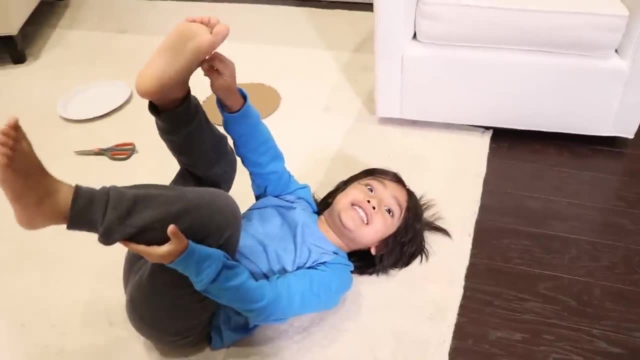 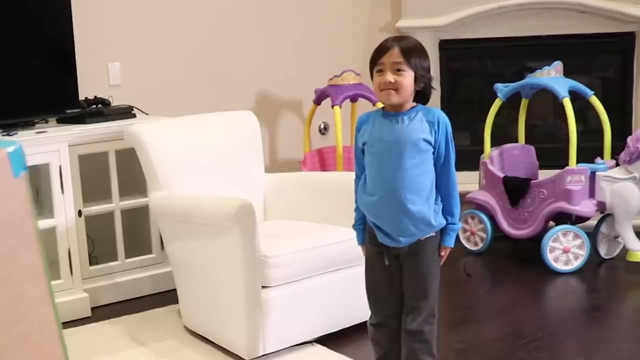 You ready, Ryan? Yeah, Stand right here. Three, two, one. Ah, That's your phone. That was actually air, Really, Yes, It feels good. huh, Wow, You feel the air. Yeah, Try it to Mommy. Okay, I want to try. 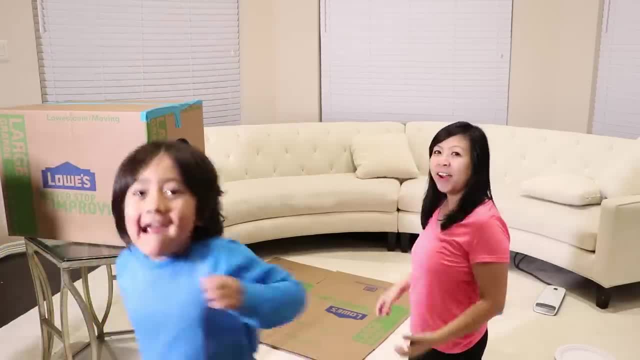 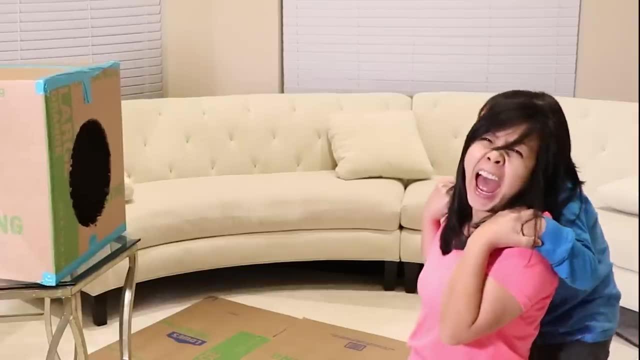 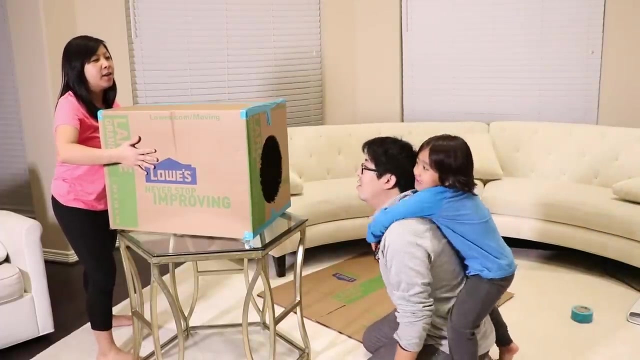 Mommy's going to try. Let's see if I can feel any air. Oh, a little bit Ready guys. Ah Ah, Ah. All right, you guys, Are you ready? Let's put my face right here. Simple as that, Ready. 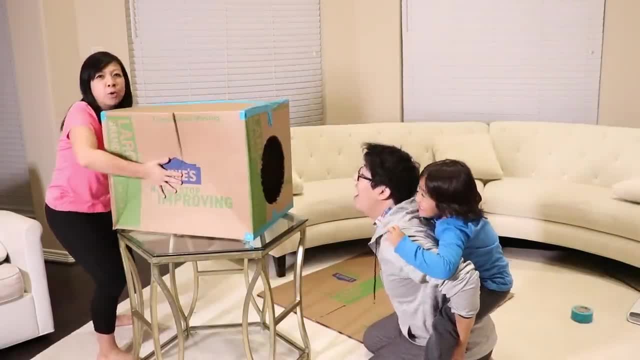 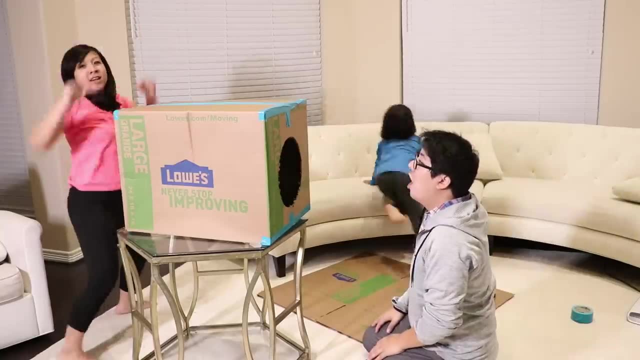 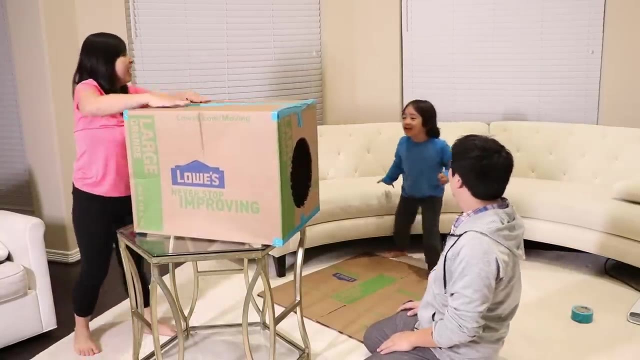 Ready Ryan. Boom, You feel it. That was nothing. I'm not blocking it. All right, I need to. Ah, Ah, We're in each other's Okay, okay. okay, My turn. All right, I got it. 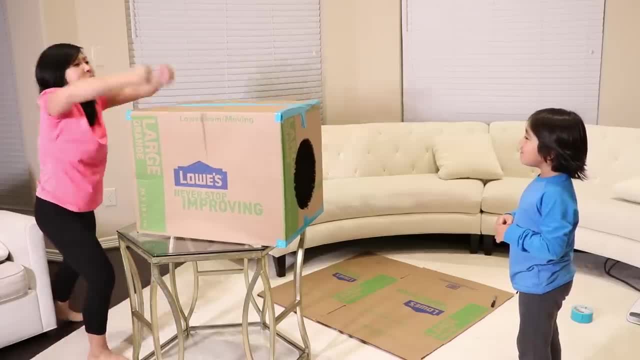 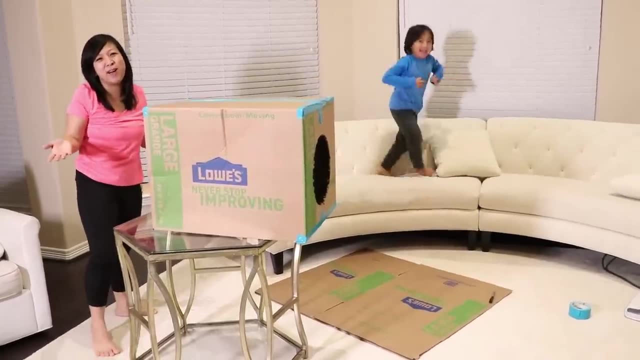 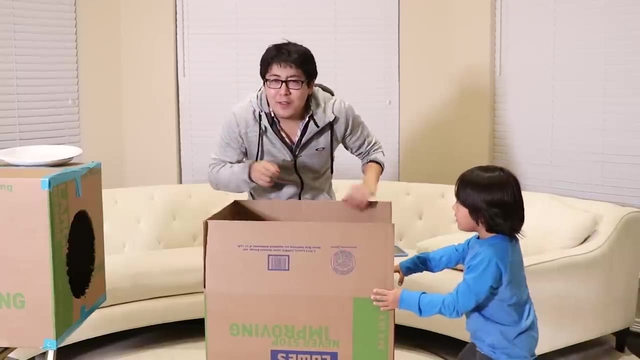 All right, Let's see. Don't run me. Ah, Nothing, I'm as strong as Daddy. that's why Now we're going to make another bazooka, but with smaller teeny holes, So we can experiment and see if it makes a difference. 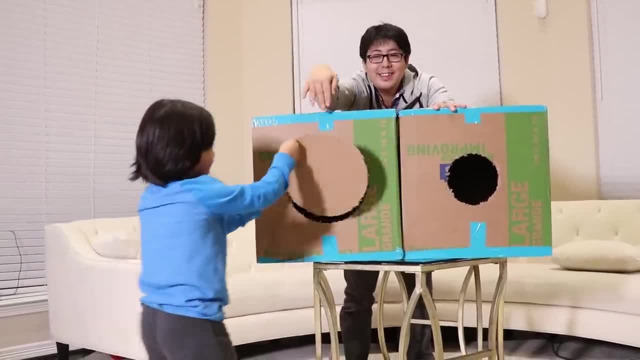 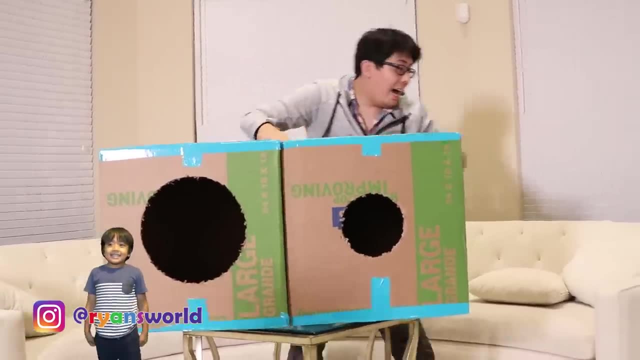 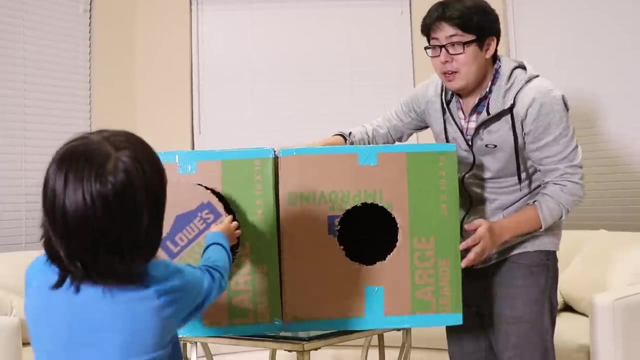 Those are two holes, A big hole and a small hole, And just to show you the difference between these two, how the air come out, I have this smoke machine here, So I'm going to put smokes in these, But then we need to cover it. 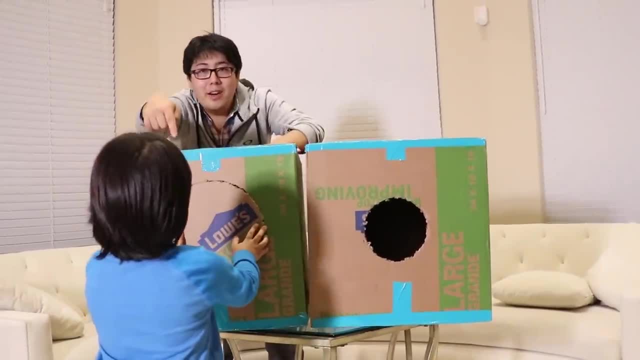 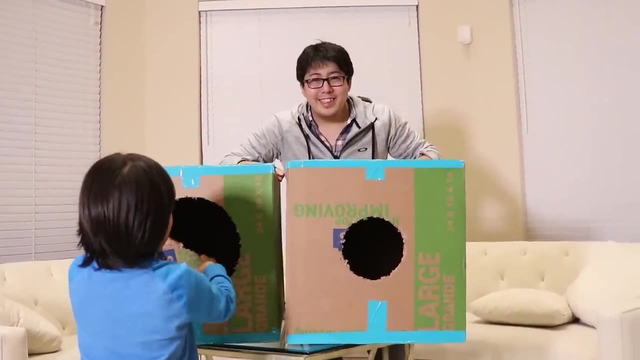 And then we cover it and when we shoot, you can see the smoke come out and you can see how the air moves out of the box. Yeah, so it's called a vortex generator. Oh, that's cool, Sounds fancy, huh. 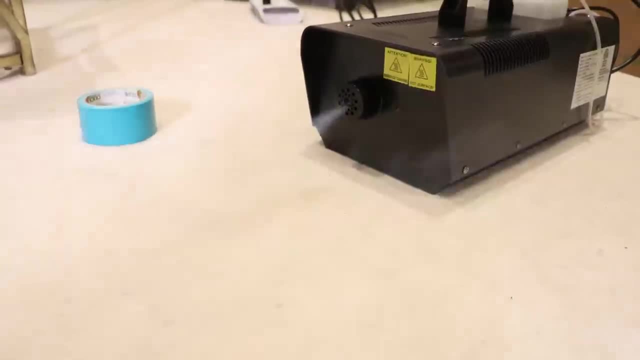 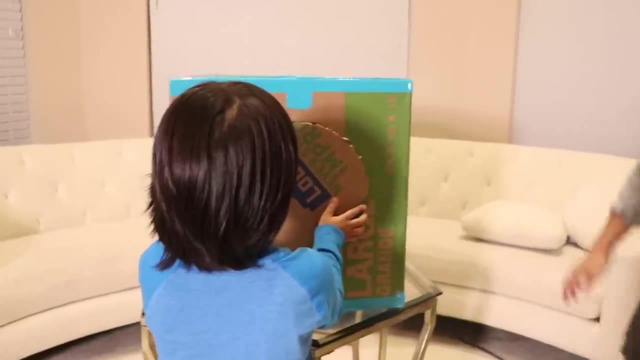 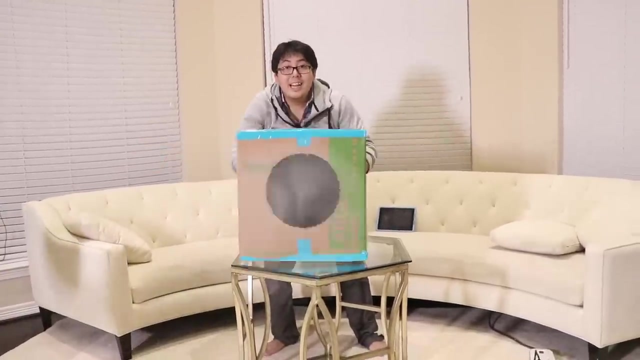 Turn it on. Ah, Ah, Stopping here, All right, Hehehe, Ready, We're trapping the air. I'm going to shoot at your camera. All right, let's see. Wow, What Did you see it? Yes, It looks like a fireball. 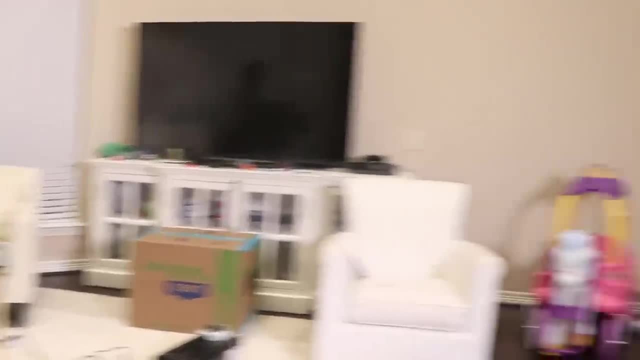 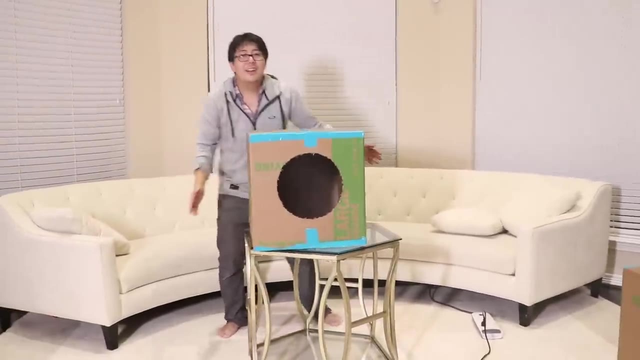 It looks like a fireball. Wow, Wow, See, it looks like a fireball. Whoa, whoa, whoa, Whoo. I want to try. Oh, I feel the air. Wow, Whoa, Did you feel the air? 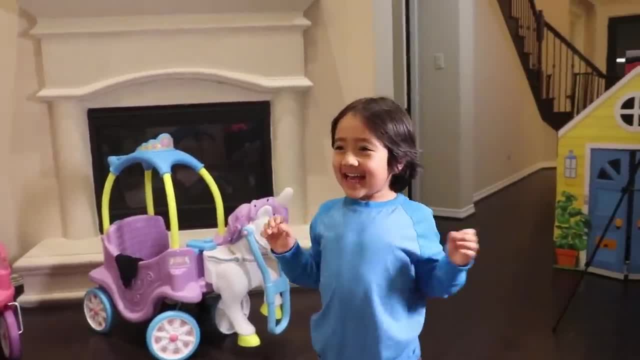 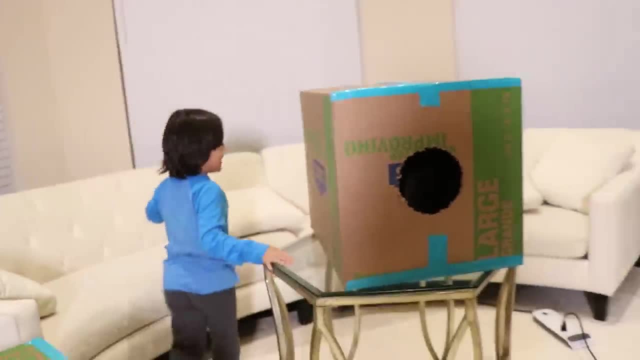 Now it's just air. That was a big hole. Now we're gonna try a small hole. Yeah, let's see what the difference is, And I'm gonna be the first, Okay, Oh, you're gonna try it. Okay, Yeah. 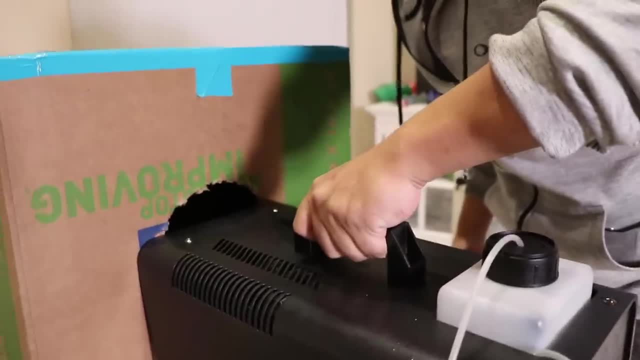 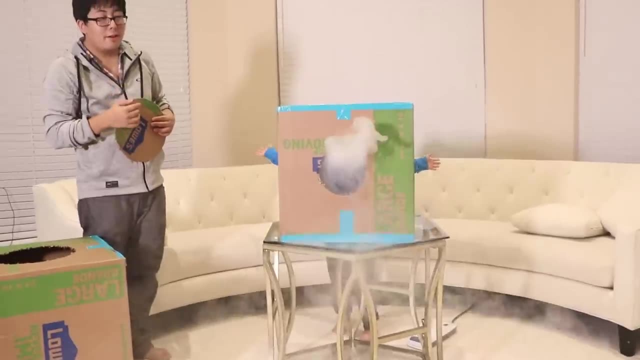 It's gonna look scary, right? Oh, this one. I can't even put the smoke machine inside. Oh, we're done, Stick it out. Okay, go ahead. Wow, You see it. Yes, Wow, this is stronger. 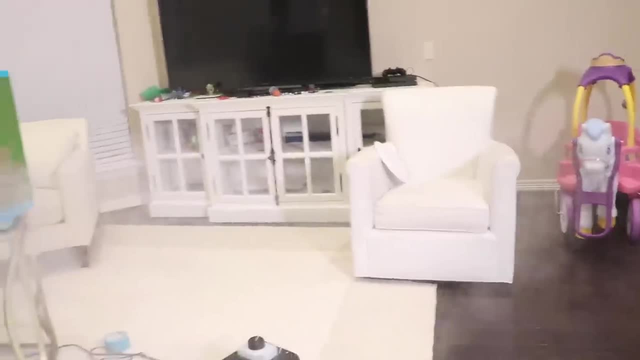 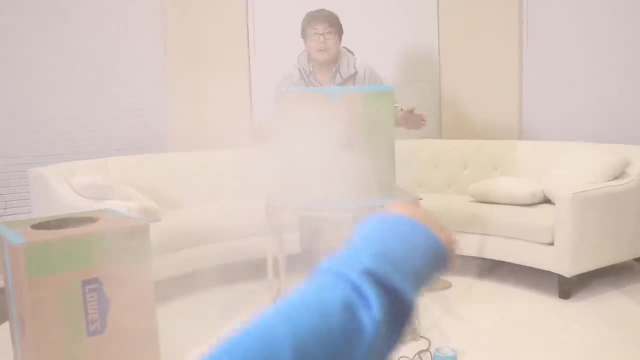 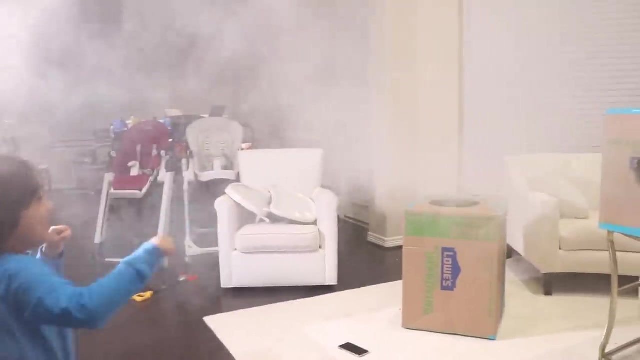 It looks like a snowball. Wow, Dad, you look. Woo, I'll just slow it down. Woo-hoo, You know what? Uh, Mm-hmm, There it is. Uh, Uh, Uh, Uh, Uh. 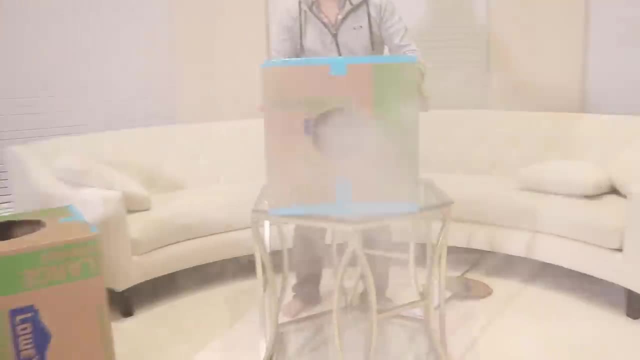 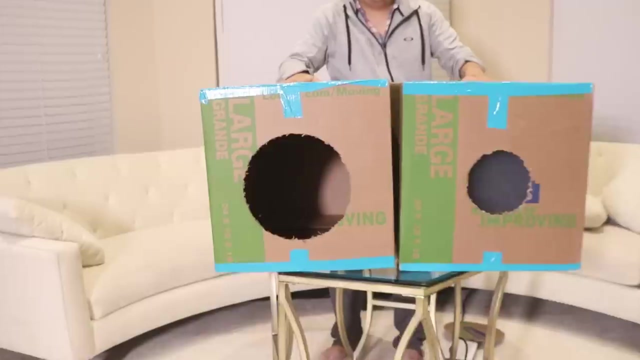 Uh, Uh, What's it? think That is awesome, possum. Oh, it's like the air. Okay, Ryan, after this fun science experiment, which hole produces the stronger vortex? This one, Yeah, Yeah, That's right. 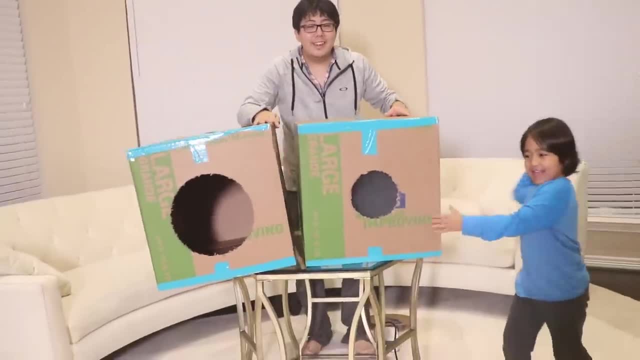 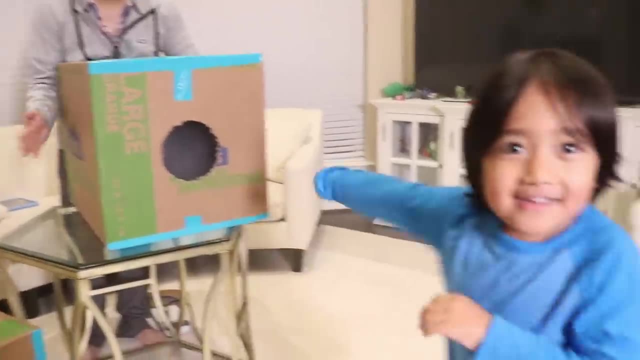 Smaller hole. It's smaller, so it's more concentrated. It still come out, huh Yeah, there's still some in there. This experiment is best done outdoors because we don't want to trigger the alarm system, But we have ours turned off, so it's fine. 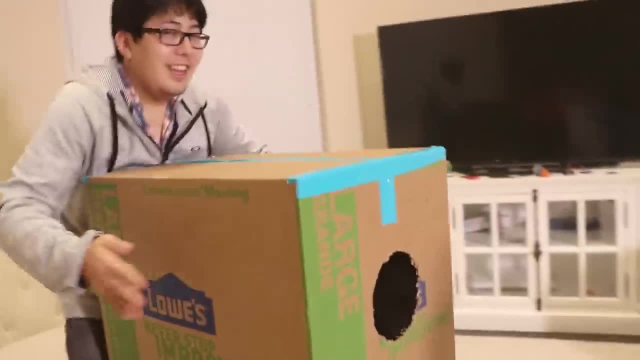 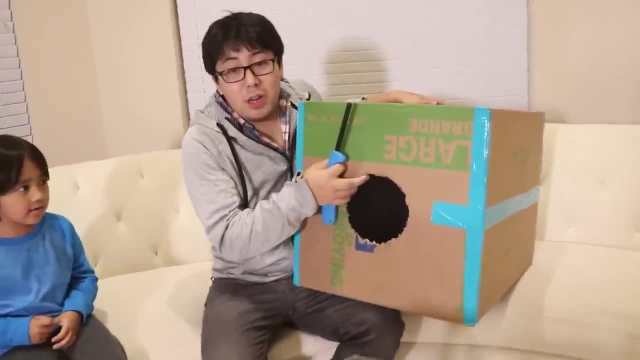 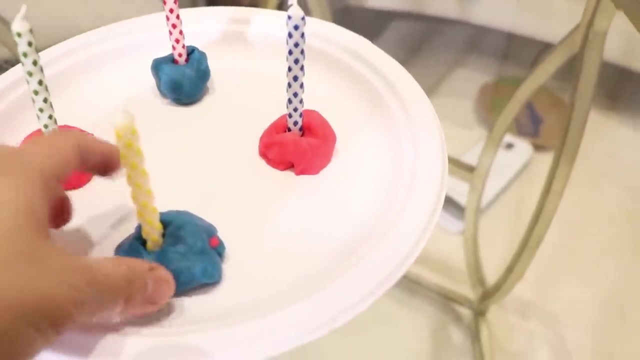 You got a jam to it, Daddy. Now we're going to use air bazooka we made to see if we can put up the fire on the candle. This is just birthday candle that we used, and then we just used Play-Doh to make it stand. 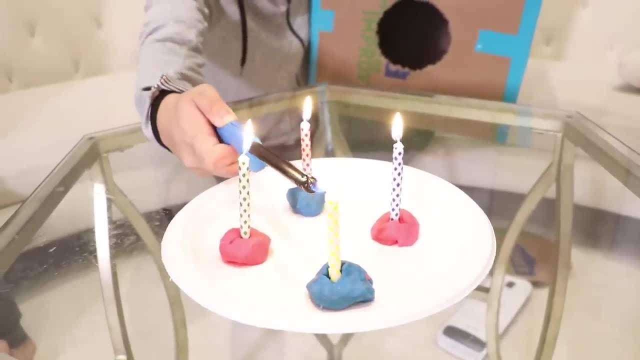 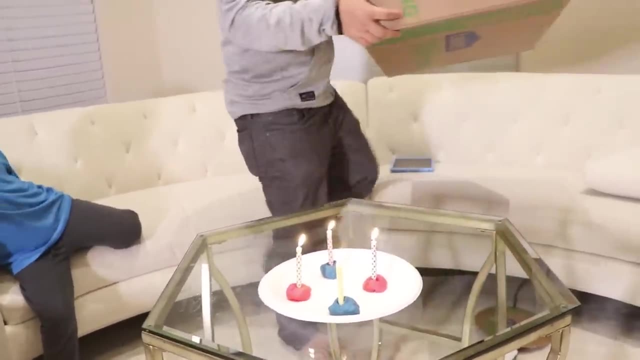 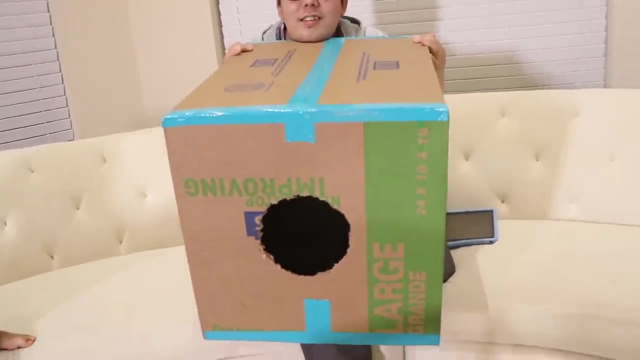 All right, let's light it up. Happy birthday to somebody. Happy birthday to nobody. Everybody. if today's your birthday, happy birthday. Okay, guys, before we start, do you think this air bazooka is strong enough to blow out the candles? 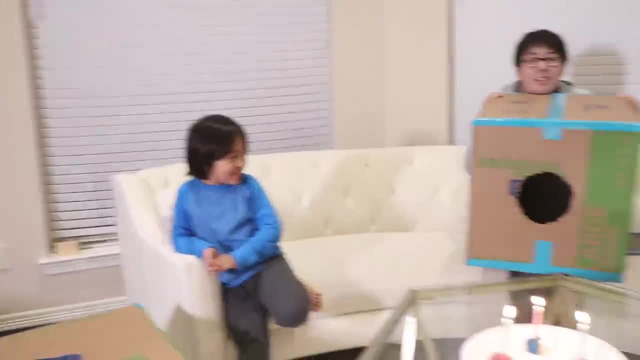 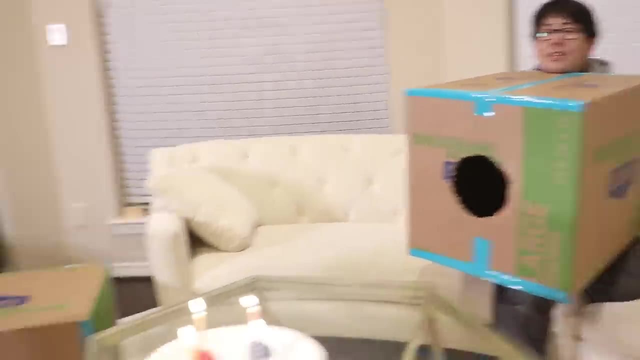 What do you think, Ryan? Yes, Yes, Yes, Okay. What do you guys think at home? Oh, the small one, Yeah, So the small one. we already experiment that it's stronger, right? Yep, All right, let's see, Daddy. 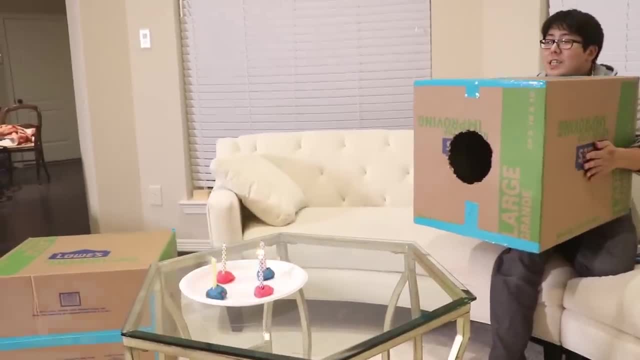 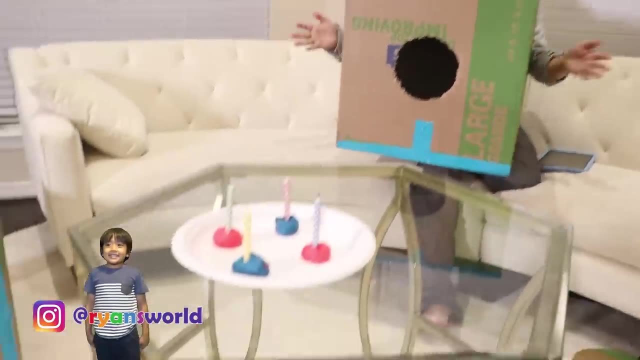 You guys ready? Yes, I'm ready. All right, Whoa, It blew out, except for one. Ah, you did it, Daddy. it worked. Yay, Yay, it worked, Yeah, it worked, Yay. 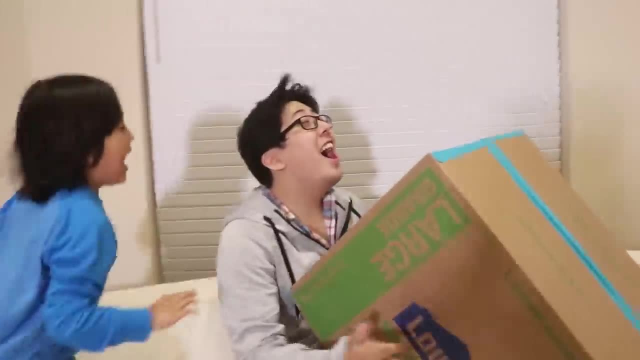 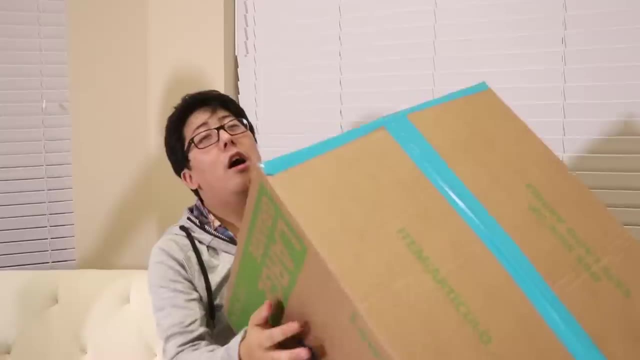 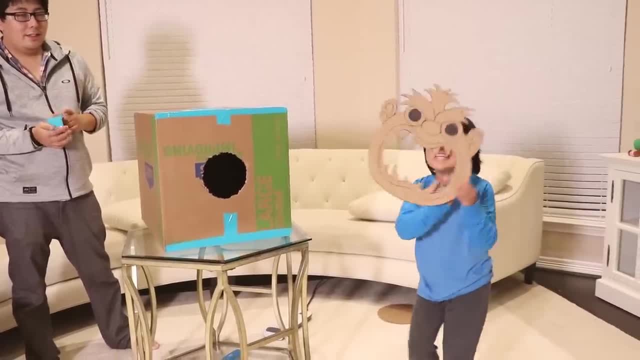 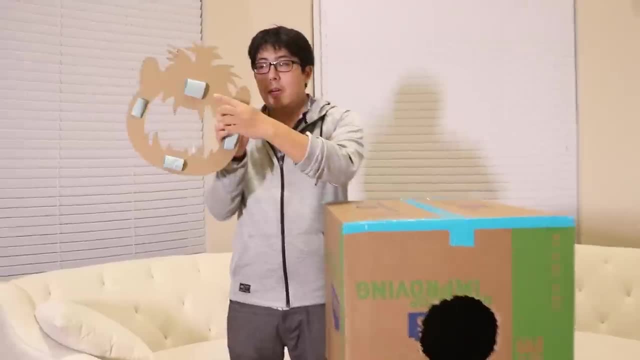 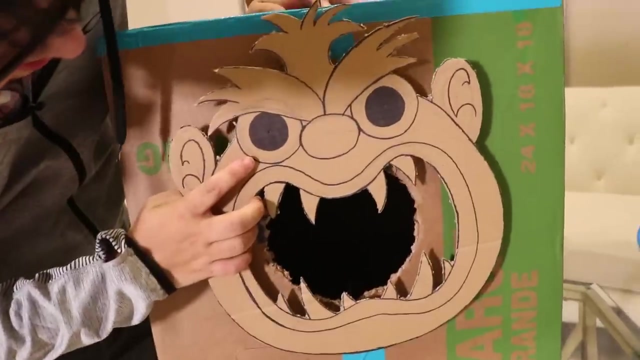 You can decorate your bazooka with faces. Whoa, That's funny. Look at him. he looks angry. Graaaaw, Put the duct tape on Boo, Angry daddy, Is he scary? He looks funny, scary, Funny, scary. 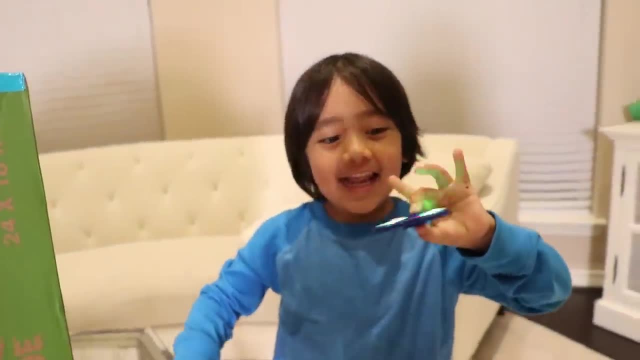 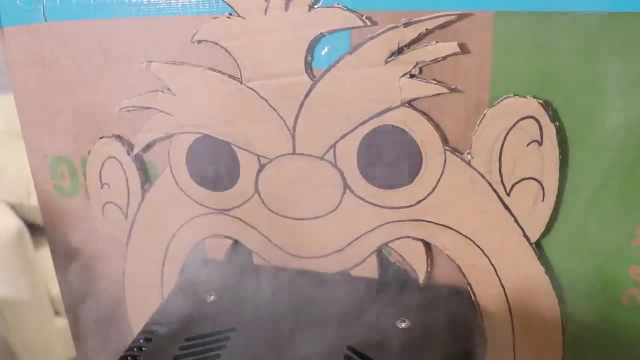 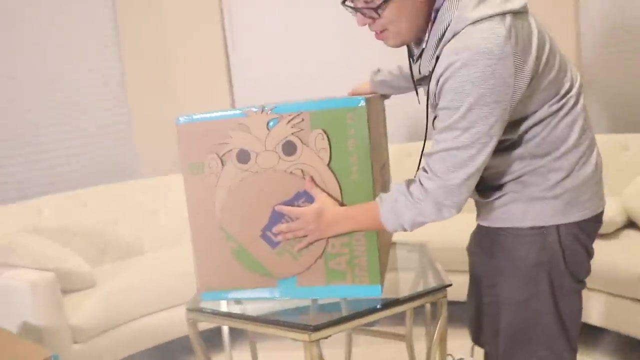 Ryan has a fidget spinner for some reason. Yay, fidget spinner. Yay, Still fun to do Smoke inside of the monster's mouth. He's eating the smoke. right now He's eating pizza. Let's test it. 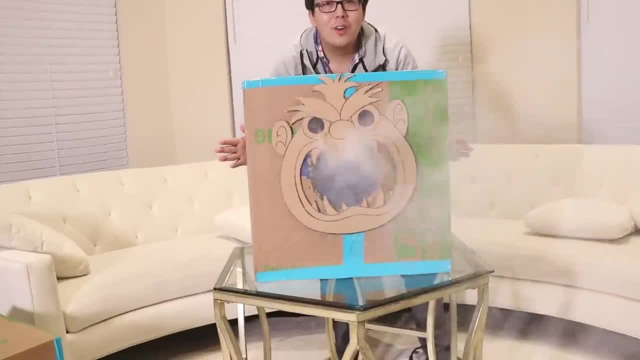 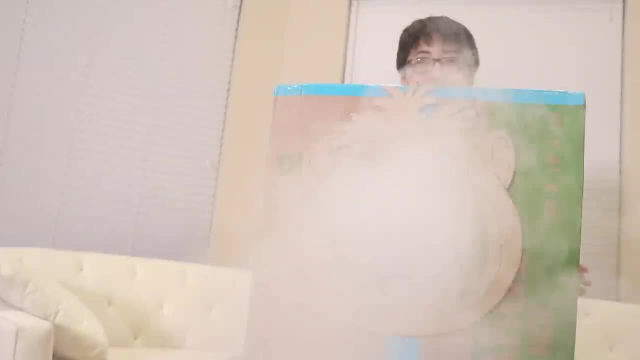 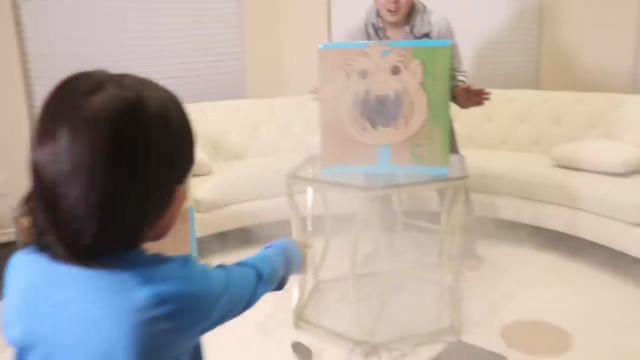 Are you guys ready? Yes Whoa, That's a small one, It looks so cool. Want him for the big one, Strong one. Yeah Whoa, Oh my god, Oh my, it broke that thing. Are you cutting it in half? 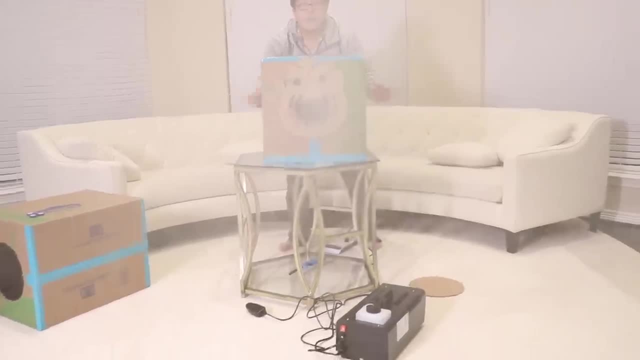 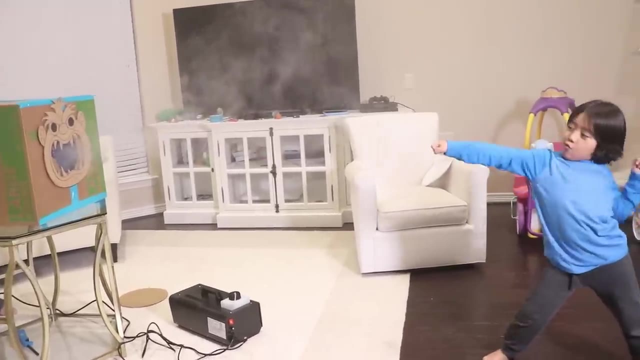 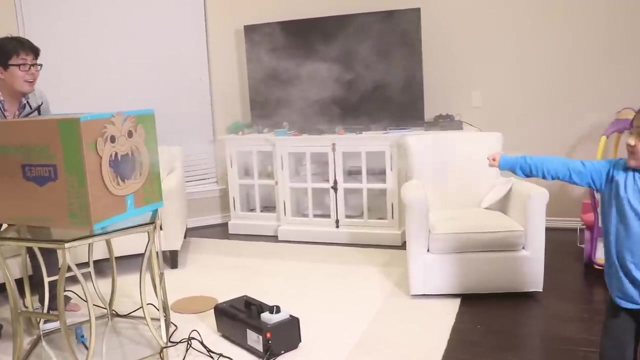 Oh, Whoa, Whoa. So cool He's punching the ring. I'll do a double ring. Okay, Whoa, yeah, you see the double ring. Wow, See, if you can do three, Am I doing it. 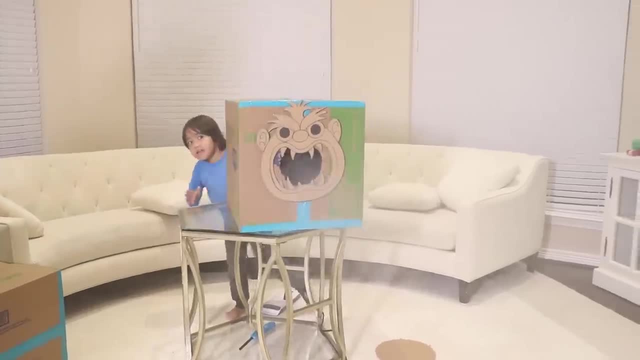 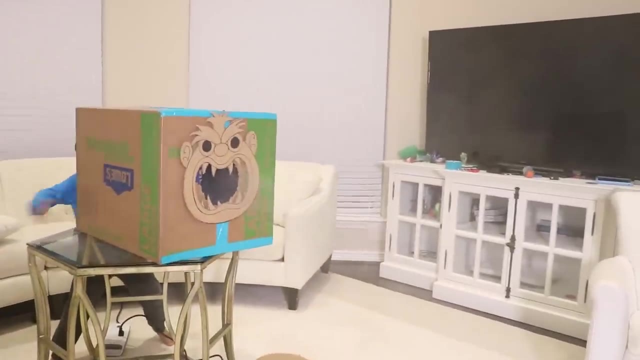 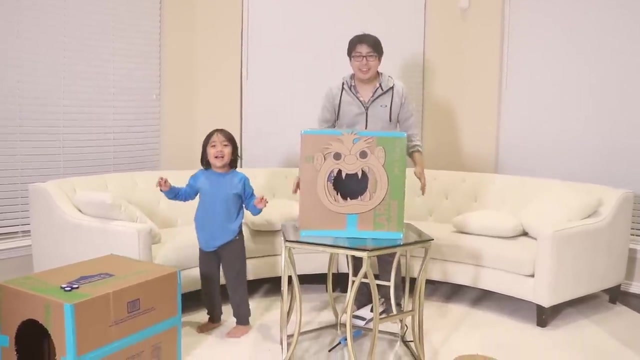 Yeah, Cool, Am I doing it? Yeah, yeah, Yours is coming out. Yours is coming out good, Yay, Thank you for watching our giant bazooka video. Bye, Bye, everybody, And if you guys do it at home, let us know. 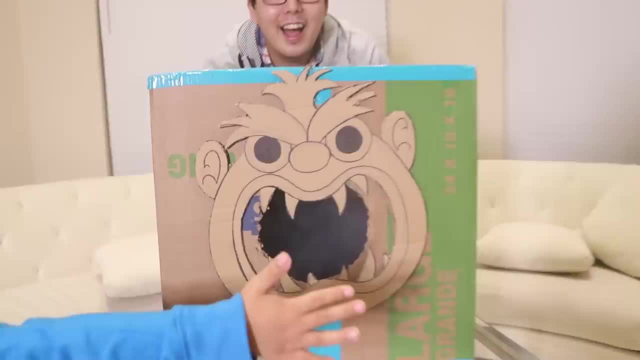 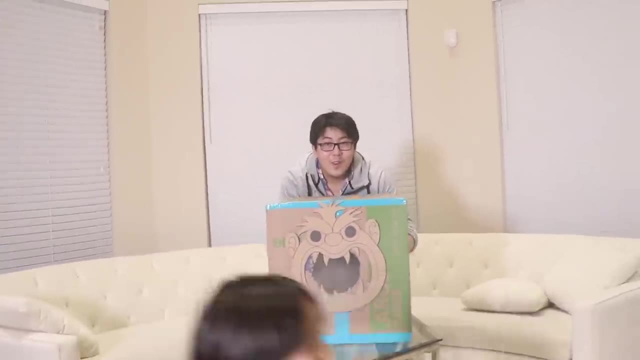 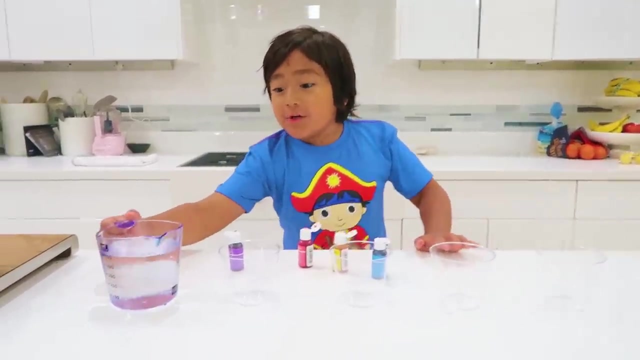 And if you do, do it, make even a smaller hole to see if it's even strong. And if you forgot happy birthday, Bye, Hi guys. Today we're doing a science experiment to learn about water. So first you pour the water inside the cups. 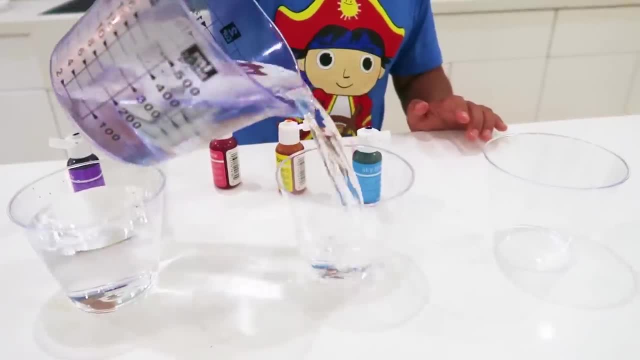 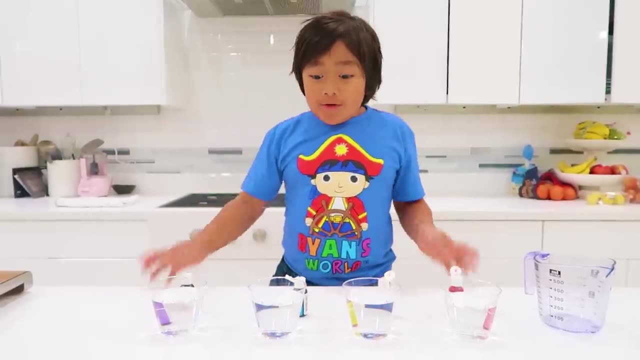 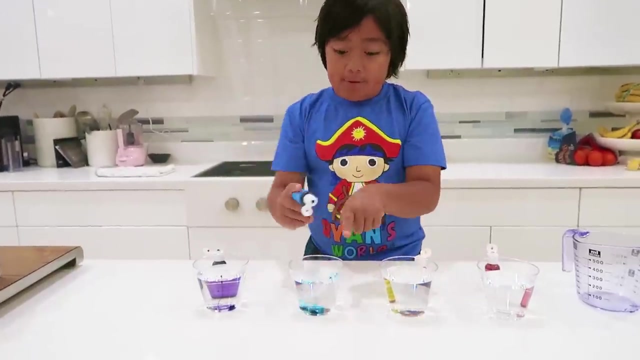 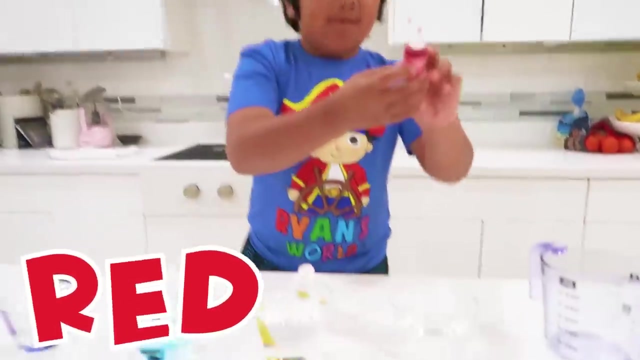 Like that, Like that. Okay, Now let's put one of the food coloring in each container. I put purple there And I put blue there, And I'm gonna put yellow right here And red Right here. Next, I'm gonna mix. 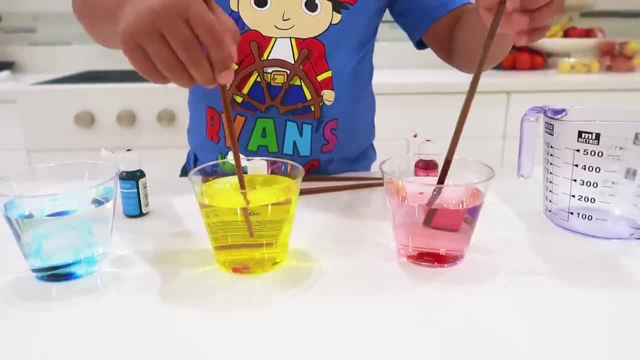 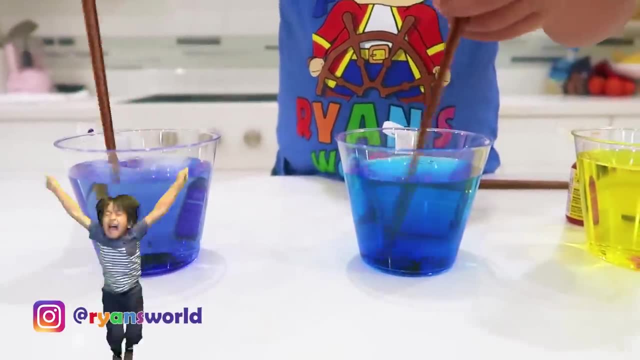 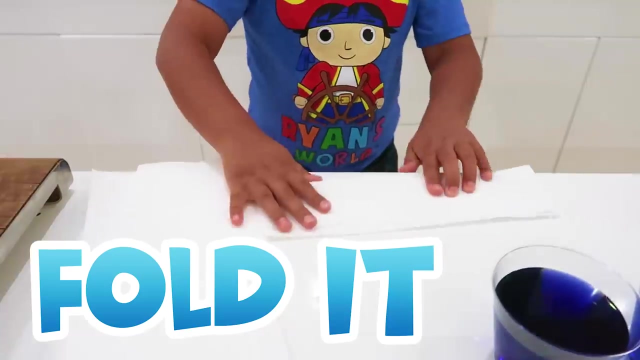 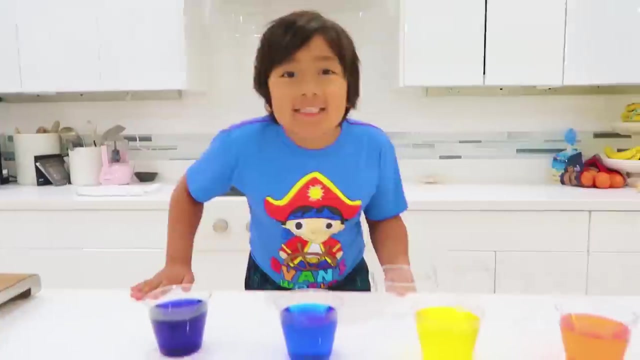 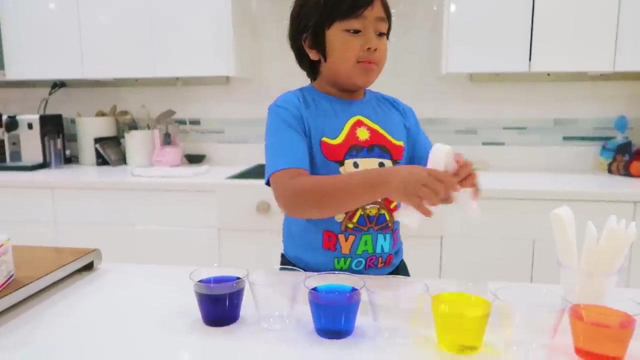 them together. Good, And now we're gonna fold some paper towels. So first you fold it, Second you fold it, And third you fold it Next up, put the empty cups in between, And now we use the paper towels. 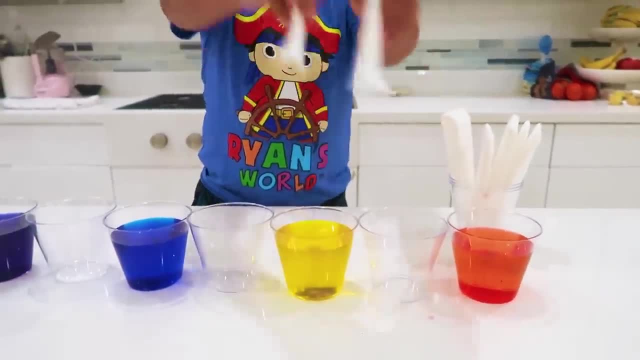 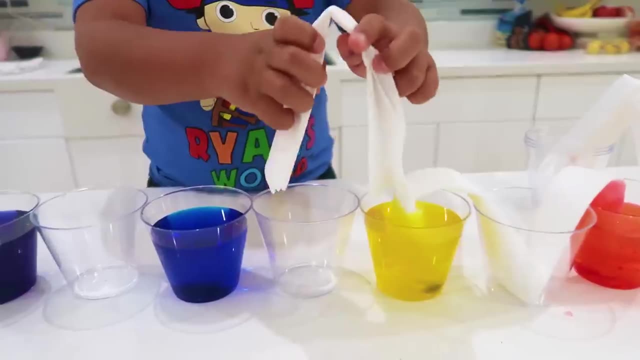 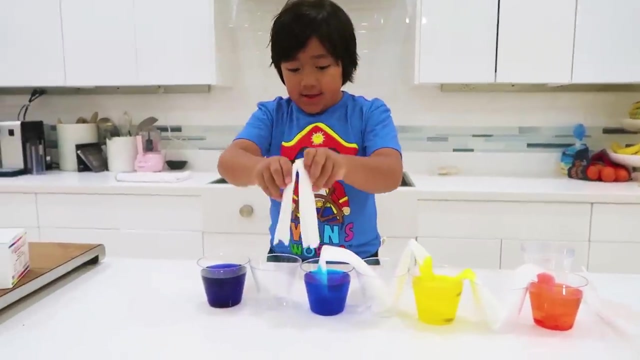 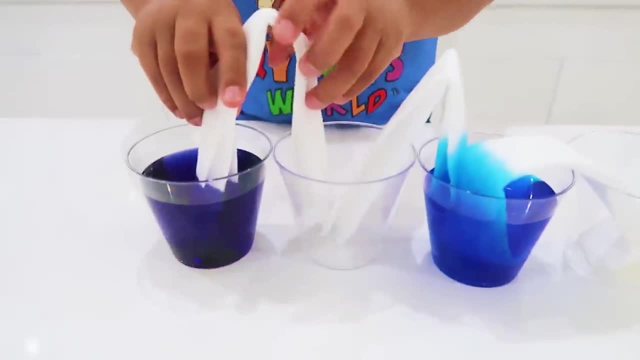 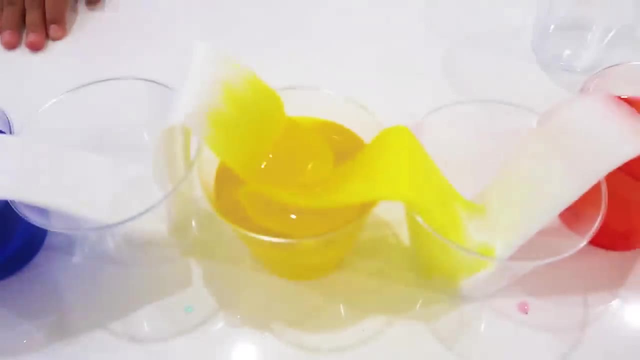 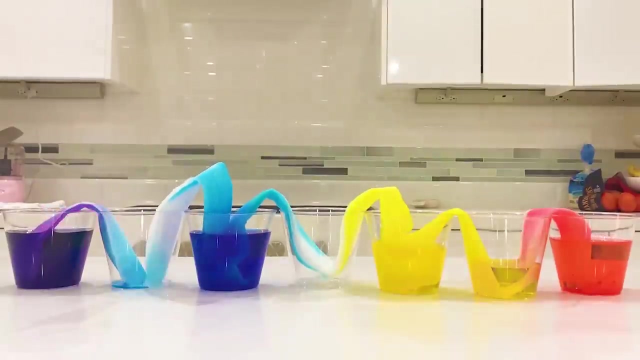 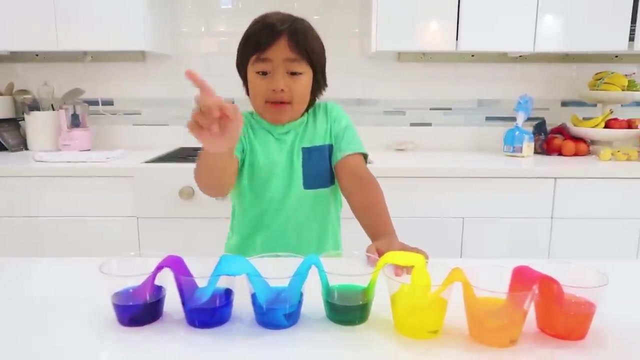 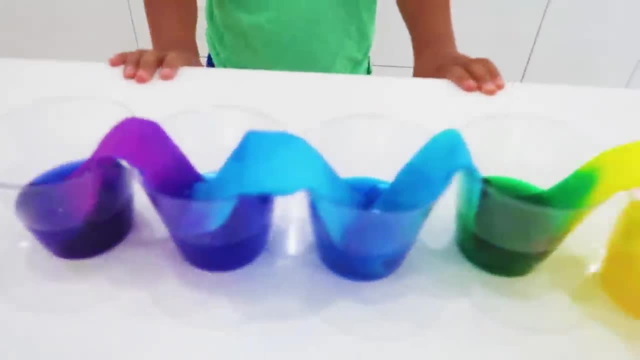 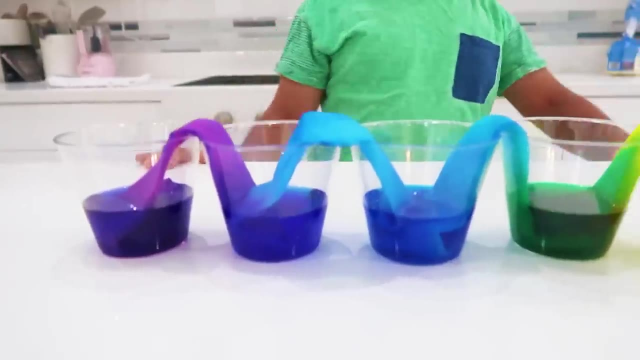 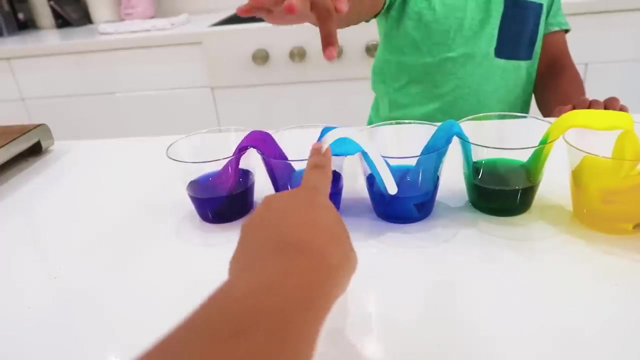 and went down and mixed the colors together. Look, And now the cups that were empty now has water. See what happened, Ryan. The water travels up and then over. And then this cup: the water travels up and then also over, right? 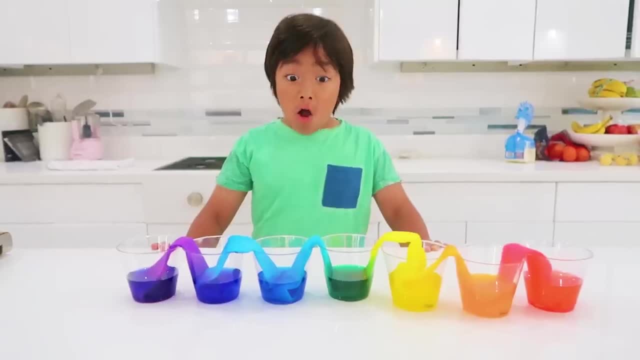 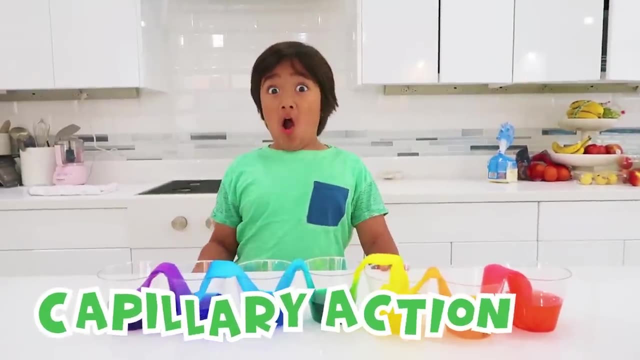 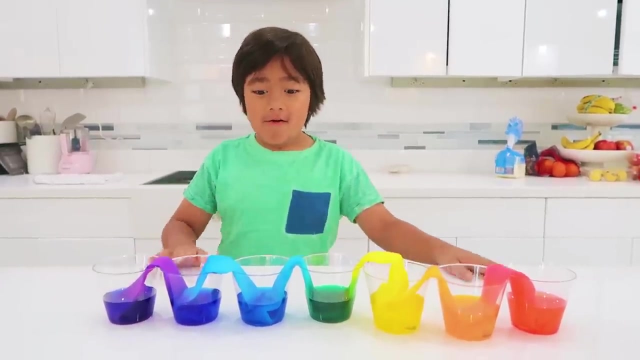 So how did the water travel up the paper towel? Here's how it happened: The water color travels up the paper towel by this thing called capillary action. So do you remember how plants, where does the plants get the water from? Yeah, underground, That's right from the roots. 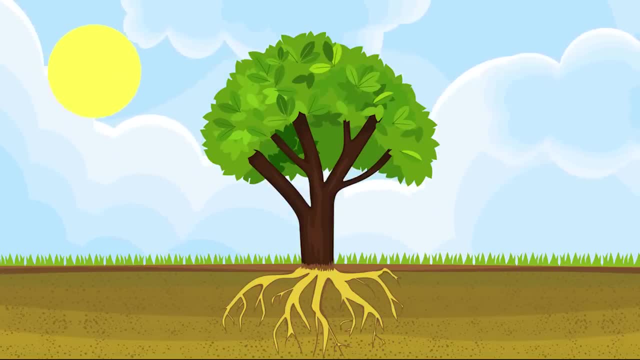 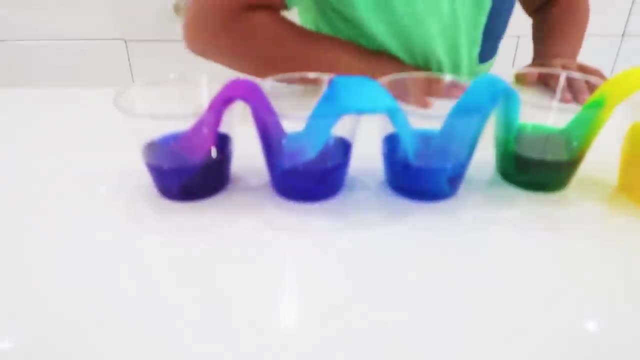 So the plants get water from the roots but it has to travel up the plants so against gravity. So it takes the water from the ground and travel it up, just like how the paper towel takes the water from the bottom and it travels up. 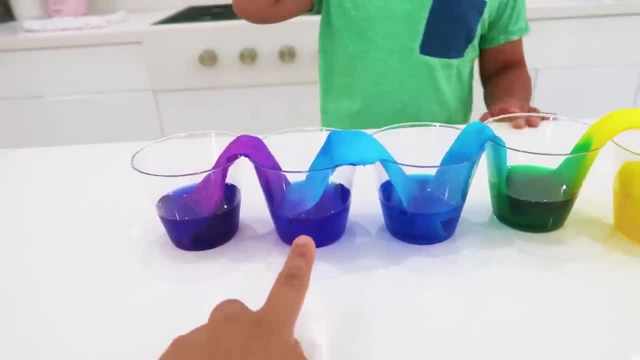 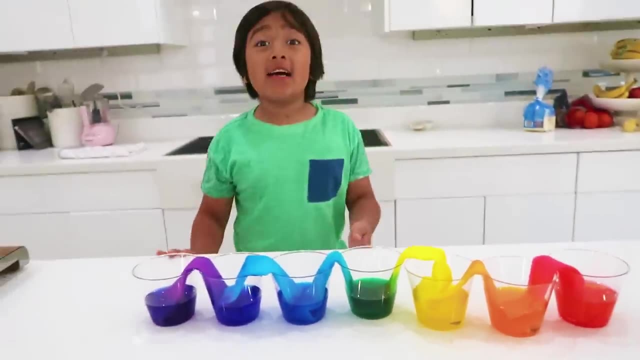 Now you see how the empty cup changes colors. Yeah, Okay. so here you have blue with yellow. When you mix blue and yellow together, what did you get? I got green, That's right. And here you have yellow mixed with red. What do you get? 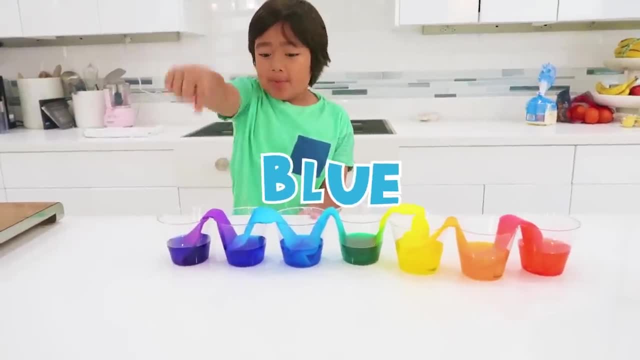 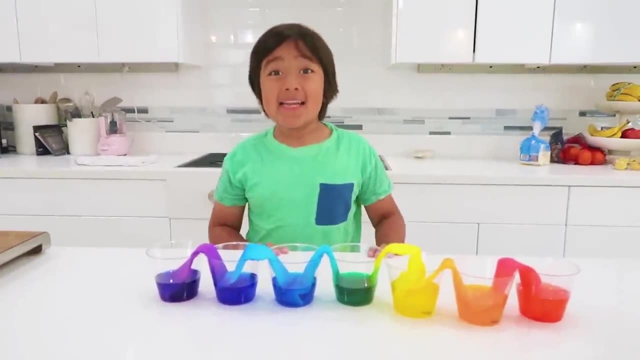 Orange, Orange, yeah, And blue and purple is like a galaxy color. That's right, yeah. That's what happens when you mix it together. That's so cool, right, Yeah? Now let's take out the paper towels and see what it looks like. 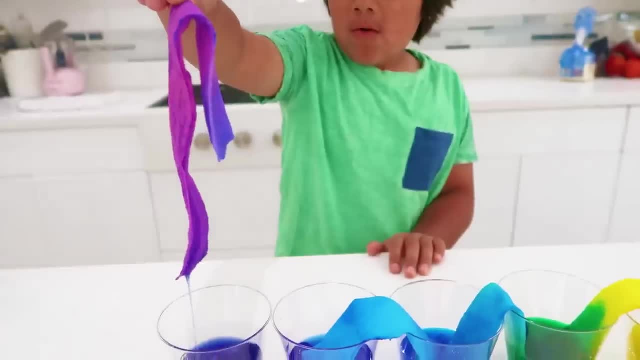 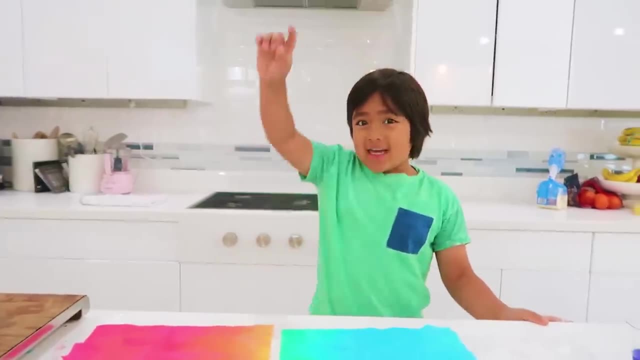 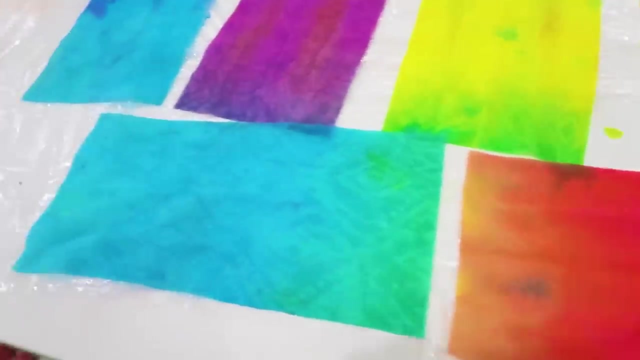 Cool. And Here's what it looks like when we take out the paper towels. Look at all the colors. It looks like a tie-dye t-shirt. Yeah, Wow, you guys see, It looks really, really cool. And look what happened. 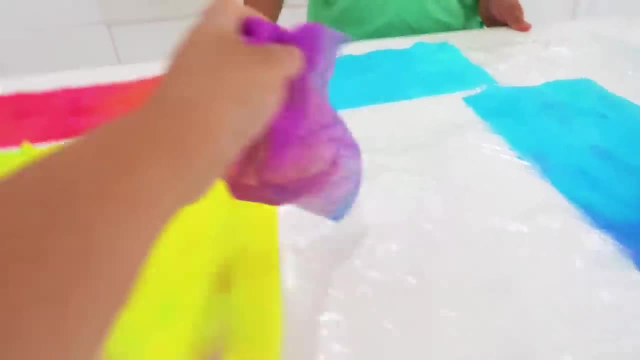 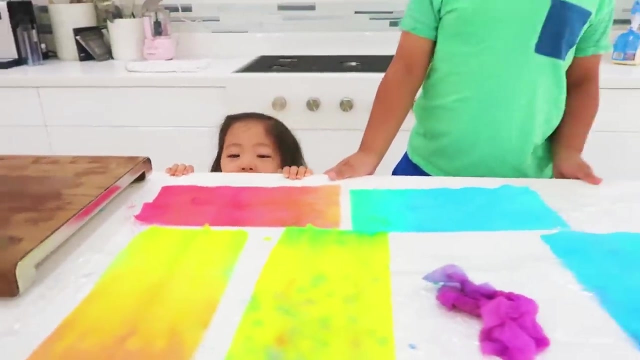 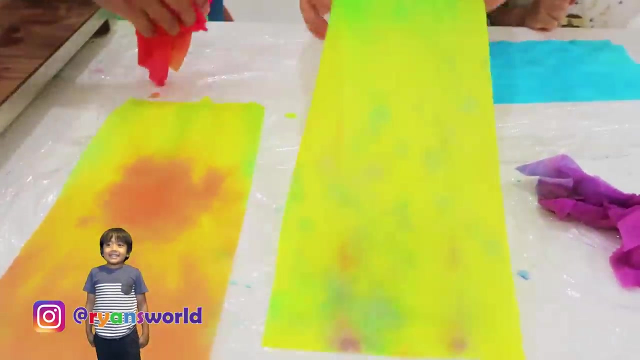 Look, you can make even more color. You can get this one And then, Aww, You want to make it too. Yeah, Yeah, come, I'm going to show you, Take it and you squeeze. Oh, you see how it makes color. 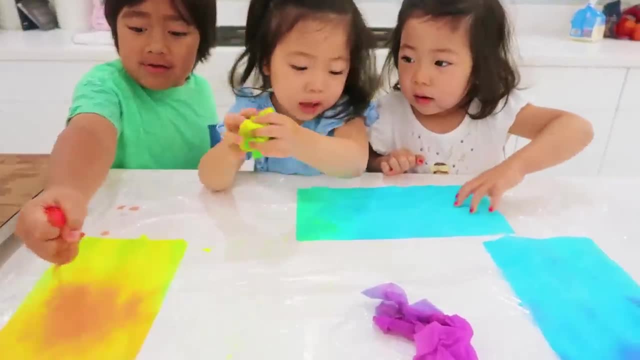 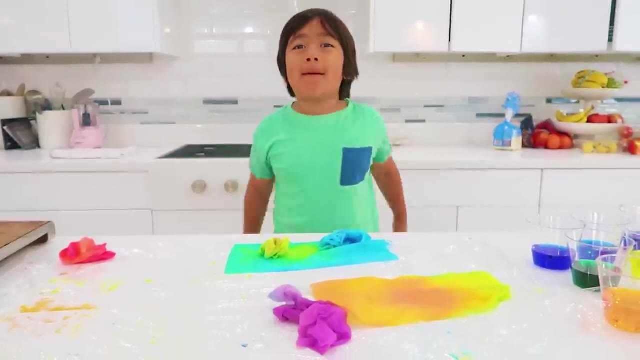 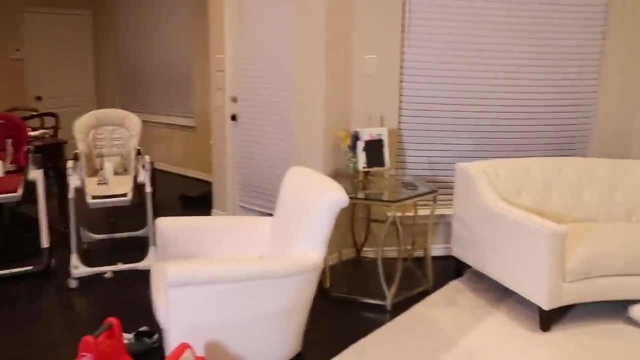 Yeah, Oh, this one actually don't move. There you go, guys. Thank you for watching my science experiment. Bye, Remember, always stay happy and rise up. Bye, Mommy Ryan, Where are you? Hi, everybody. 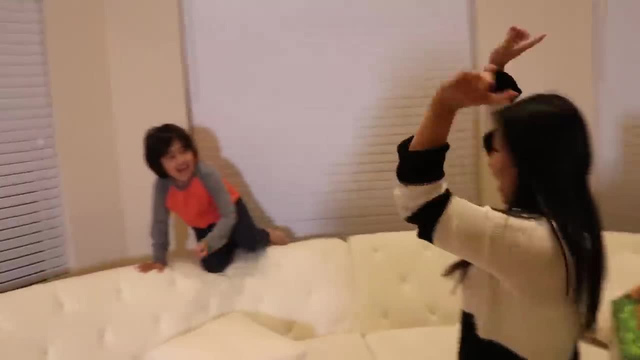 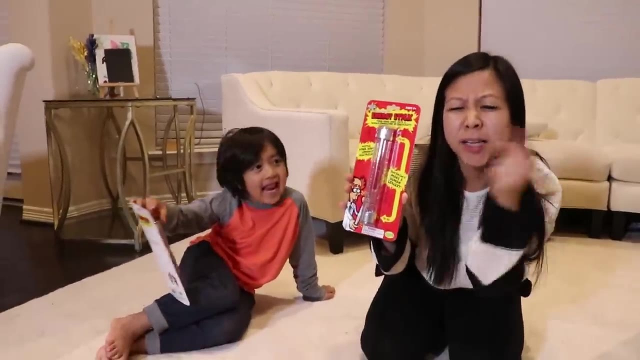 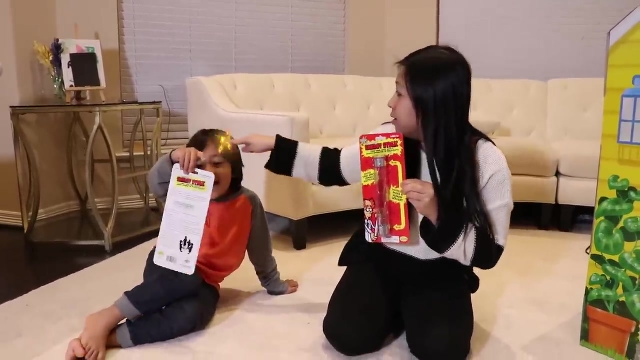 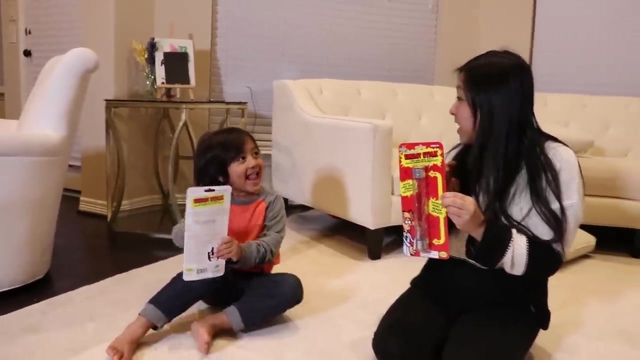 It is Mommy and Ryan. Today we have this cool, awesome energy stick here and it says: turn your body into a human conductor of electricity. It says: watch your body conduct electricity. Isn't that cool? So inside this stick here I'm going to open it up. 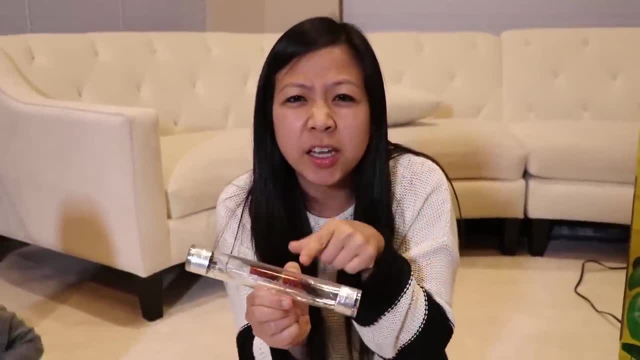 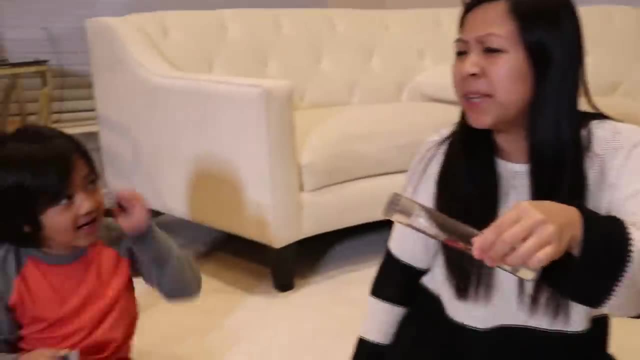 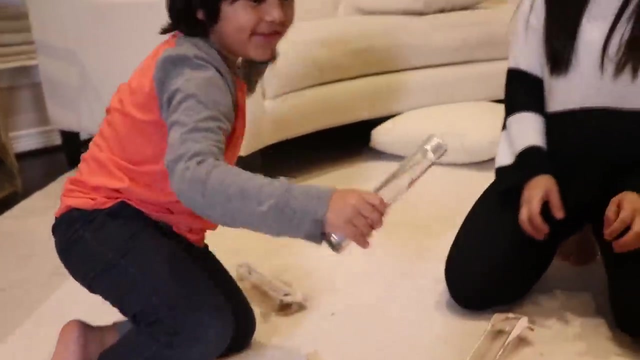 so you guys can see Inside. the stick here has a circuit, It also has batteries and it also has some LCD light. What is missing is for us to complete the circuit. How do we complete the circuit Here? you try, Yeah, so we connect. 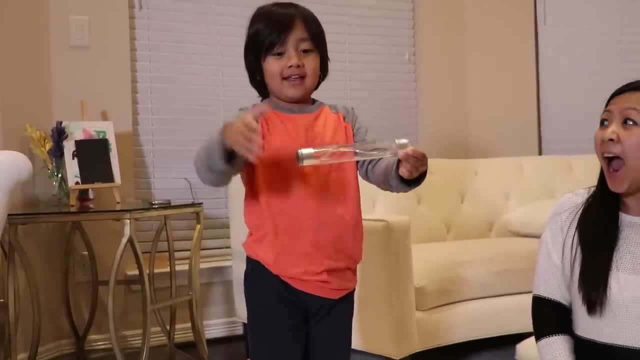 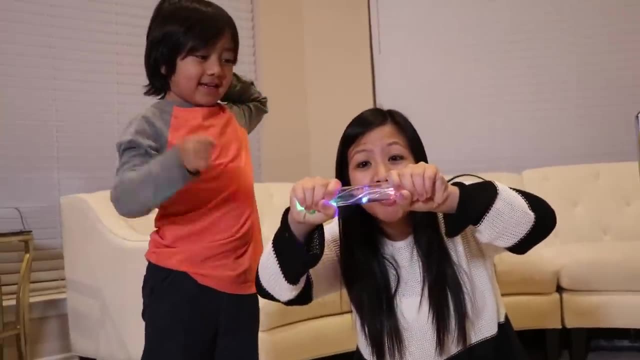 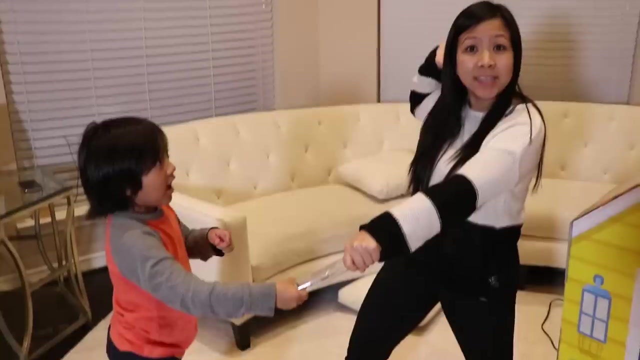 and complete the circuit. Yeah, so when you let go, it stops, and then when you put it on, you complete the circuit and then it lights up. Now you think we can do it with two people. So Ryan won, Mommy won. 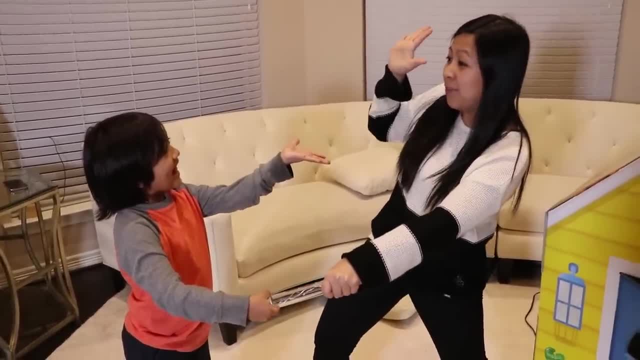 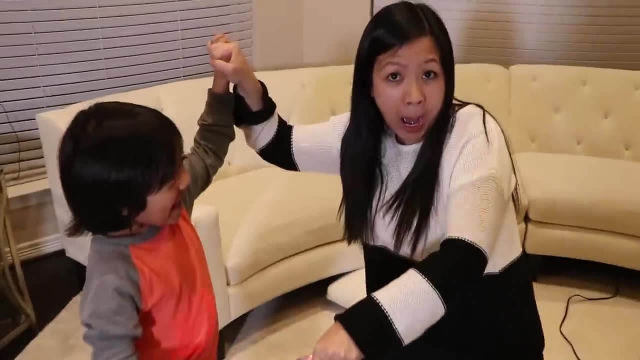 It doesn't light up. but how do we light it up? Let's high five, Ready High five. Did you guys see Open clap, Whoa, It's cool. Yeah, Don't clap, Ryan, I just go. 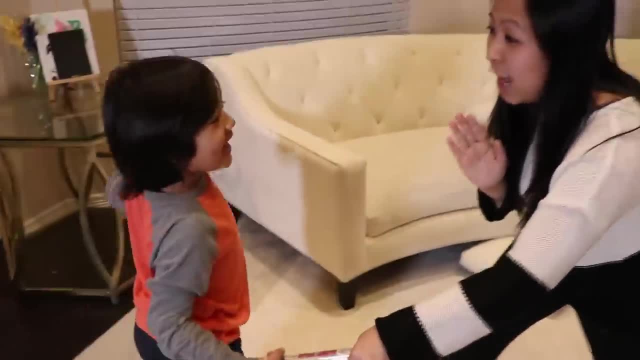 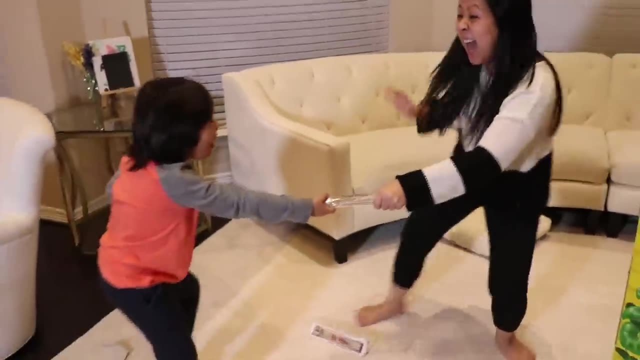 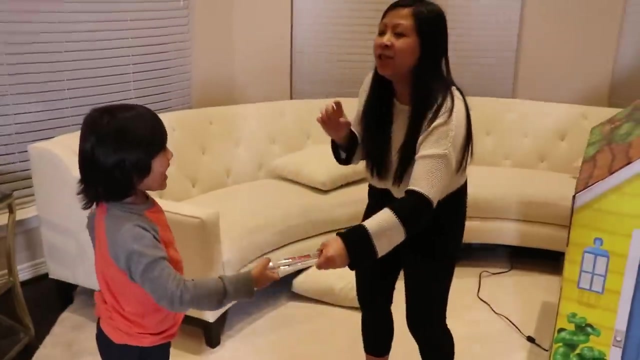 It's working, Ryan's cheek working, Yes, Oh, and you know what else works? How about we touch feet instead? Are you ready? Let's try again. You ready? What about by saying jingle bell? You guys want to work by saying jingle bell? 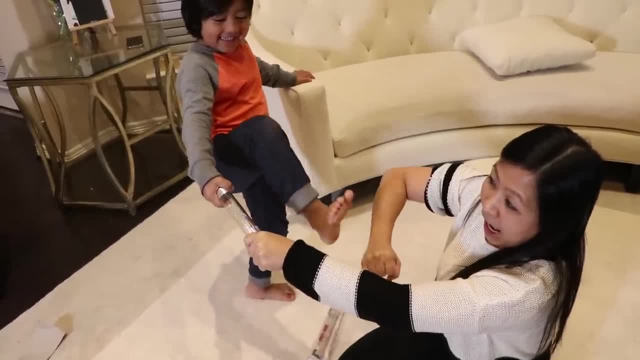 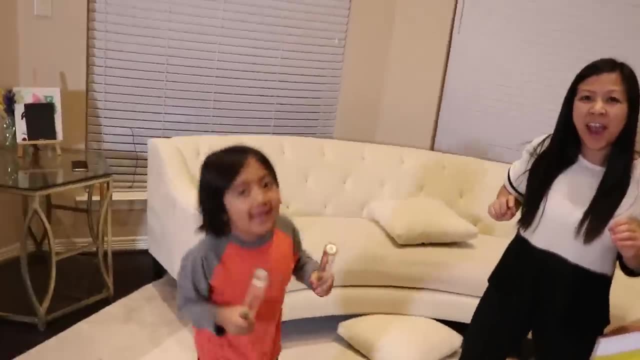 No, Let's see You ready. Jingle bell, jingle bell, jingle bell. Nice, So how about we make it work with two? Do you think we can make two work? Hold still, so Mommy can hold. 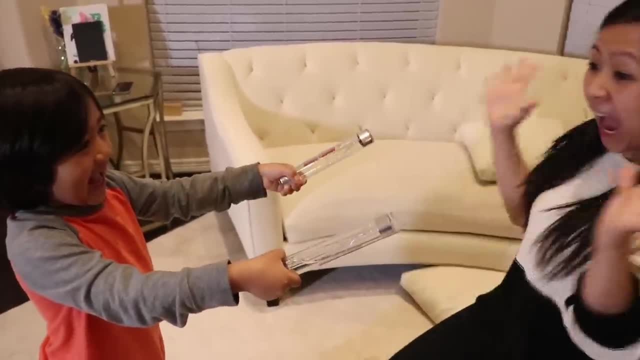 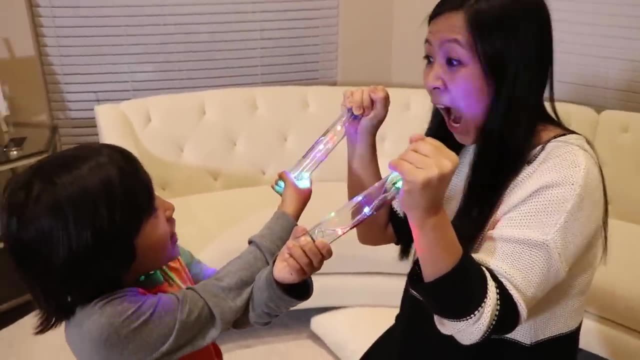 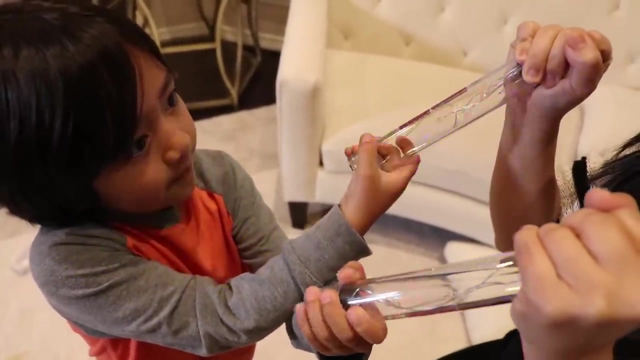 Yeah, We're gonna try crossing your hand. Oh, it still works. It only works if both of these are together. Yeah, because you have to complete the circuit. There you go, you have to close the circuit. Okay, so we're going to try stick. 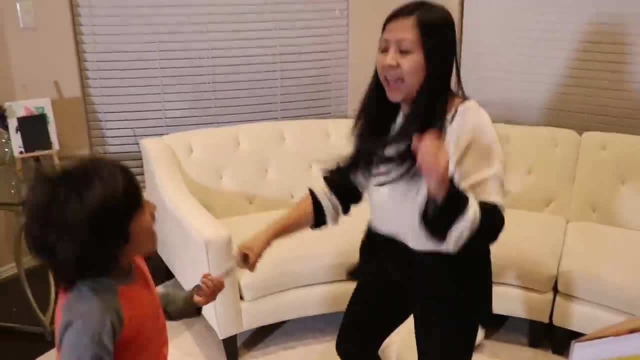 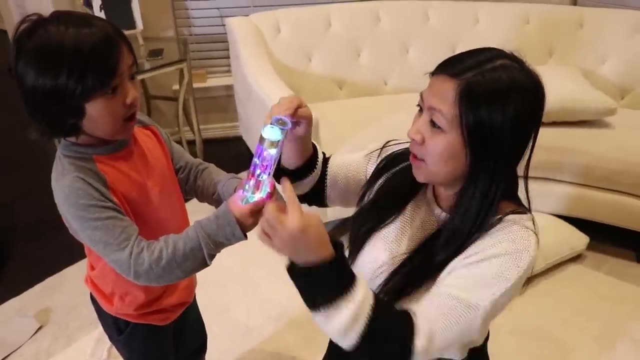 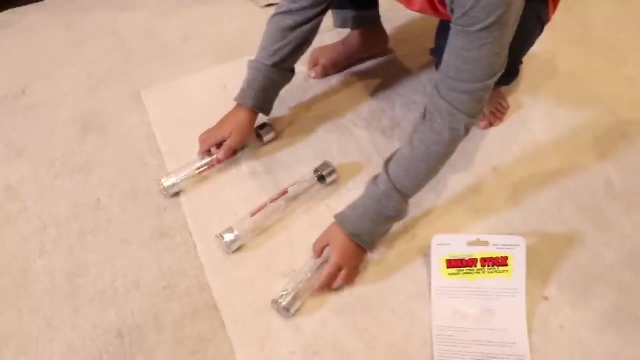 two feet. Let's see, Yay, it worked. Yay, Okay, now what about we try with three sticks? Wait, how is this working? Because they're connecting. Now the electricity goes there. Okay, guys, we're gonna try three-stick challenge. 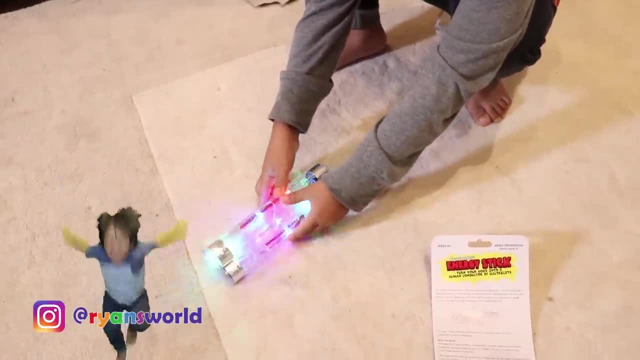 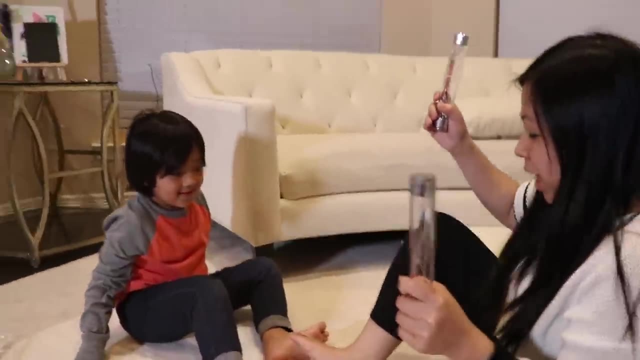 Whoa, Whoa, She put the flash in there. Oh, it worked like that too Cool. All right, Ryan, a three-circuit challenge. All right, you ready? Yes, Did you see, Daddy? Wow, that's cool. 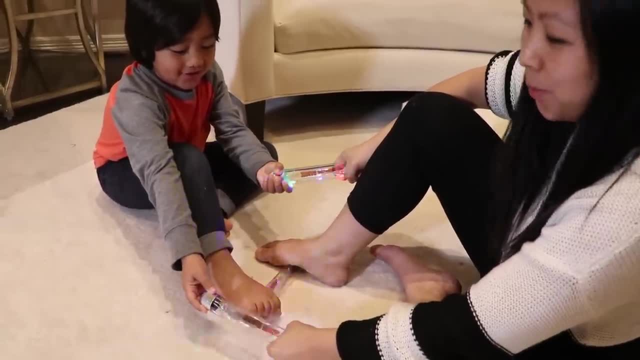 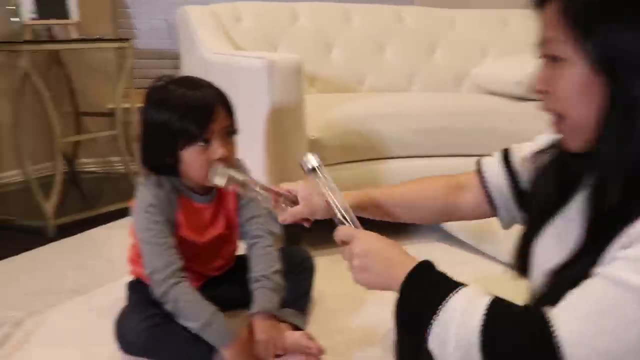 Look, if you let go, none of them work. And when Ryan touched, all three of them worked. Wow, that's so cool. I have another idea. So your body conducts electricity because you have water inside, and water conducts electricity. 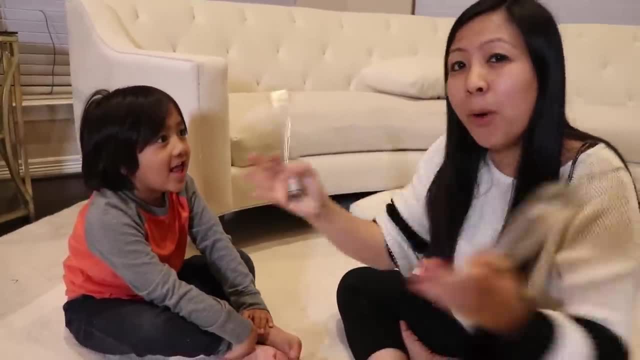 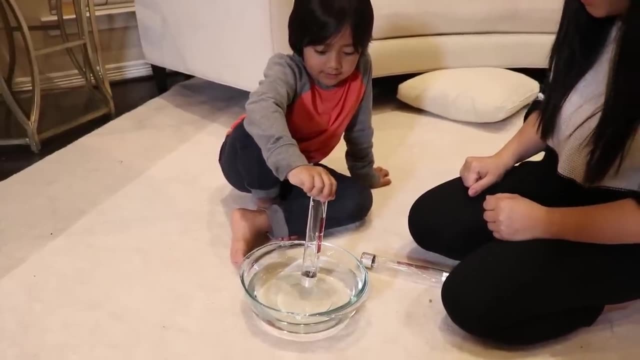 Now what if we don't touch each other and we use a bowl of water? Oh, You think that will work? Yeah, Let's test it out. So you put one end in. There you go. okay, There you go. 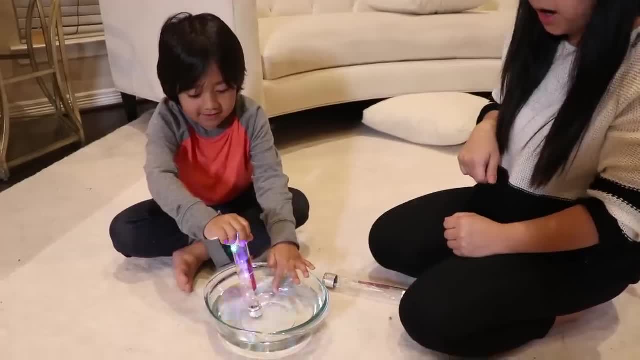 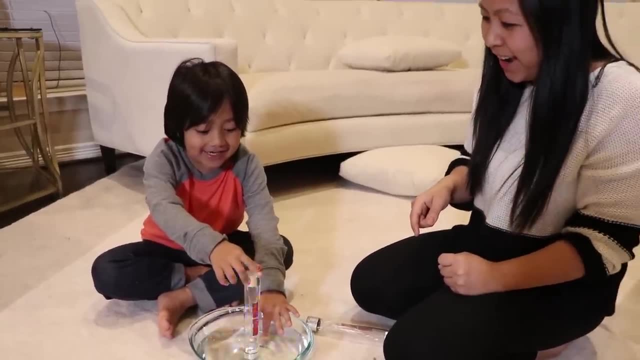 And put the other hand and then just put your other hand in. All right, it works. That's so cool. Do you feel the electricity? Oh yeah, I do. I do You do Okay. okay now, Pete, now. 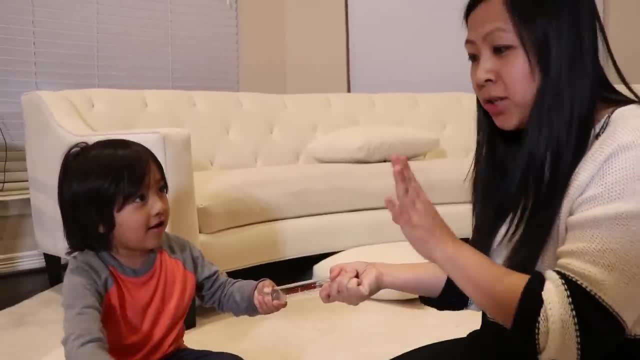 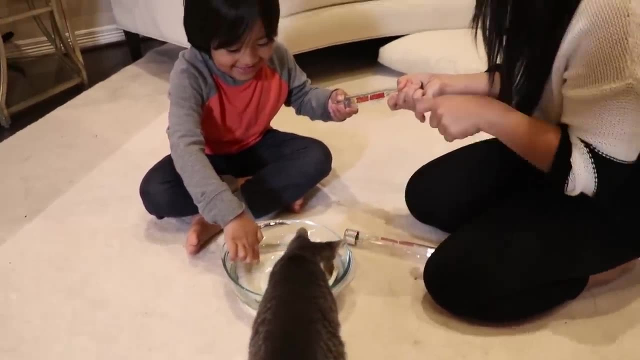 let's try with two people Now. we each put our hand in, but don't touch each other. You go first. Oh, the cats, That's not drinking water. That's not drinking water. We're doing a science experiment. 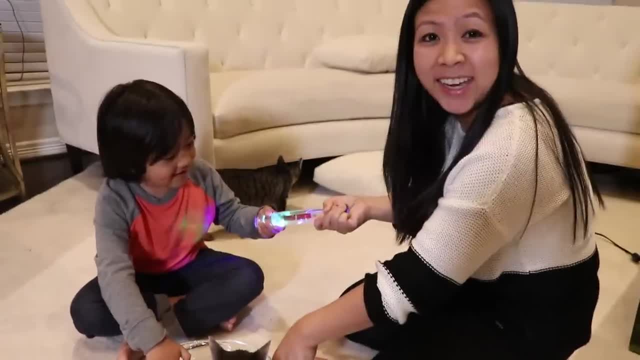 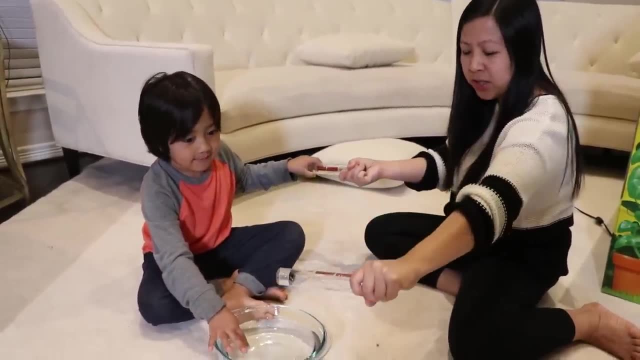 Whoa. Oh, look Look at that, Our hand's not even touching. That's so cool, Isn't that cool? Look you guys. All right, let's see if we can complete the circuit without touching each other, and the water will. 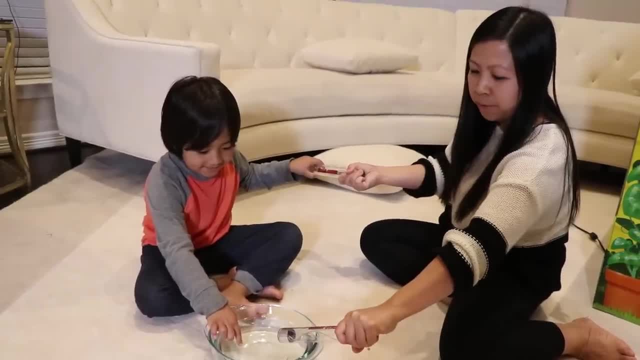 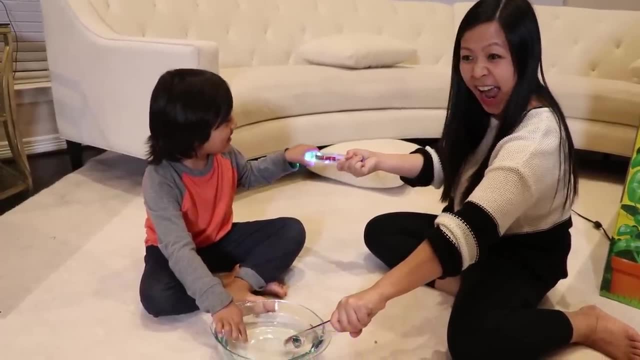 Oh, so I use it from that, Yeah, and the water will complete the circuit for us. Let's see dipping it in, I feel. I feel the electricity. Do you Boop, boop? Try with three, Ryan, you hold one too. 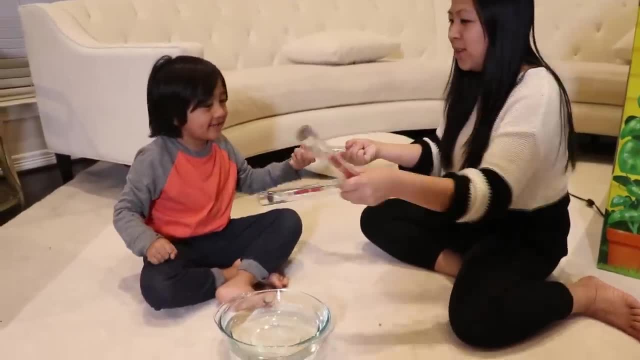 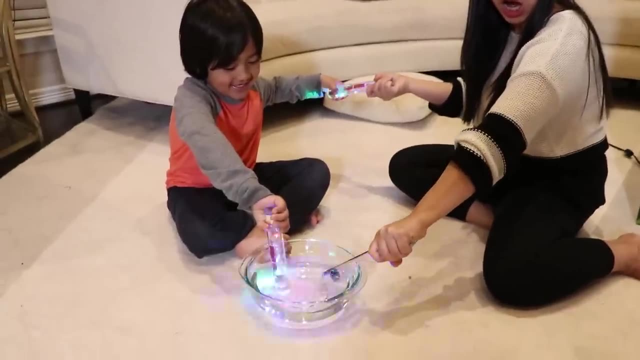 Oh yeah, Oh yeah, Okay. so we each hold this one and you hold that one. Okay, you ready, Ready, go. So one doesn't work. Let's see if I can complete the circuit. Oh, three of them. 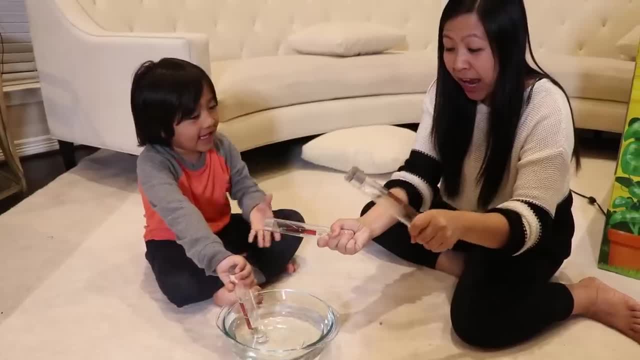 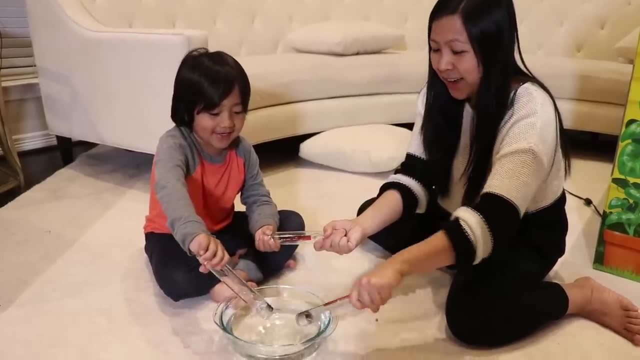 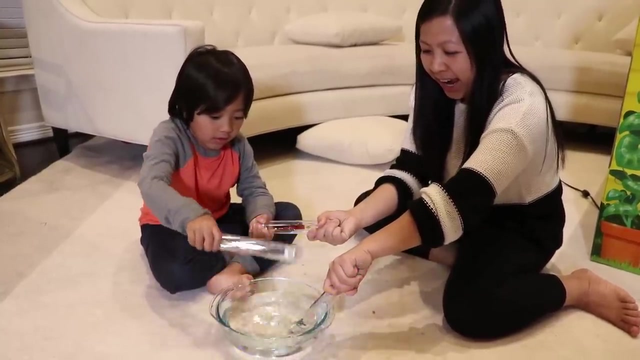 Look at this. It'll let go. It doesn't work, I'll put it in: Wait, let me do two. Okay, go ahead, You do it. Wait. oh, Yay, All right, Let's try it with Daddy. 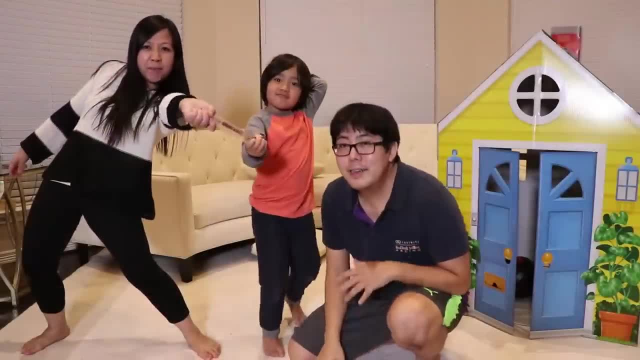 All right, I'm ready. I'm ready, Let's do it. let's do it. So, Ryan and Mommy- right now we're missing Daddy- to complete the circuit. Okay, ready to complete the circuit? Uh-huh. 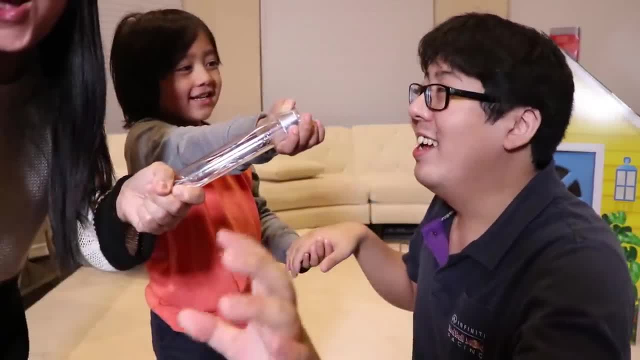 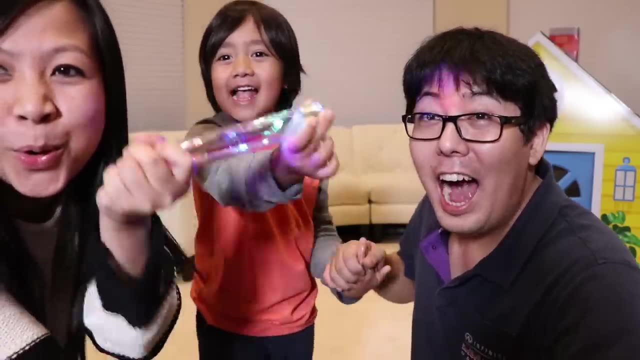 Whoop, Ah, All right, let go. Ah, Oh sorry, sorry, Ready, Ah. Ah. Oh, Just kidding it did. We don't feel anything. Woo-hoo, It's completely safe, and fun, That's cool. 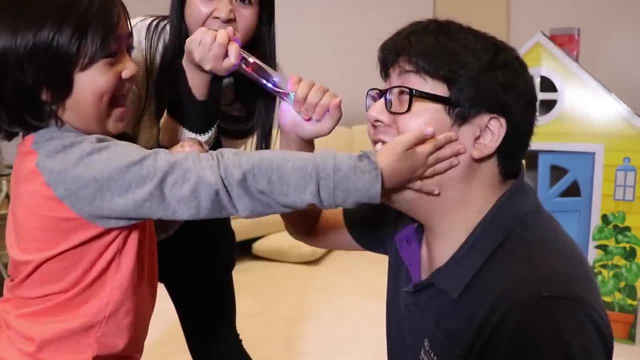 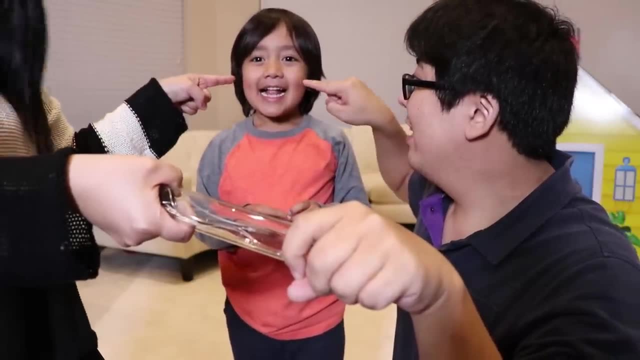 All right, let's see. Ah, it's working. Ah, All right. so Mommy and Daddy gotta poke Ryan's cheek at the same time. Huh, It doesn't work. Oh there, it is it worked. There you go. 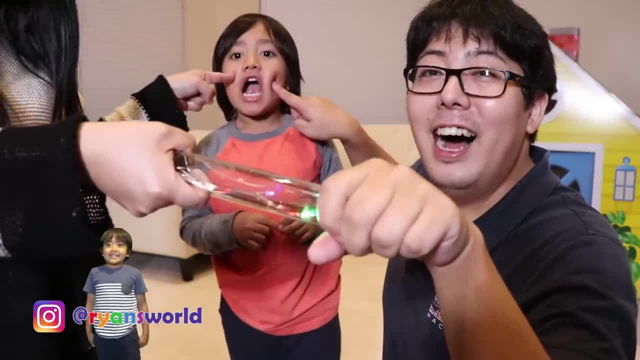 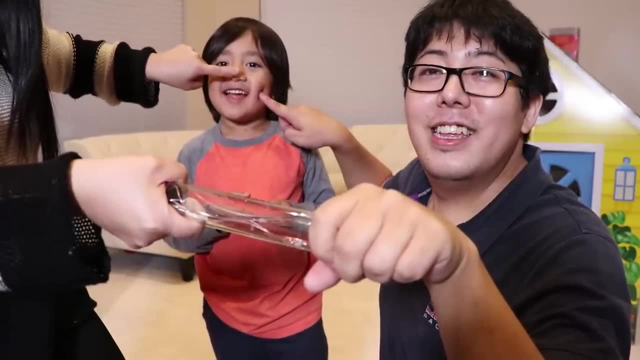 I let go. it doesn't work. Let's see, Whoop, Ah, it works. If you put it in the same spot, it doesn't work. What about your nose? Let's see, It works a little bit. All right, let's try with another energy stick. 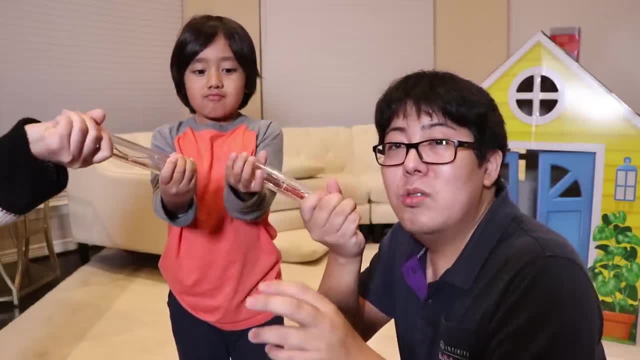 That's cool, Let's do it, let's do it, let's do it. All right, so we got two energy stick here. We got two. We're gonna hold some hands. Huh, Huh, Oh, no, no. 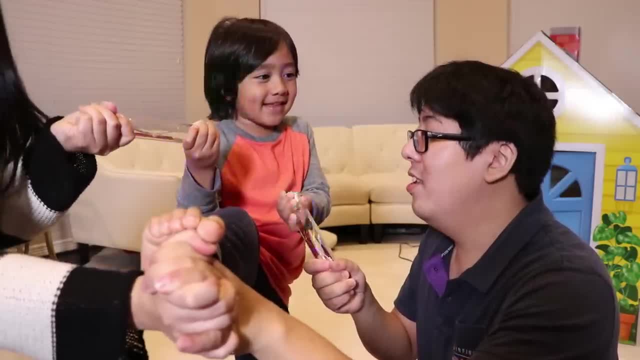 What Put my feet in? What Ryan had to put his feet in? He needs his feet. Okay, let go of your feet. Let's see what happens, What Makes more sense. Oh, I know why You have to flip it. 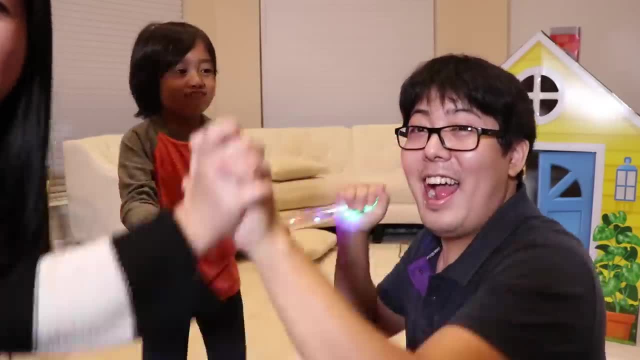 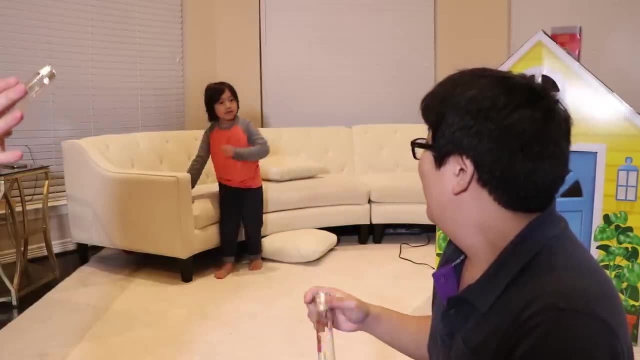 Whee, Yeah, because we flipped it, it works now, Yay. Energy circle, Oh, last one, Oh, complete, One more, Yeah, So each one of us have an energy stick Ready go. Yeah, Oh, it's working. 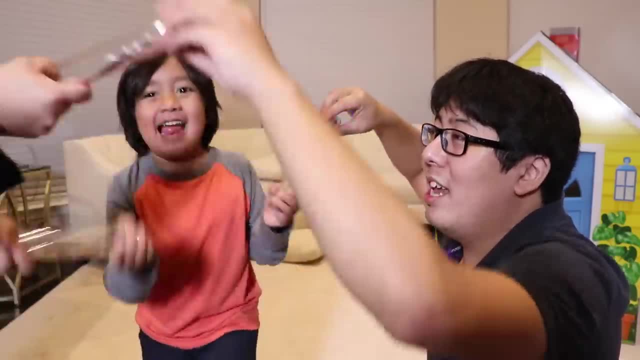 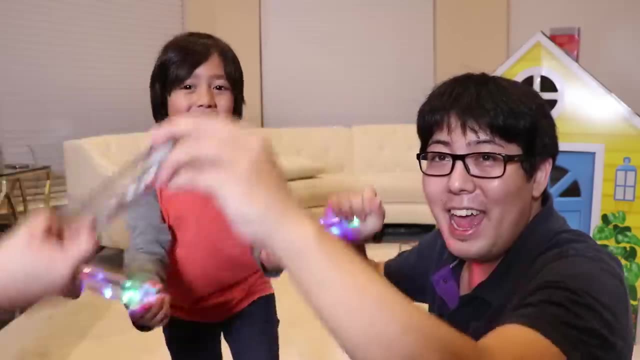 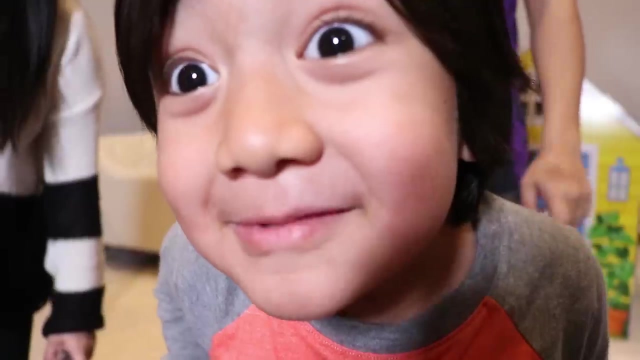 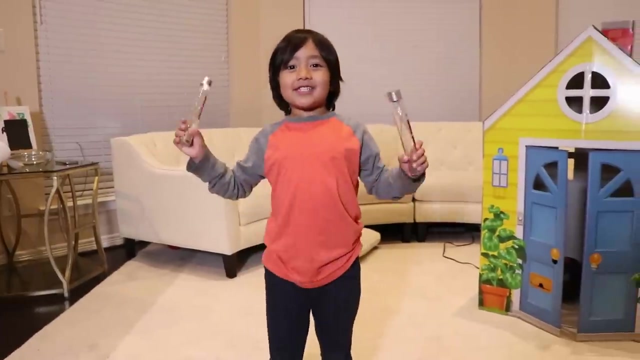 Yay, We're offering you energy wave, energy wave. Yeah, it's working, Filled energy. Who's giving who energy? Am I giving Daddy energy? We're sharing energy or energy in her house? Thank you for watching our science experiment. 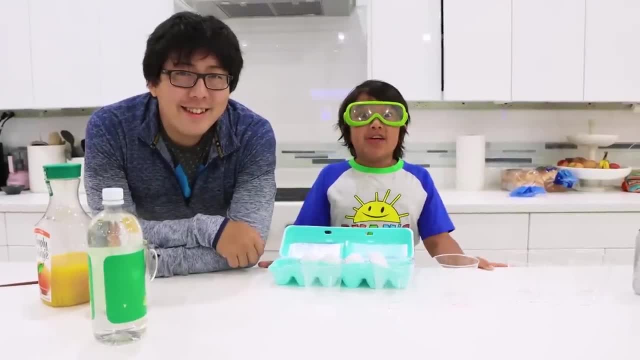 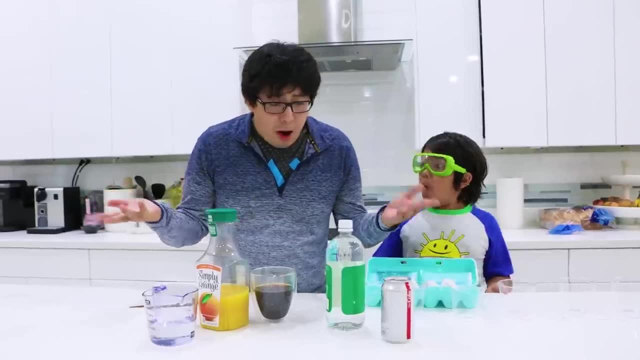 Bye. Who needs energy? Hey guys, Today we're going to do a science experiment and see what happens when we put these eggs in liquids. We prepared so many different kinds of liquid. You've got Diet Coke, vinegar, Coffee. 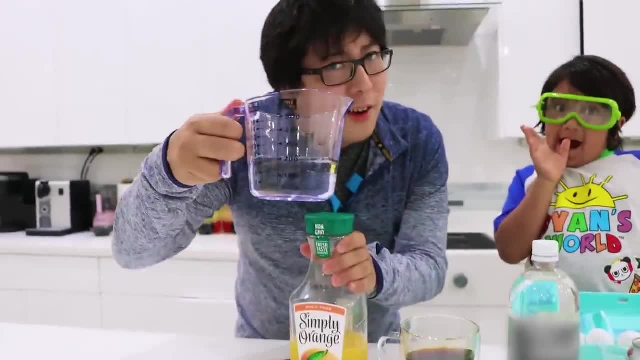 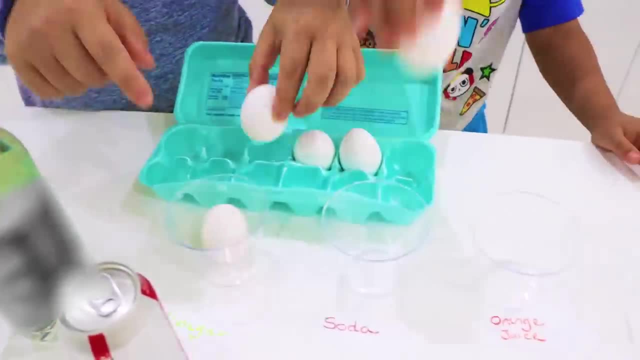 Coffee, Juice, Orange juice and water. Baja Eggs are made up of a similar material as your teeth. We're going to put the eggs in each cup with the different liquids so we can test out and see what happens to the. 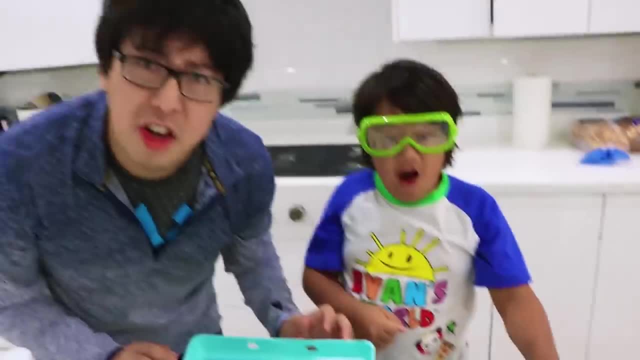 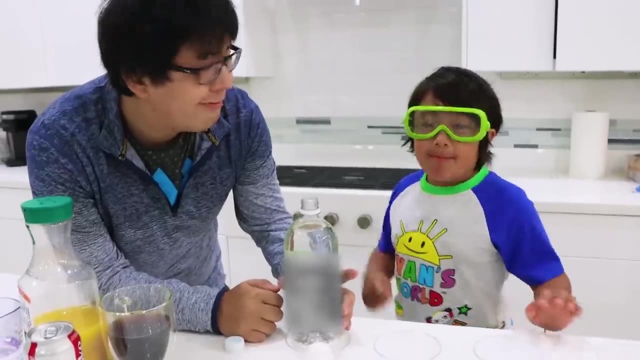 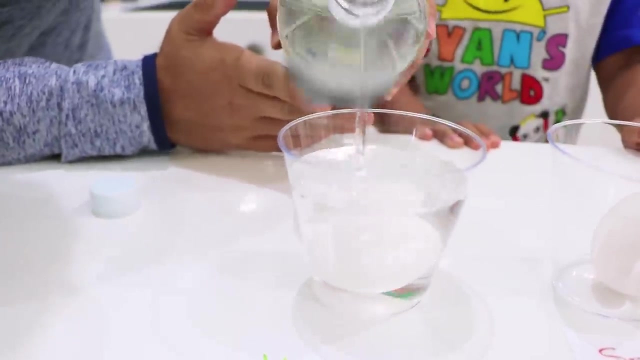 So we can test out and see what happens to the Hey guys, to the teeth, if you don't brush it. this one says vinegar, we're gonna pour vinegar. all right, here we go. daddy's gonna pour vinegar, let's see. oh yeah, it does smell like a vinegar. all right, perfect. 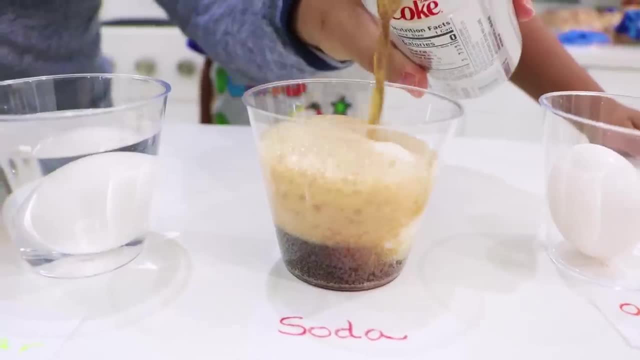 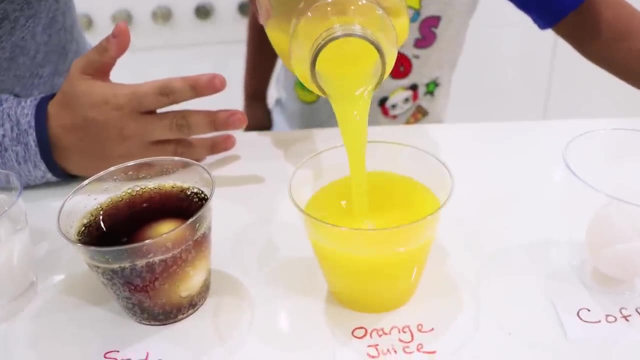 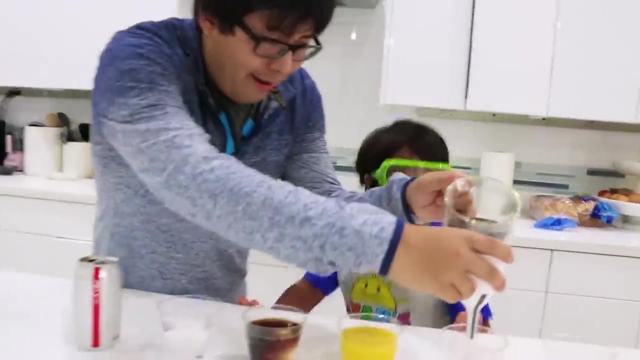 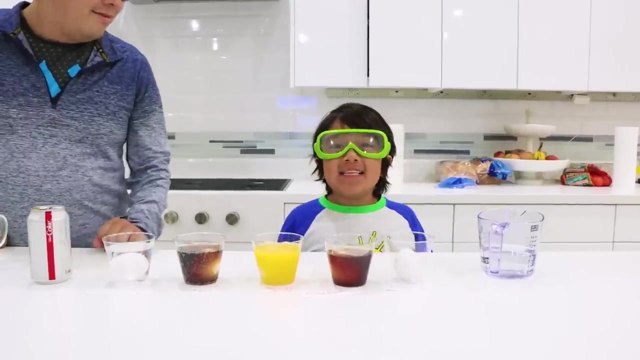 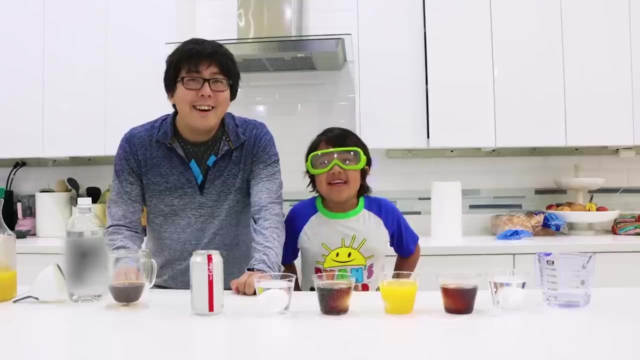 next is coke: pour this into. next is orange juice- what's smelling. and the next one is coffee. next one is coffee. all right, here we go. all right. last is water out of the way and go. good job now. we're gonna wait one day. see you soon. 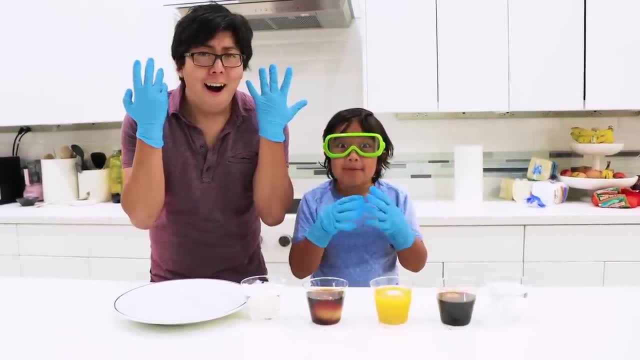 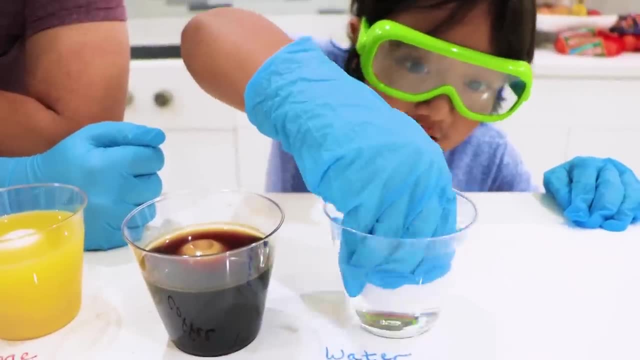 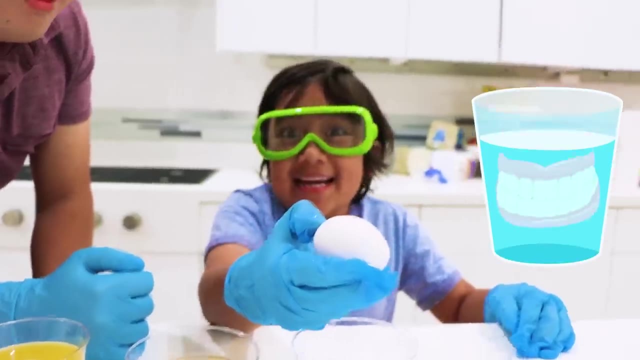 it's been one day now, and now we're gonna check what happened to the eggs. now we're gonna start out with water, carefully touch it. oh, it's the same, so the exact same. yeah, so if you put your teeth in a wall in water for a day, 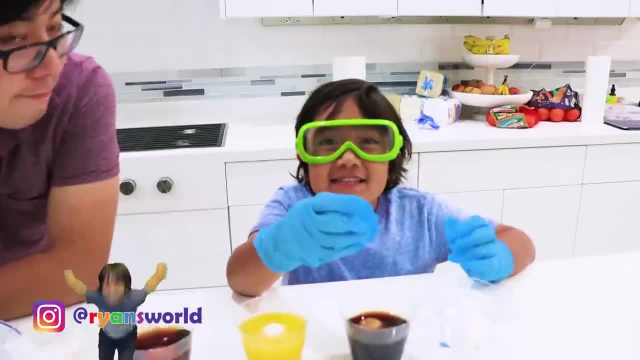 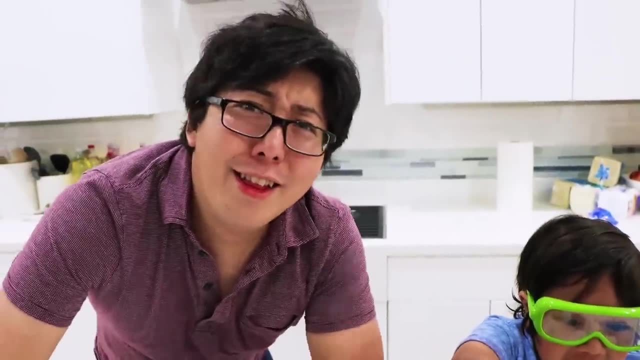 nothing happens, okay, so water is good for you. next, let's look at the egg in coffee. oh yeah, i drink coffee all the time. so this is my teeth blah, I thought i'll brush my teeth. look at this. what happened to the egg, ryan? it's brown. it changed the color. look at it. so what happened if you don't brush? 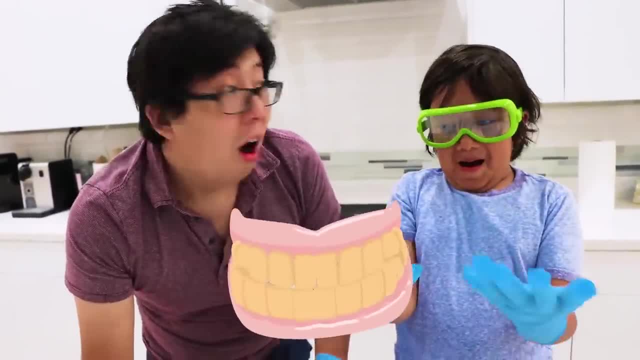 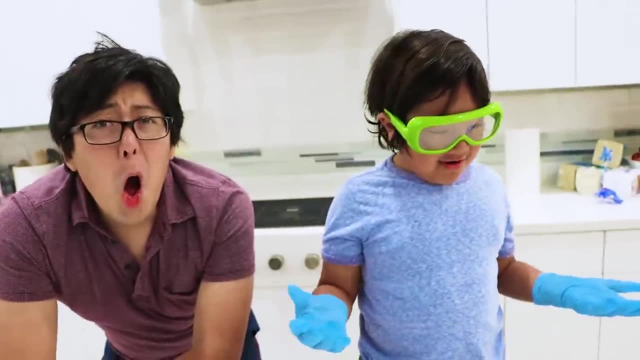 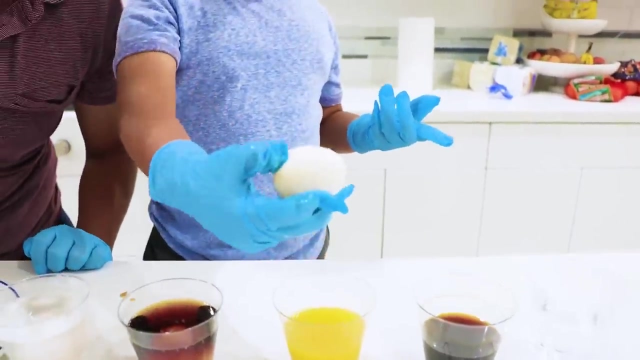 your teeth after you drink coffee. it's kind of brown, i know no more white. this is what a normal egg looks like, and this is what an egg in coffee looks like. Now let's try orange juice. it can't be orange, right color. let me see what. oh, you see the bubbles that are on it. yeah, but 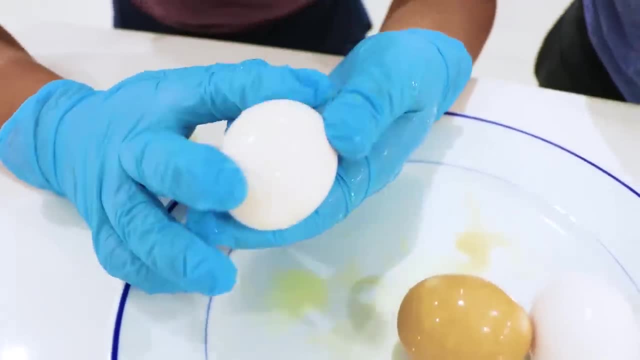 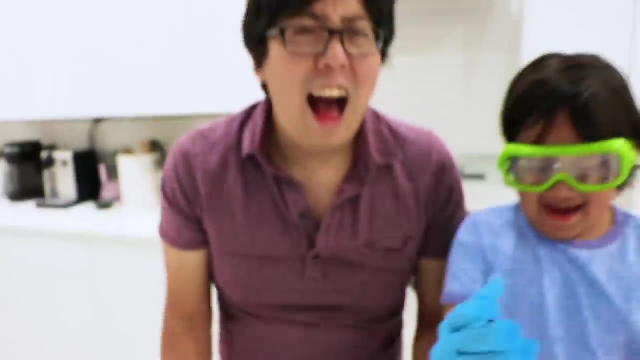 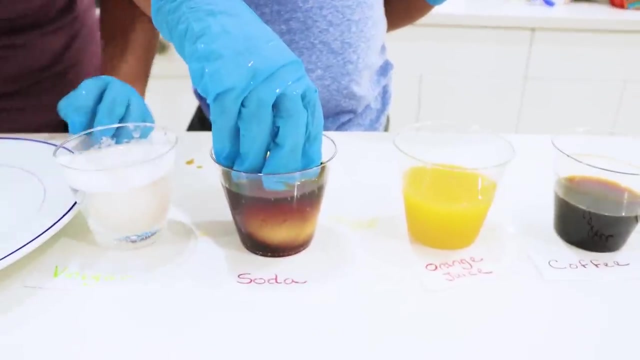 besides that, it's same right. don't forget, there's sugar on there too, so if you leave it for a while it might attract bacteria and germs. stop touching that. now we're gonna try soda or coke. oh yeah, we hear all the story about soda. let's see what happens. soda also have lots and lots of sugar. 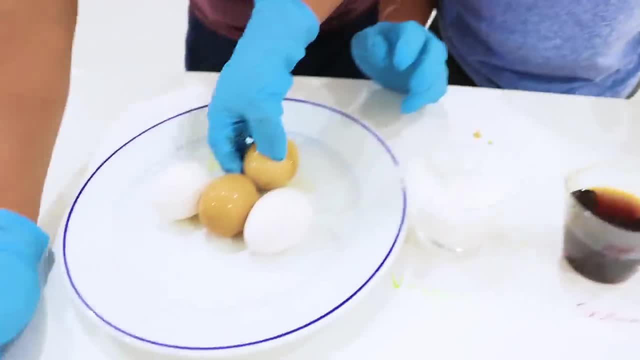 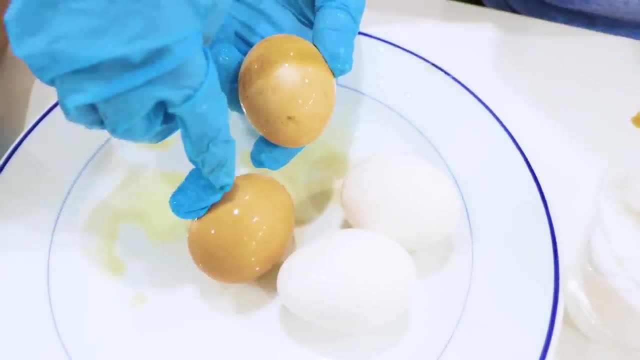 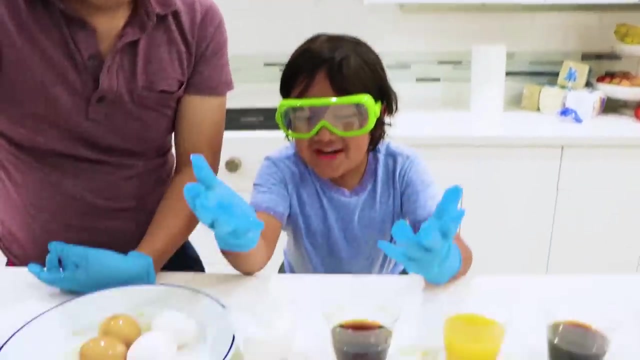 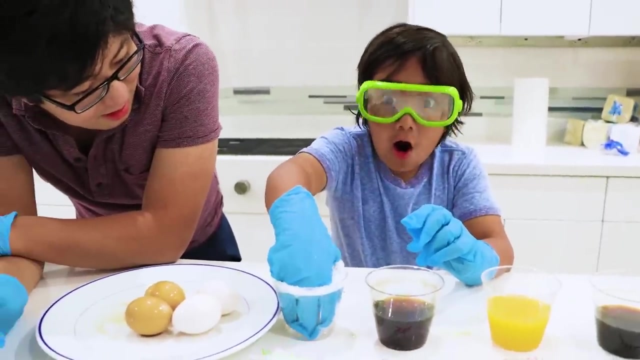 no, it also stains the egg. wow, wait. so this is like a super good version. this is a second best version. this is a worse, the worst version. no more white teeth. right, this is the most exciting one. vinegar- all right, let's see, take it out, Ryan, take it away. all right, you gotta be gentle, oh. 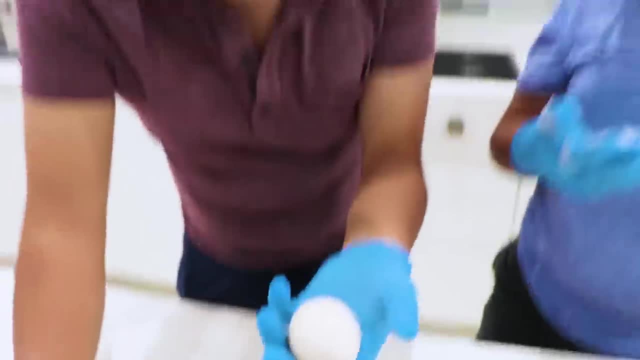 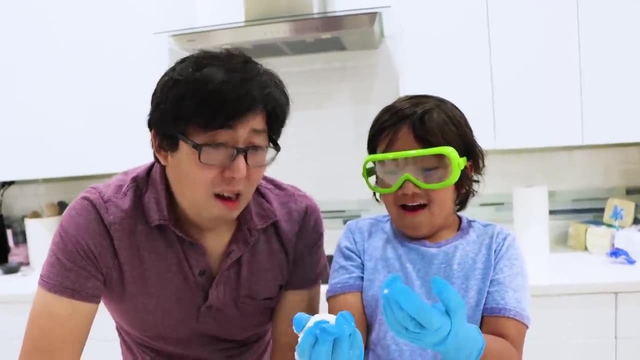 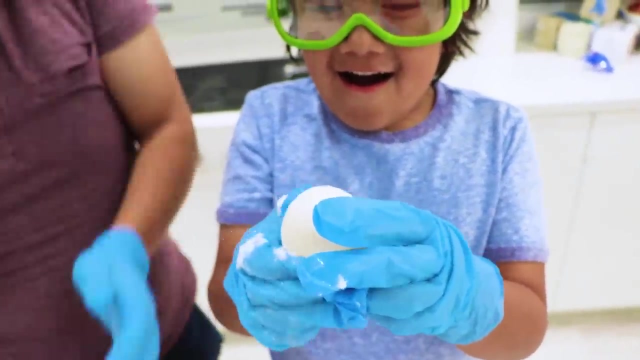 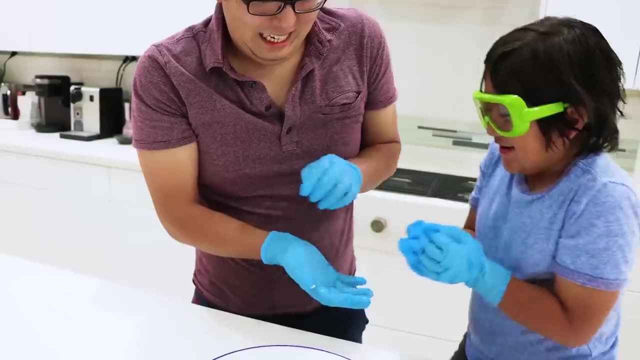 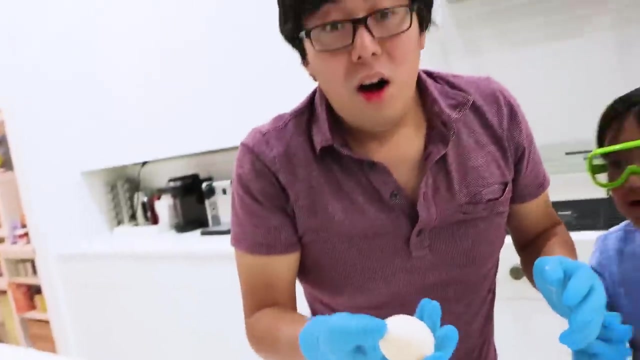 feel it. feel it. vinegar is very acidic, so it actually dissolves the shell. the shell is gone, Ryan, I knew it. it's all you left. it's gonna explode. it's like a bouncy egg you dare to bounce. yeah, it's actually pretty bouncy, you guys, you can bounce it. it's actually pretty bouncy, you guys, you can bounce it. 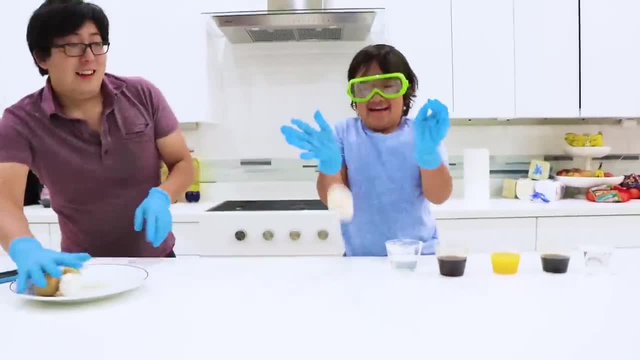 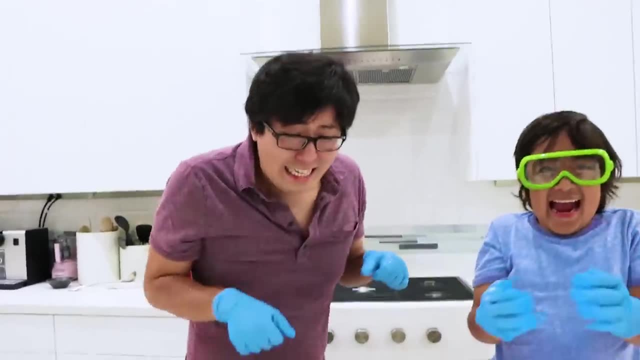 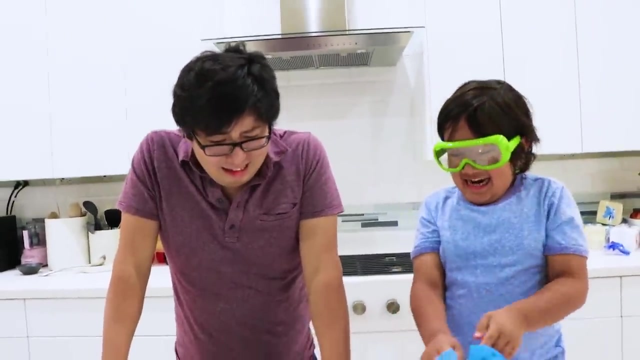 it's: oh yeah, maybe we should have kept it in there a little bit longer. it'll take a day, so maybe you need two days. so ride it the shell. so I'm probably bouncing a little bit too much, but if you leave it in for two days, it's actually more. 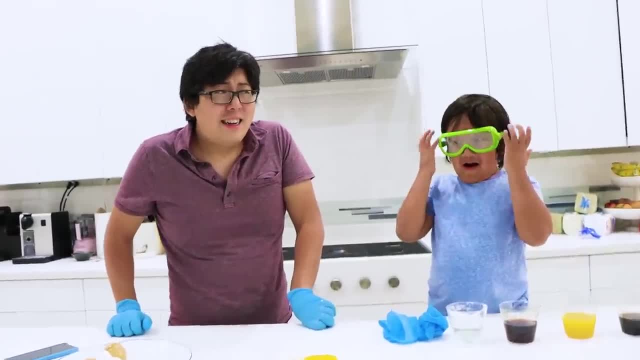 bouncy. Wow. so now you know what happens to vinegar. what does it do? it just all. I just see I knew it partes it there. so it's this Bounce's and you get a burnt shell right. so I just need to take it out in there. D problems, Frank. 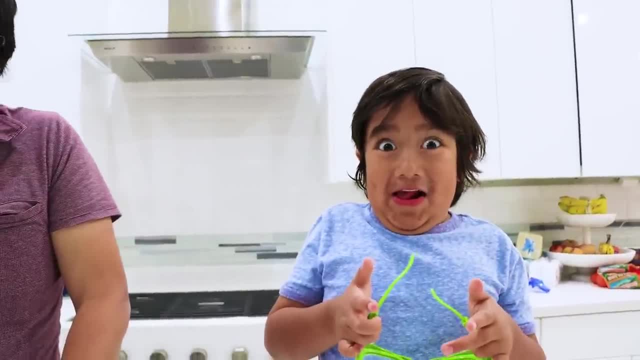 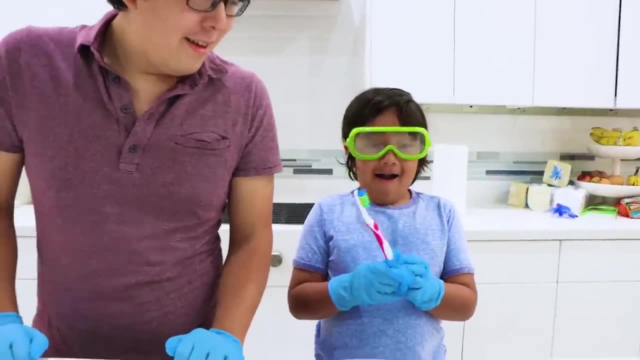 It dissolves, It dissolves. All right, guys, clean up. time, We're back. we cleaned up. we got new gloves, right. And then Ryan learned not to touch raw eggs, right? Yeah, Ryan also go wash his hand already. 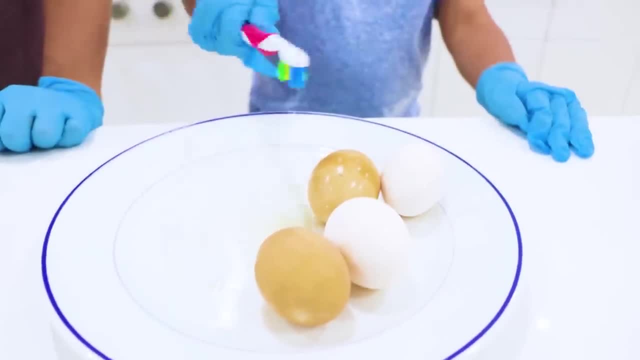 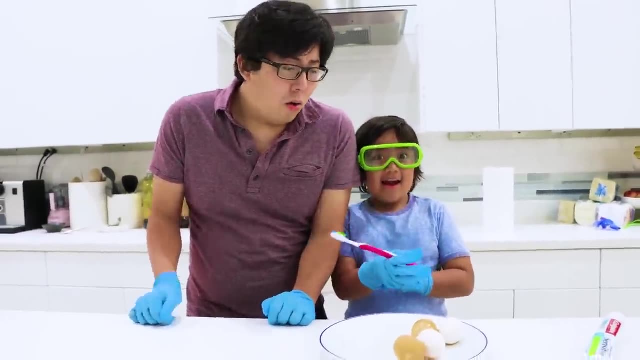 So now do you see how the eggs that was in coffee and soda was brown? We're gonna test it out to brush it, yeah, to see if it has any effects. okay, Yeah, Yeah, make sure you put the toothpaste on. 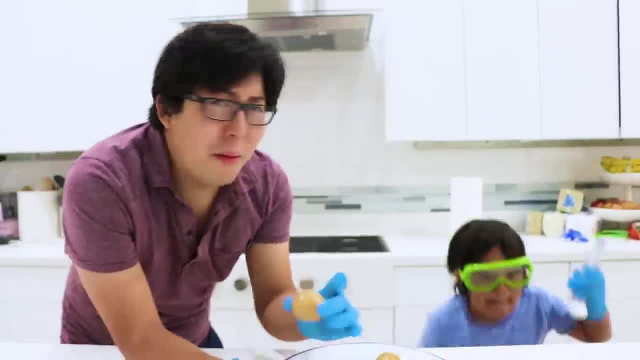 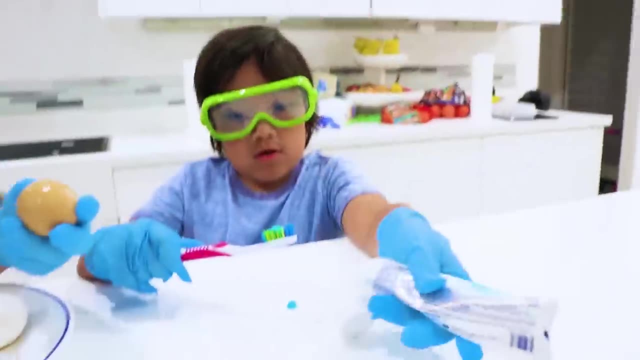 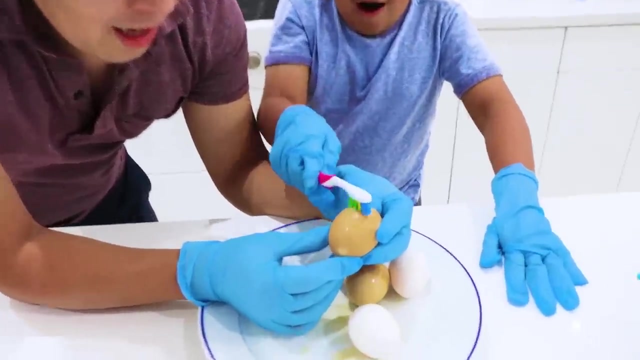 Oh, be careful, Teamwork. Oh, Cannot be my toothbrush. Okay, Ryan's holding gloves, so maybe that's like a little bit hard. Yeah, that's good, Here we go, Three, two, one Brushy, brushy, brushy. 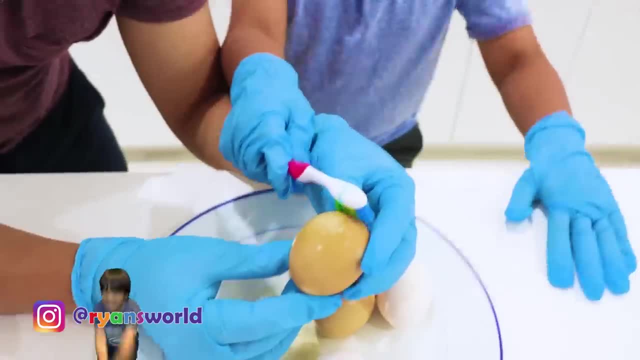 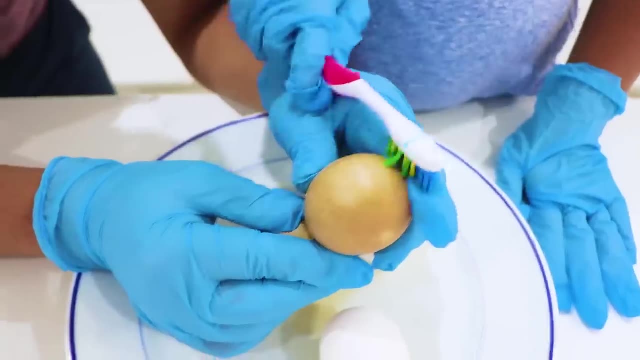 Brushy, brushy, brushy. 10 hours later, No, We're seeing if it works. Whoa, whoa, I can tell already Does brushing help make your teeth whiter. So Oh yeah, I see it. 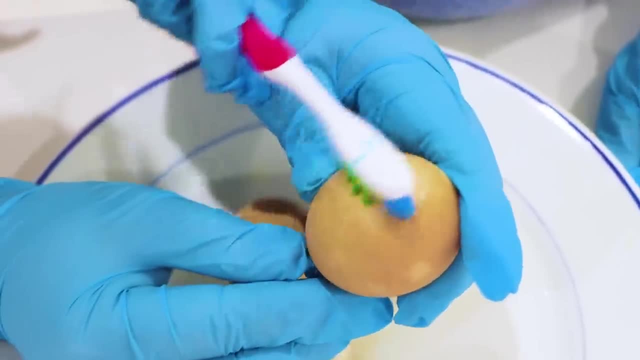 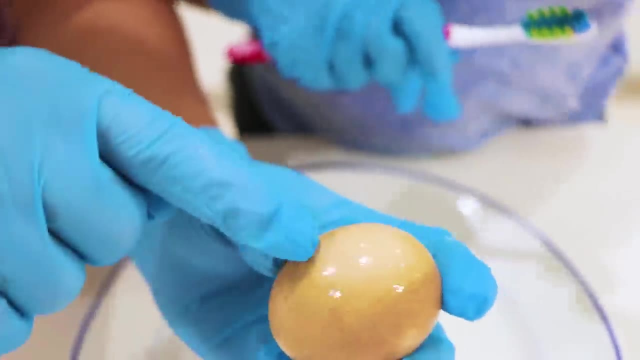 Look, Yeah, Yeah, Ryan, Look, it's already getting less brown on the spot that you're brushing. You guys see, Oh, look at it, Oh, it's already the difference. This is the regular spot and this is where we brushed it. 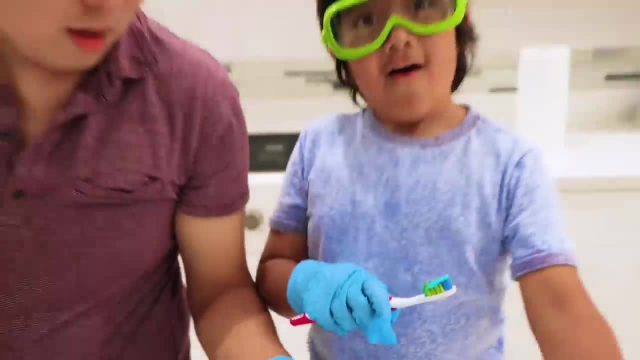 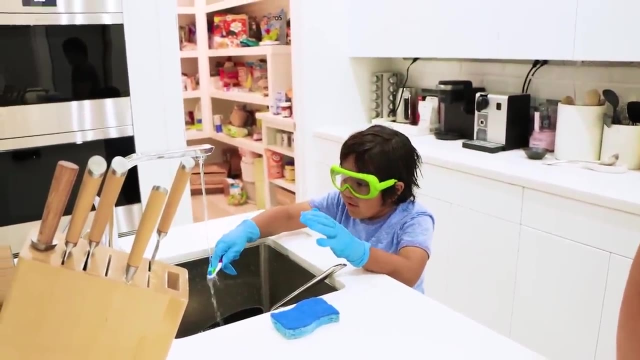 Oh yeah, Look at how, yeah, Wow, the importance of brushing your teeth, right? Uh-huh, Ryan's brushing the toothbrush. Oh, Oh Okay, Ryan's brushing more to see. Whoa, Oh yeah, I can tell the difference. 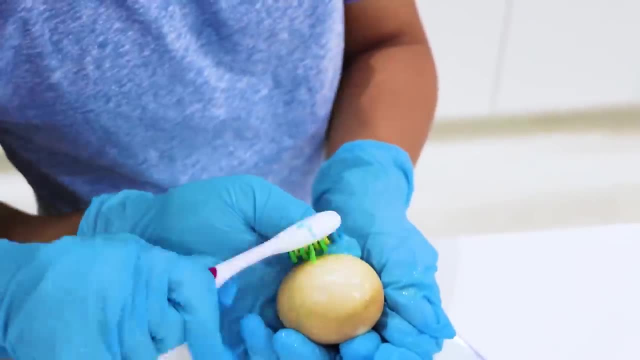 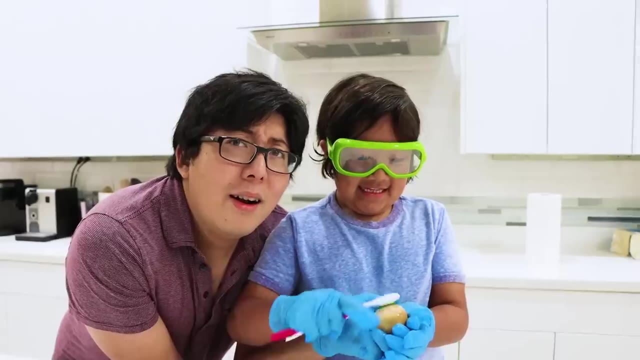 Good job, Ryan. Whoa See the difference? Yeah, I can tell Nice Big difference. So what did you learn, Ryan? That brushing your teeth helps a lot. Yeah, it does. And how many times a day you're supposed? 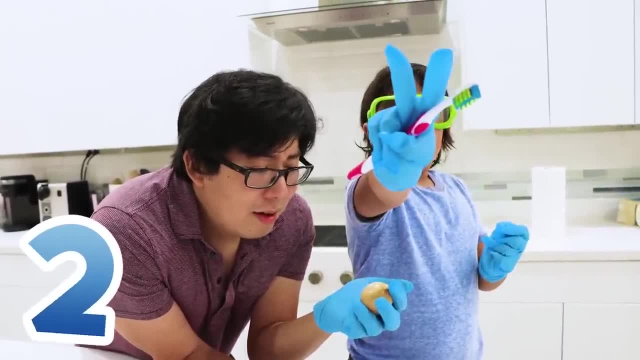 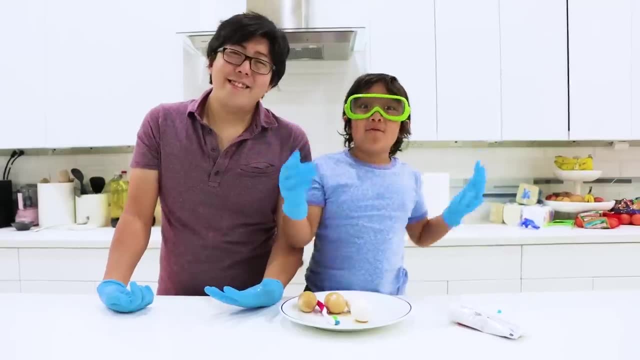 to brush your teeth at least Two, Two times a day. Good, For how long, Do you know? Two minutes, Two minutes- Yeah, Easy to remember. Thank you for watching. I hope you like this science experiment. Bye. 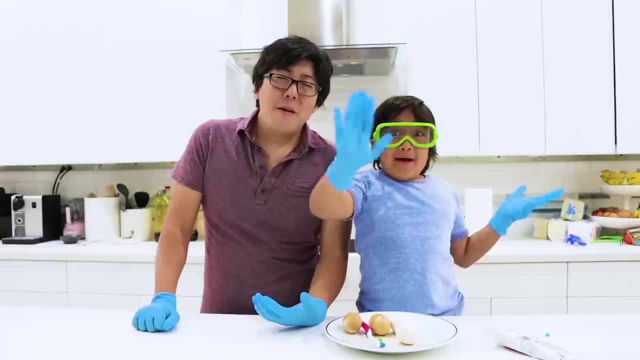 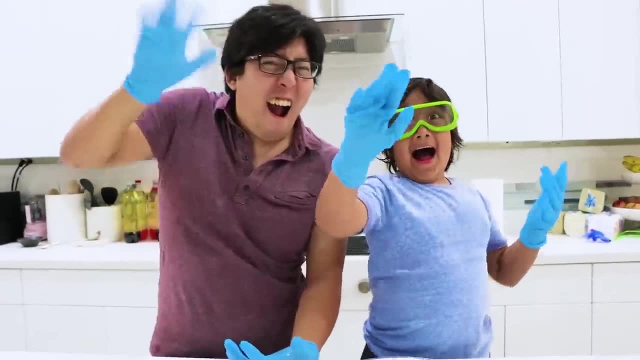 Remember always stay happy and rise up. Bye, Bye, guys, And see if you guys can put eggs in different types of liquids to see the difference. Aw, Oh, where's Ryan?